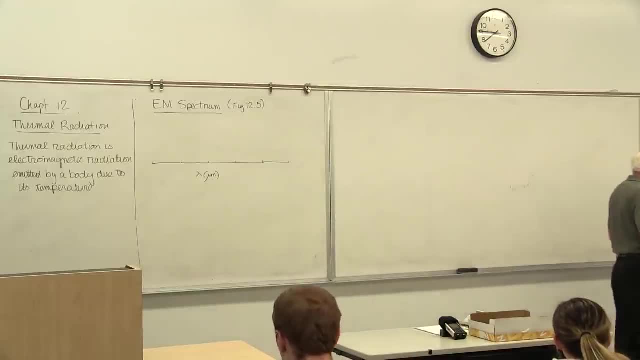 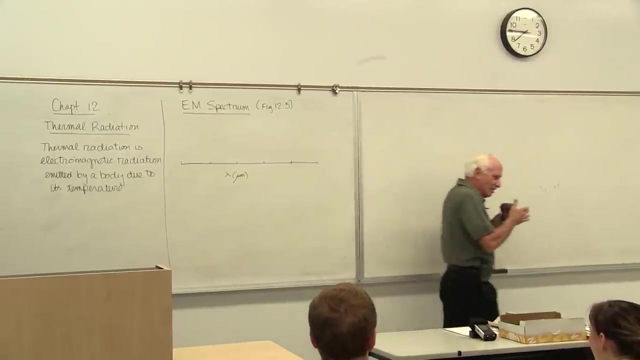 Sometimes it's not And it can be neglected. We'll talk about that later on when we get to certain problems. Official definition: Thermal radiation is electromagnetic radiation emitted by a body due to its temperature. You can also look at it from the point of view of photons carrying energy. 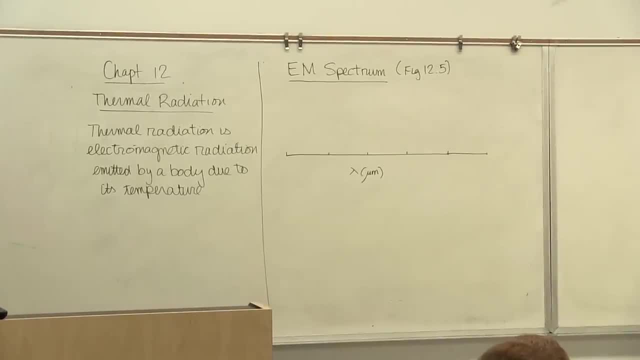 There's two approaches We're going to focus, and our book focuses on talking about thermal radiation as electromagnetic radiation. The key thing is it's due to its temperature. Okay, Figure 12-5 or 3.. Let me make sure which one it is. 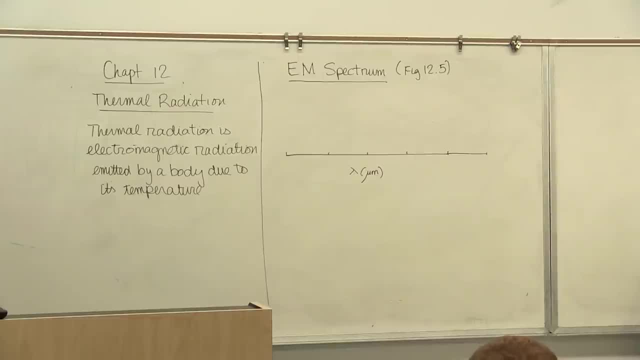 I think it's 3, maybe Yeah, it's 3.. Figure 12-3.. The EM spectrum We plot on the x-axis the wavelength. Wavelength is lambda. It's in units of micron, 1 times 10 to the minus 6 meters. 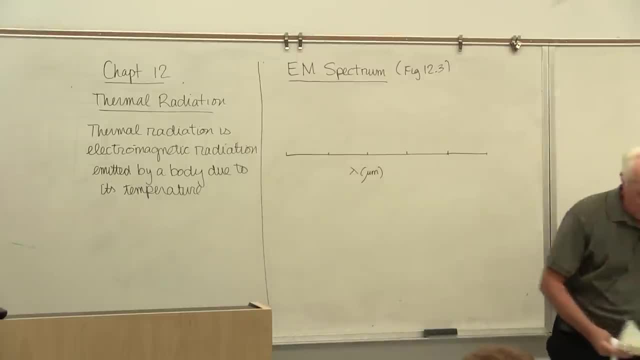 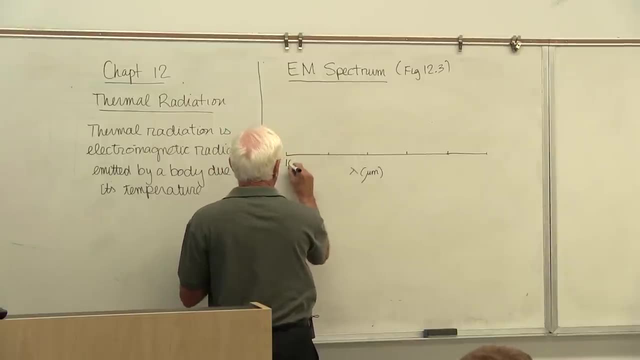 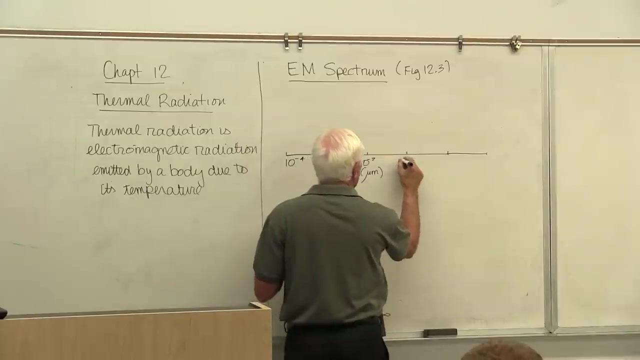 And we're going to show first of all, at very short wavelengths, x-rays out from this is, by the way, 10 to the fourth: Minus 4., Minus 3.. Minus 2., Minus 1.. 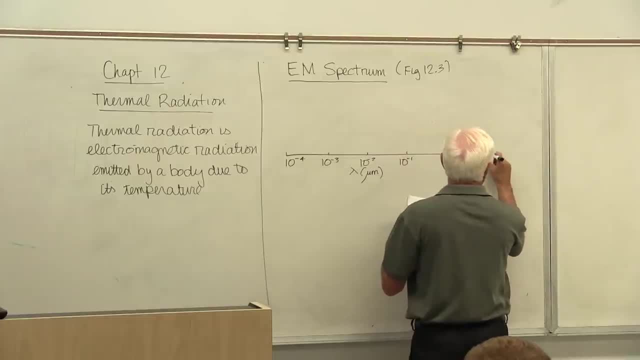 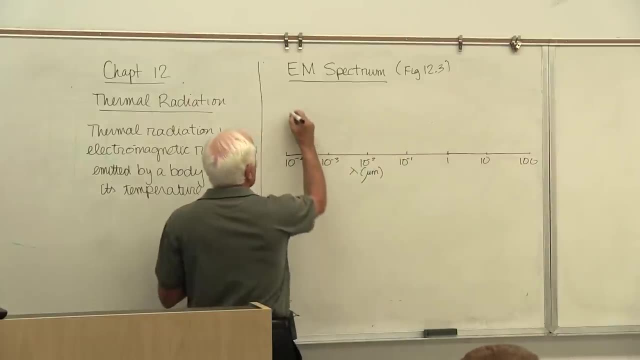 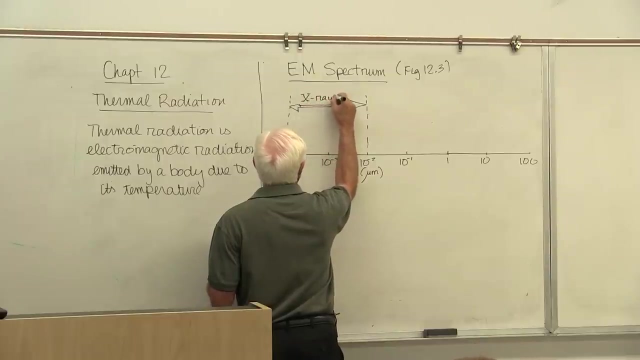 1. 10. 100.. Okay, so we said we'll start here at 10 to the minus 4.. Let's just show x-rays on this side: 10 to the minus 2.. X-rays: Short wavelength. 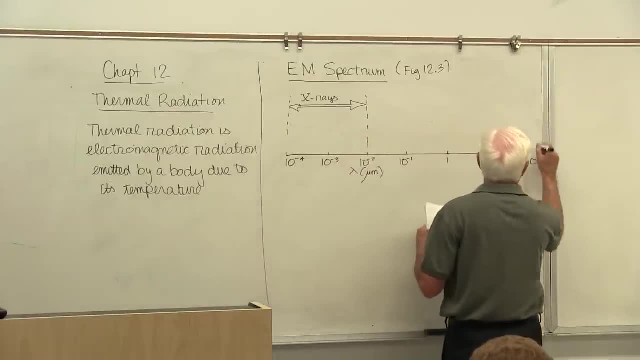 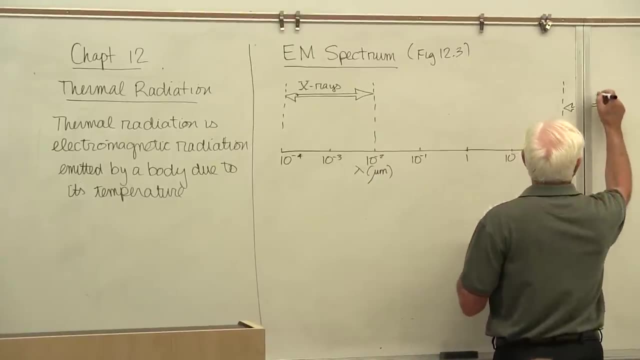 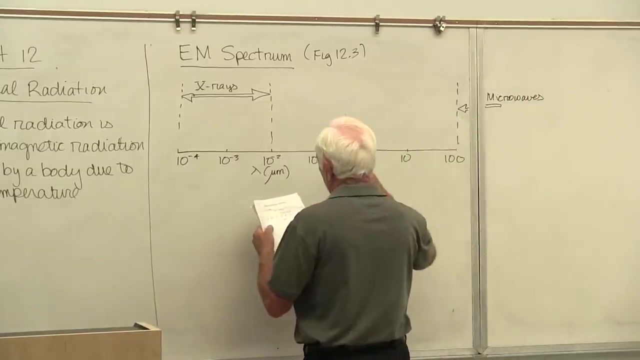 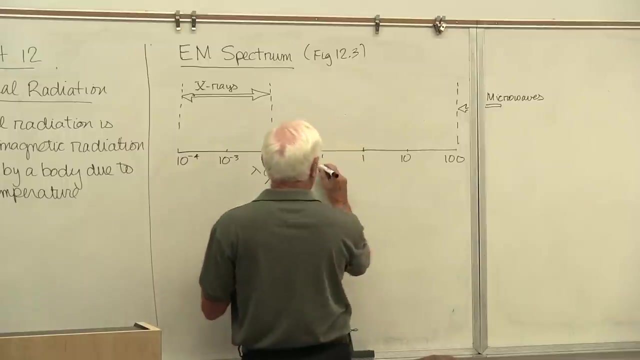 We go out above 10, above 100.. And on out, these are microwaves. We go from 10 to the minus 2 to 0.4.. There's 1,, there's 0.1, 0.4.. 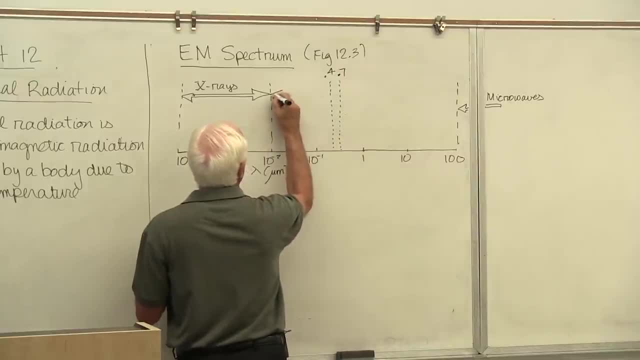 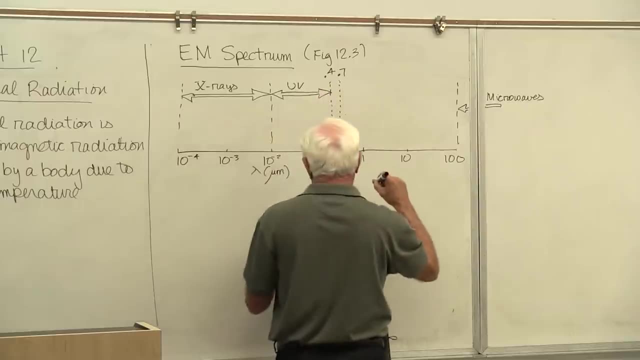 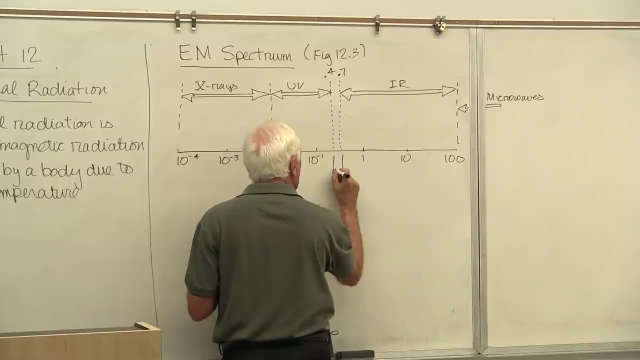 0.7.. So we go from 0.01 to 0.4.. UV 0.7 out to 100.. Infrared: The region from here to here, visible 0.7.. 0.7.. 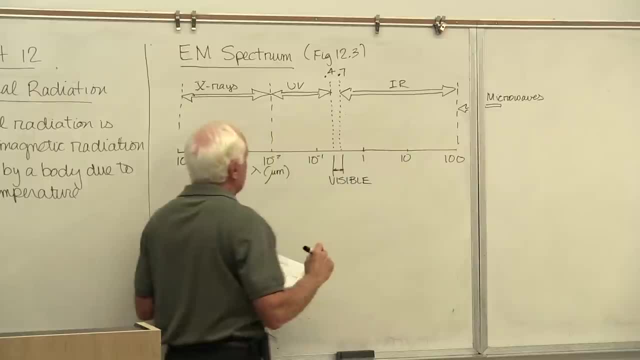 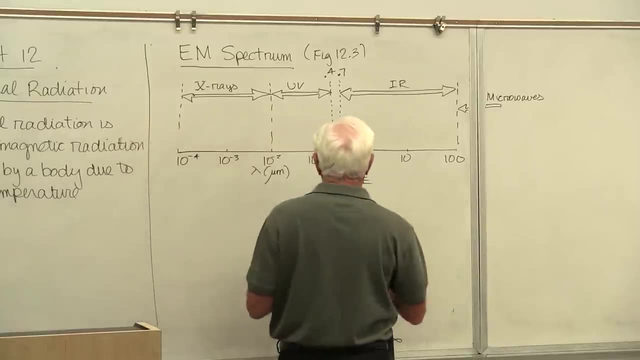 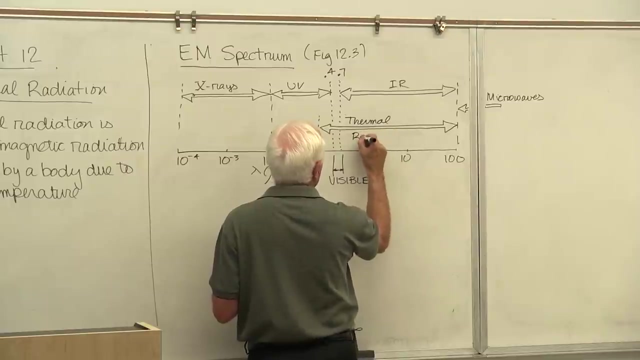 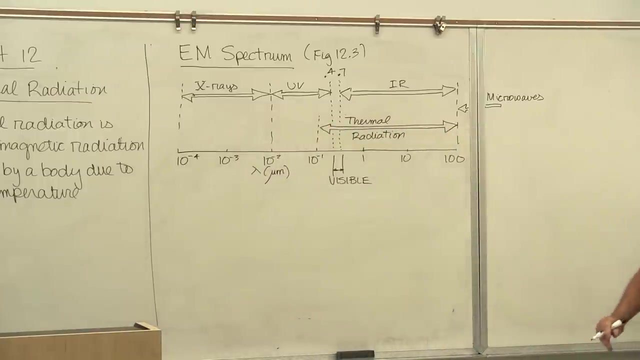 0.7. 0.7. 0.7. 0.7.. Now thermal radiation starts 10 to the minus 1 and goes out to 100.. And that's what we're talking about in these chapters. 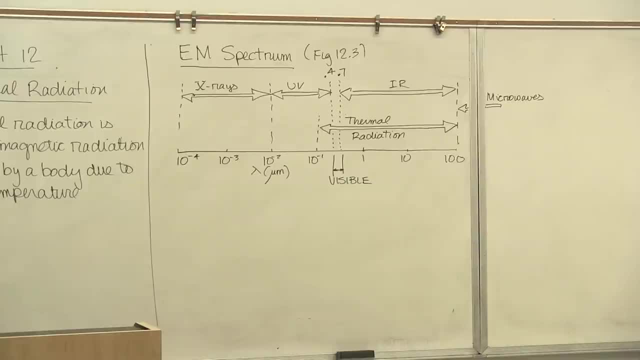 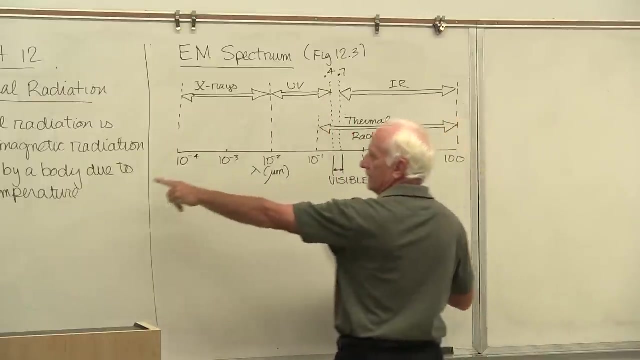 thermal radiation from 1 10th micron out to 100 microns. now we talked about a black body. I'm gonna erase microwaves. you just panel the board right here. of course, microwaves aren't caused by the body's temperature. x-rays aren't caused. 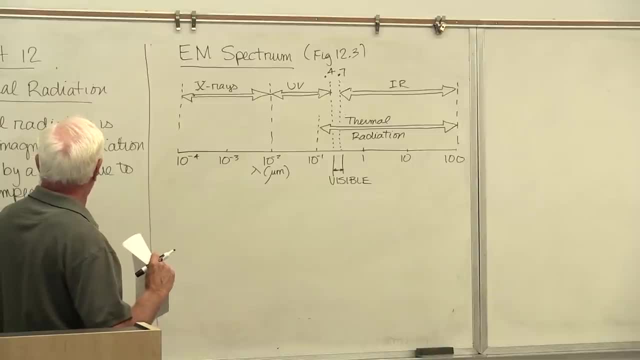 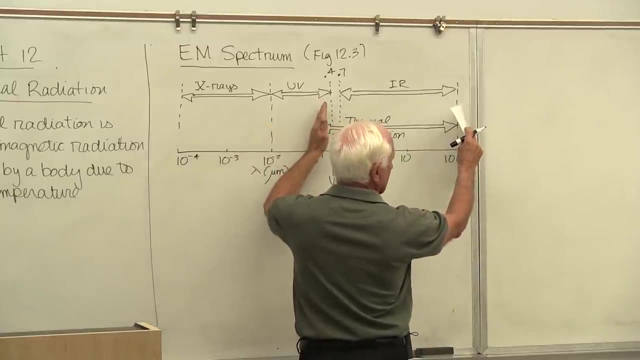 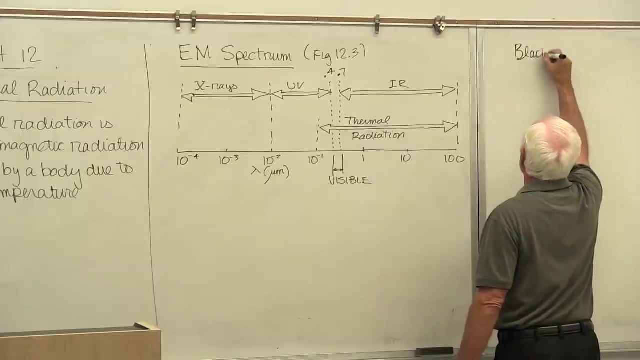 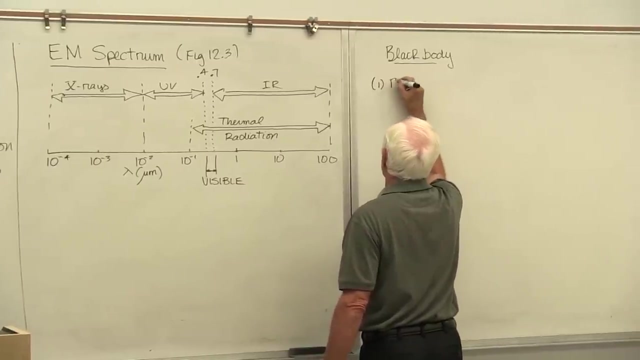 by the body's temperature. what's caused by the temperature of the body- thermal radiation. so from here to here is where we focus our attention for radiation. we're gonna go back now and talk about a black body, again from chapter one, black body. it's characterized by this: it's the best possible emitter. 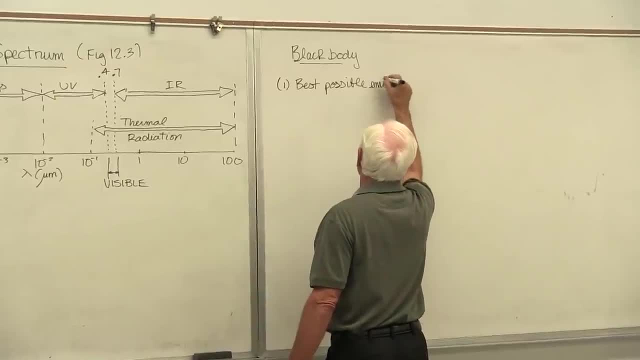 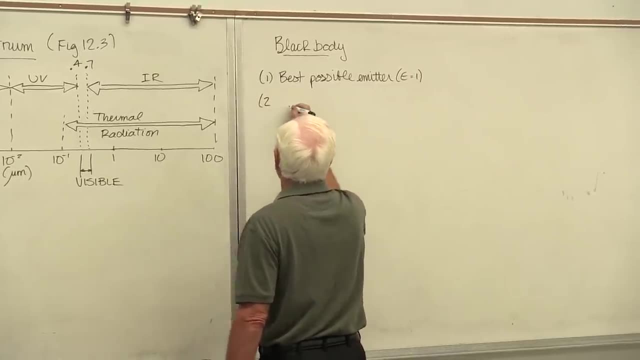 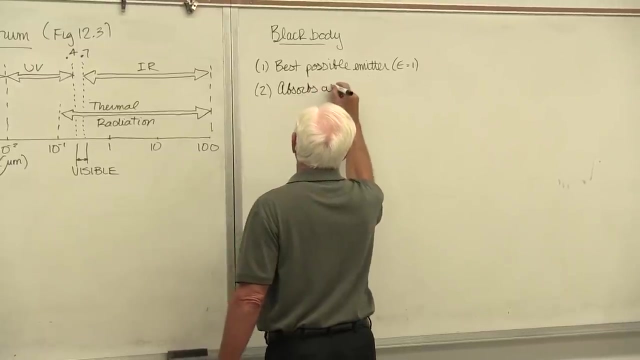 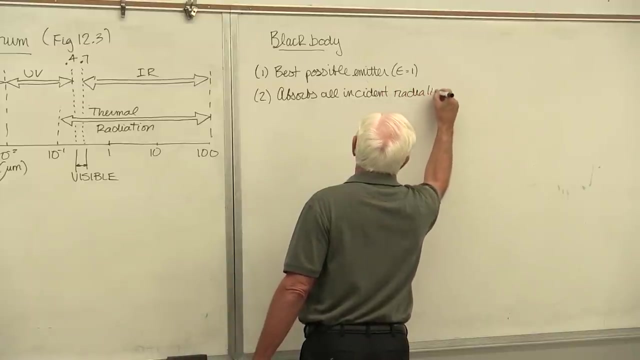 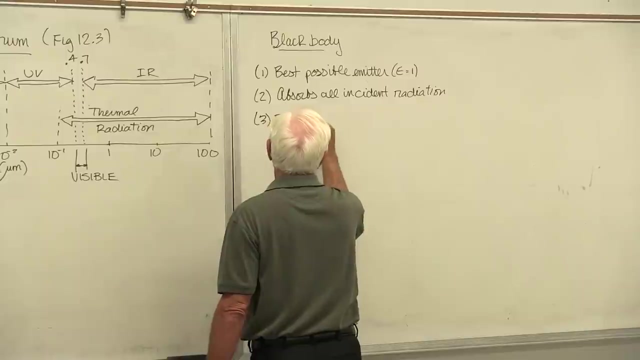 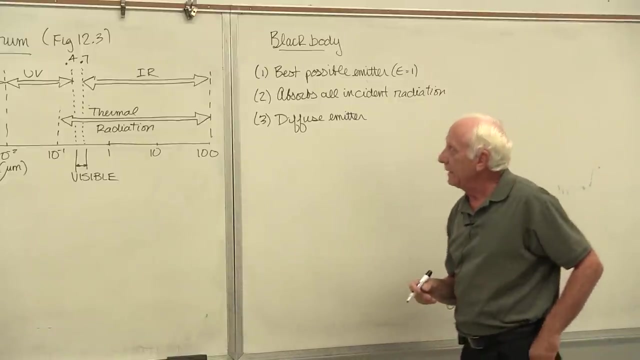 and we said in chapter one, that means the emissivity is one. it absorbs all incident radiation. and number three, it's a diffuse emitter. we'll talk about a dope. you see there, probably the start of Wednesday's class. so those are the three things that define a black body. it's, it's a model. 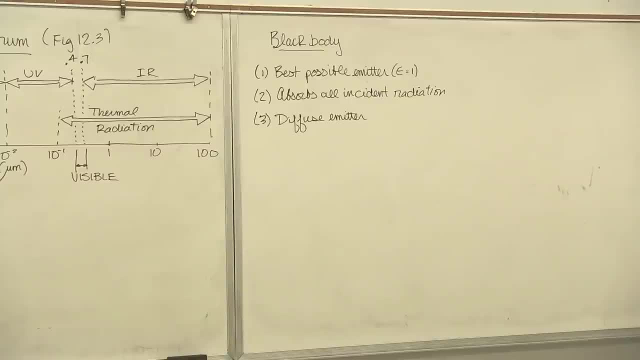 it's hard to build a black body. we talked about that before. you could buy a good flat black for butt cup cup paint at a hardware store, good flat black paint and painted color right here, kind of flat that might be an emissivity of 0.92 or 0.93.. 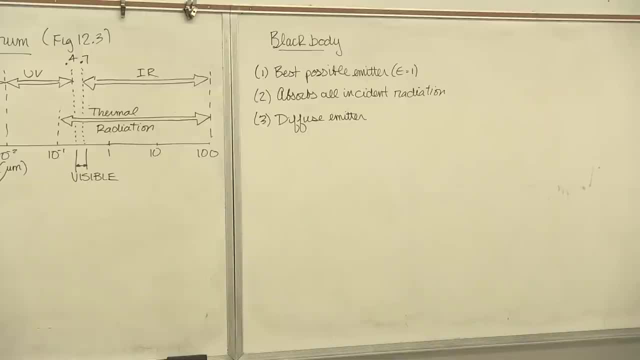 It is not 1.0, but it's up there in the 90s- 90%, So that paint might absorb 90% of the incident radiation. So it's a model. It doesn't happen too often. Nothing in this room really is a black body, obviously. 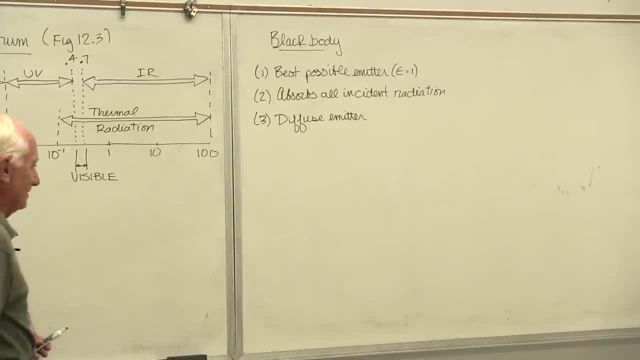 The walls are a gray-green color, The ceiling's white, The floor is tan And those all have emissivities, less than one. They're not black bodies. We'll talk more about that in about maybe two days. Okay, so for a black body. 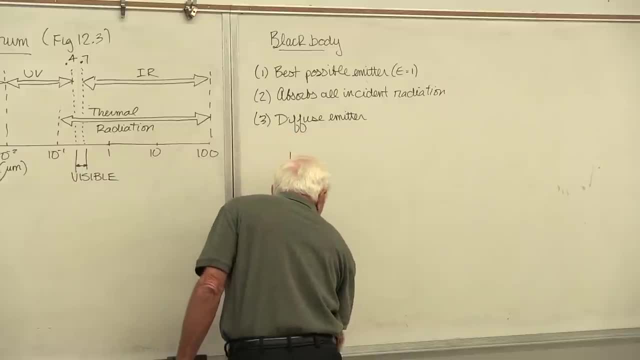 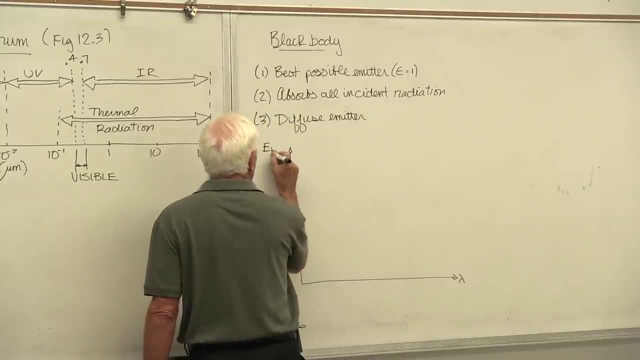 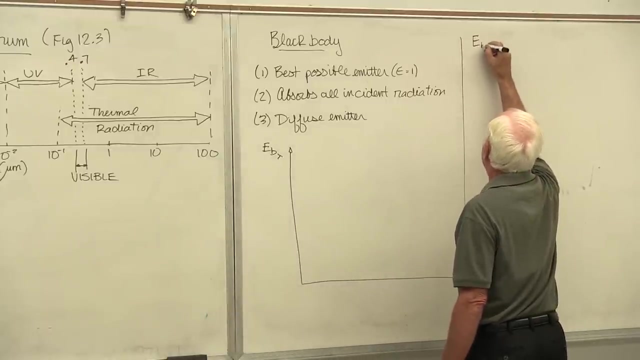 we're going to plot how it emits radiation. So on the x-axis we have lambda, On the y-axis we have something called E b lambda, And I'll just define those right here. E b lambda is the spectral black body, emissive power. 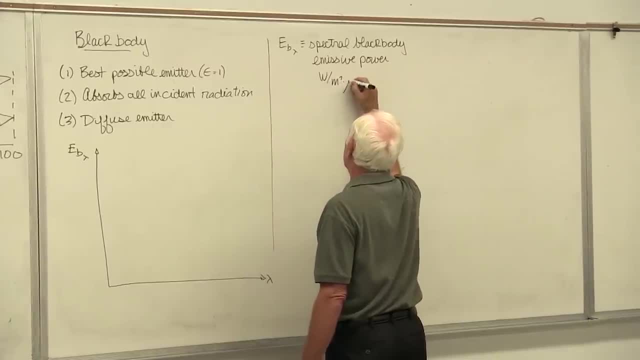 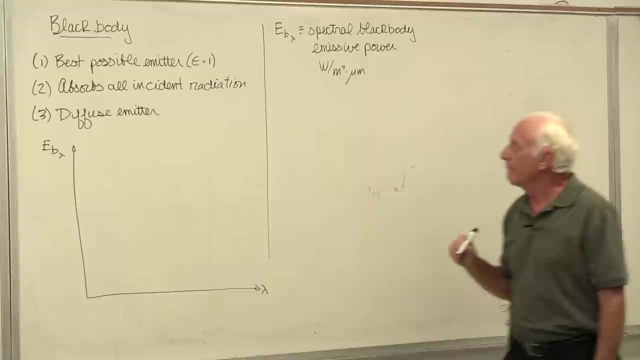 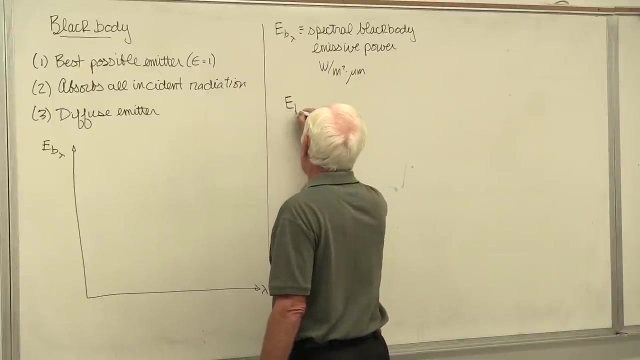 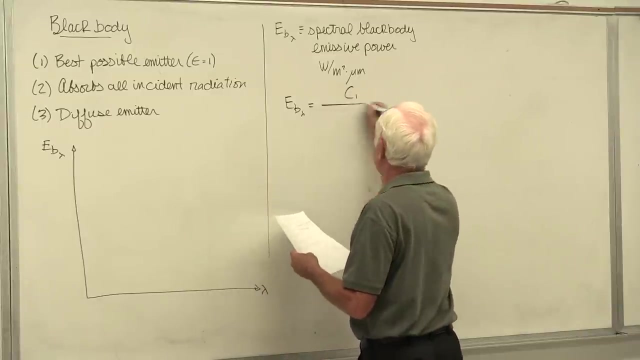 It's in watts per square meter. It's in watts per square meter per micron. Kind of strange, but it's in watts per square meter per micron Bar of black body. I'll write down the equation: A constant divided by C1 and C2 are constants. 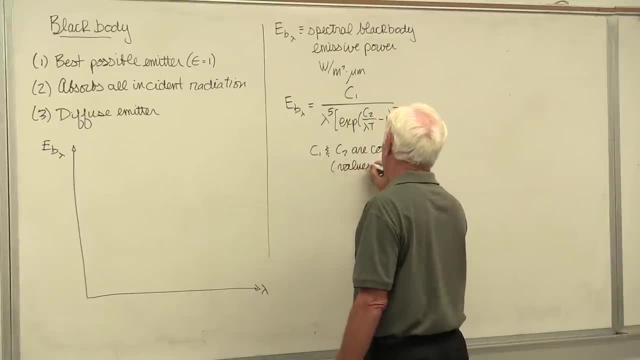 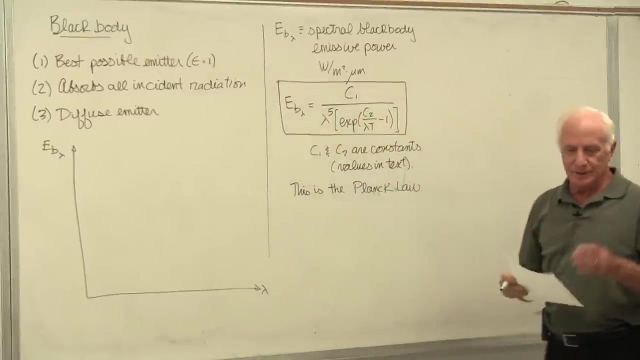 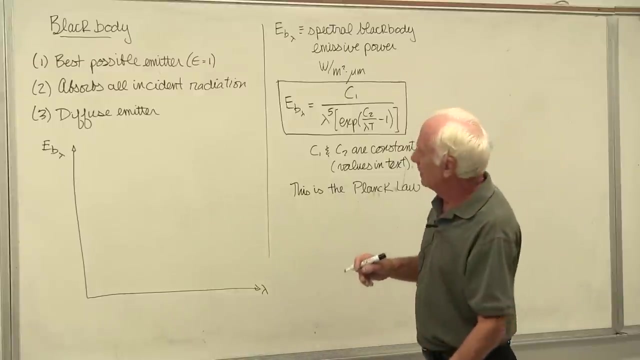 Values in the text And it's called Planck's Law. Planck's Law. It tells us how a black body emits radiation. Here's what the terms mean. 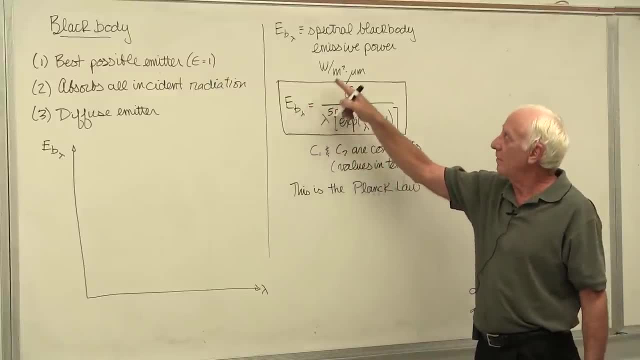 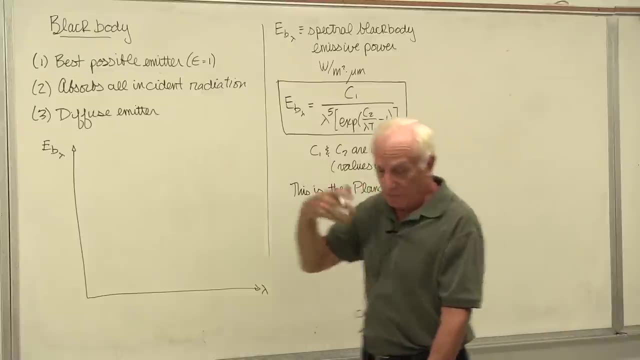 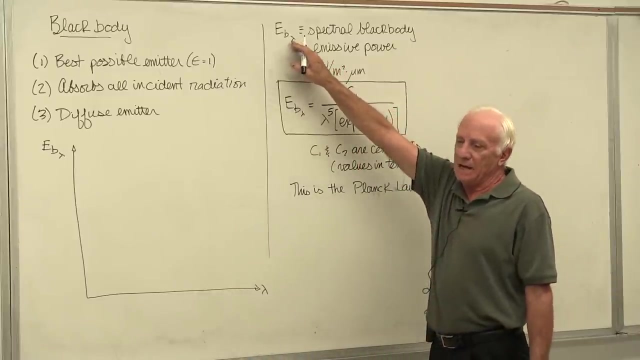 When you see a capital E, it stands for emissive power. E stands for emissive power. Emissive power means how much is getting out emitting. It's the emitting part. What's the B stand for? Subscript B- black body. 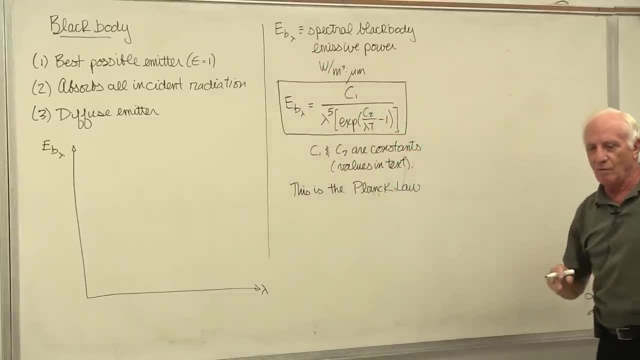 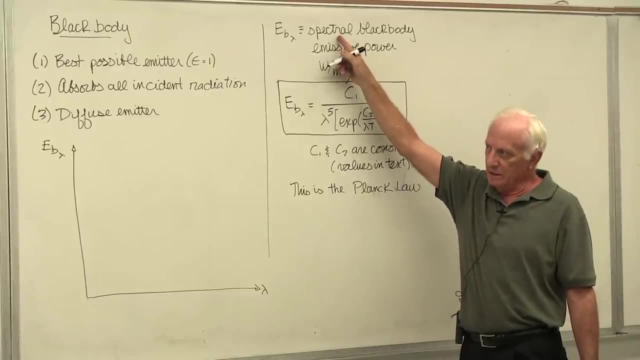 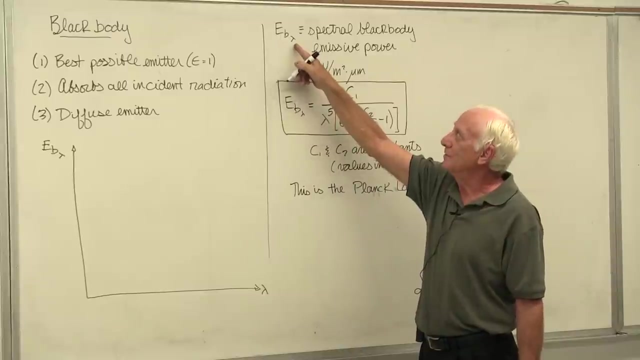 Subscript lambda: a function of wavelength. a function of wavelength. The word spectral means depends on wavelength. Spectral means depends on wavelength. So it's the point to them. The spectral black body, Emissive power. That's how you read it. 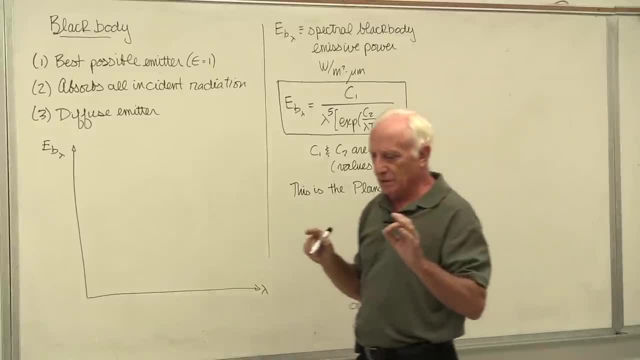 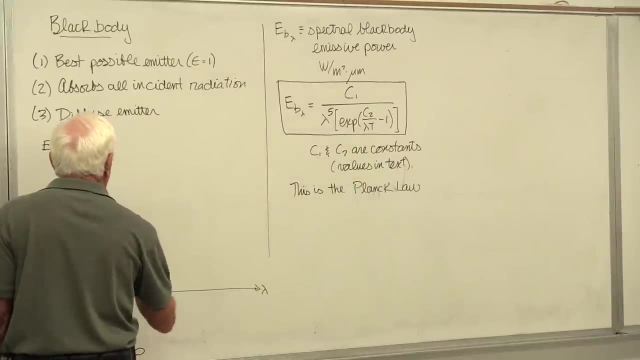 You can plot this guy now. Choose a temperature T, Hold the temperature constant and plot EB lambda versus lambda And you would get a family of curves that look something like this: As the temperature goes up, different curves. Let's just I'll put some numbers in. 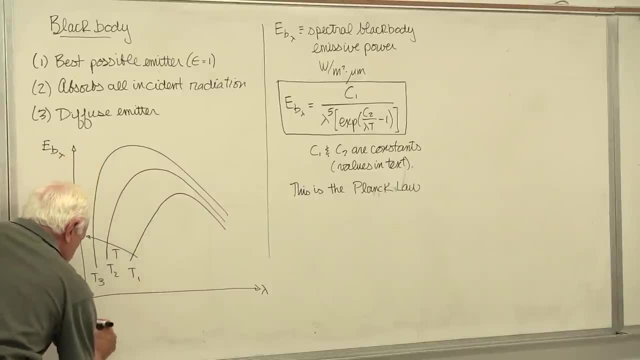 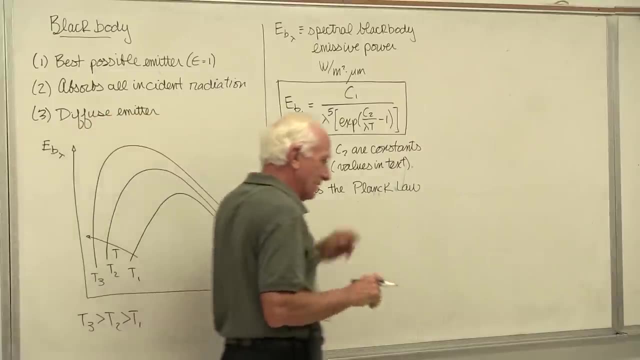 T1, T2, T3.. So for this particular picture, T3 is greater than T2, is greater than T1.. So if we're going to describe this graph now, you'd say, okay, as the temperature goes up. 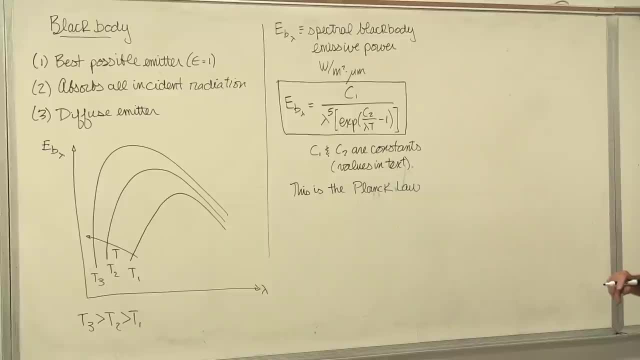 it looks like the body is emitting more energy. Well, that kind of makes common sense. That's to be expected. The hotter something gets, yeah, it's going to emit more energy. Thermal radiation. Conclusion number two: For any curve where temperature is a constant, it looks like it goes through a maximum. 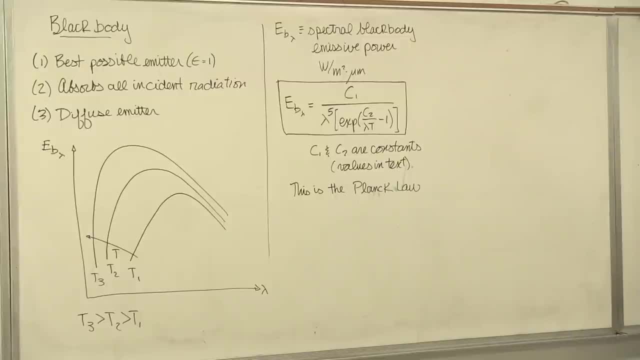 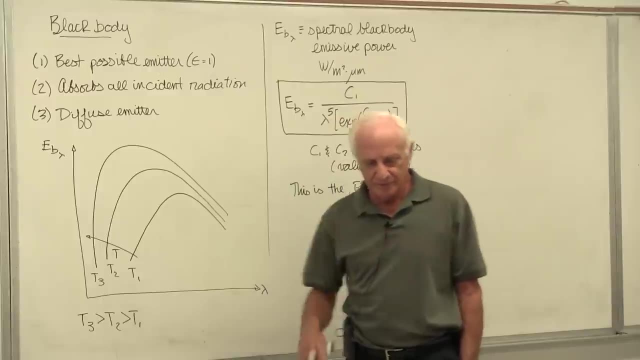 Yeah, you're right It does. For any given temperature, the curve goes through a maximum. That's two conclusions from the graph. See, a graph is really neat When you plot it. you couldn't tell it from a spreadsheet. 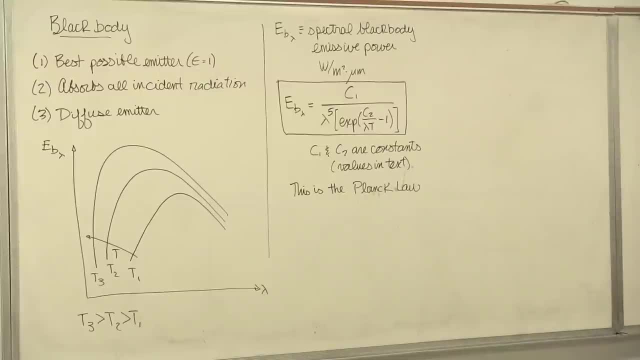 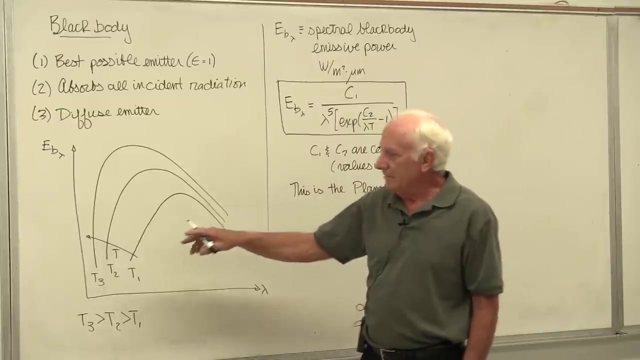 If you put those numbers on a spreadsheet, I guarantee you you have a real tough time figuring out what I'm saying right now. Okay, so as the temperature increases, the body emits more radiation. Okay, For any given temperature, we go through a peak value. 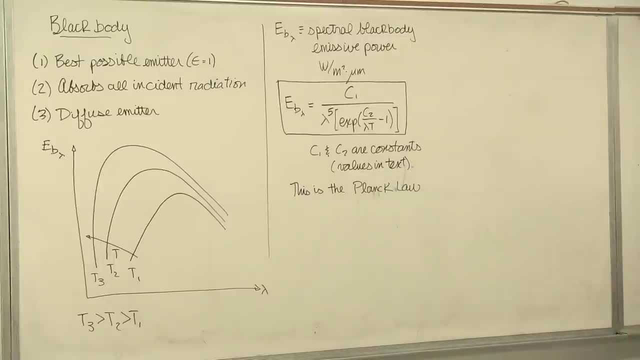 Here's a third conclusion. It looks to me like as the temperature gets lower, that peak value moves to the right at longer wavelengths. As the temperature goes down, the peak emissive power moves to the right. So longer wavelengths, longer wavelengths. 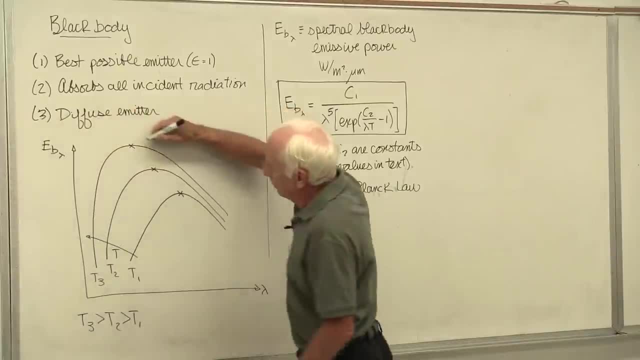 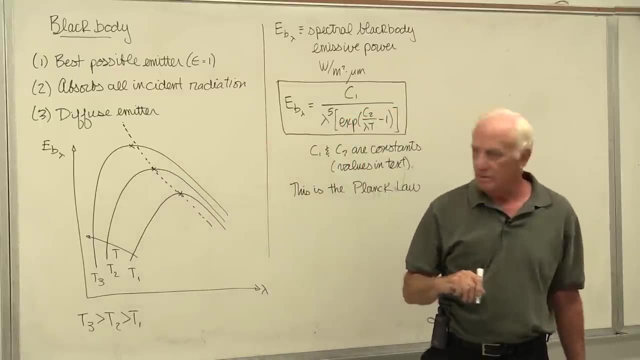 Yeah, they found that out. And then if I had drawn it right, if you plot this, it would look something like this: It's a curve. It's not a straight line, It's a curve. This is the locus of the peak emissive powers. that dashed line. 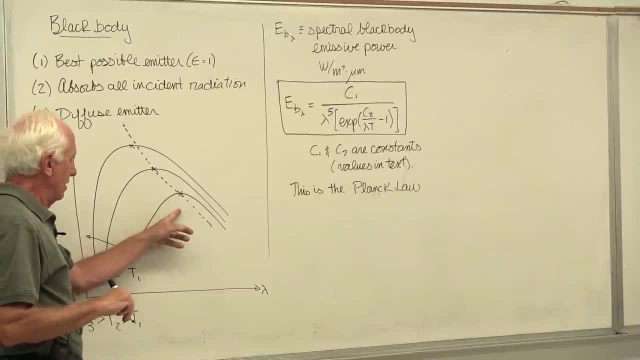 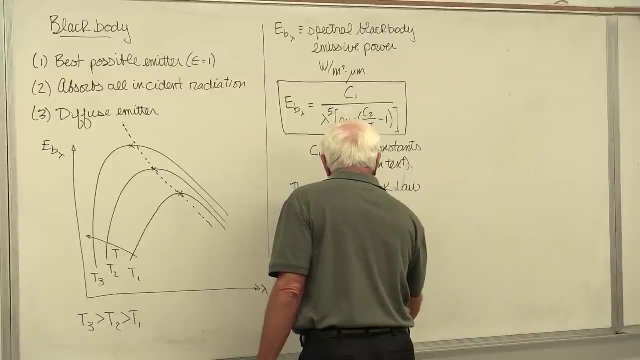 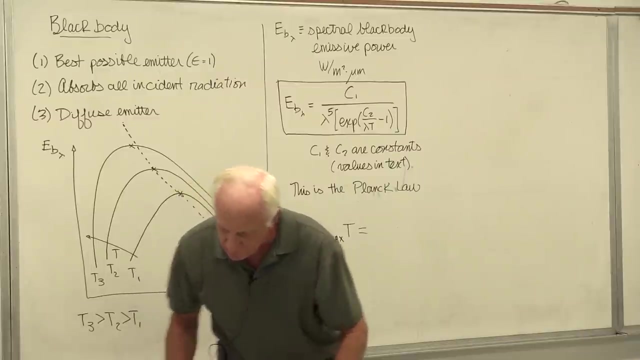 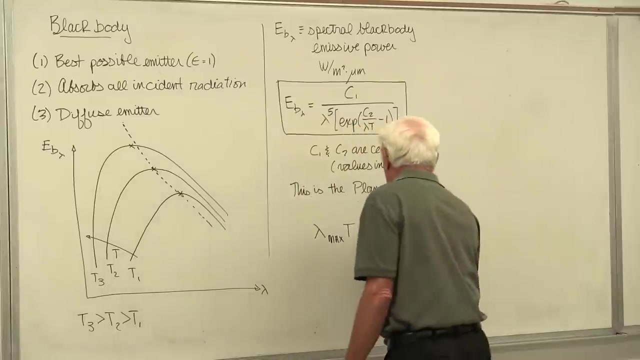 The locus of the peak emissive power. Well, they found out that lambda max t Equal a constant And that constant is 52, 15 point. Now let's do the SI version: 28,, 97.6.. And the constant is micron k. 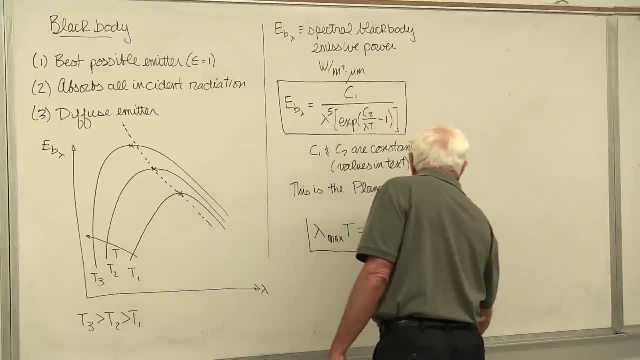 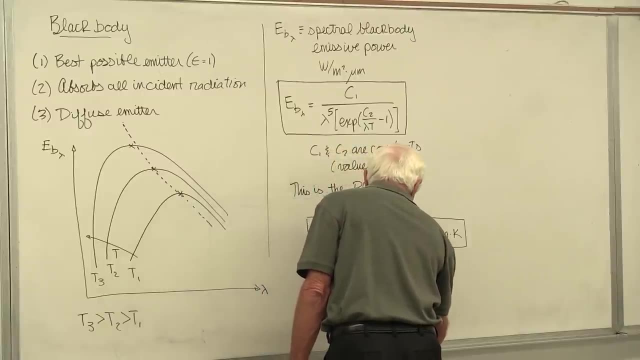 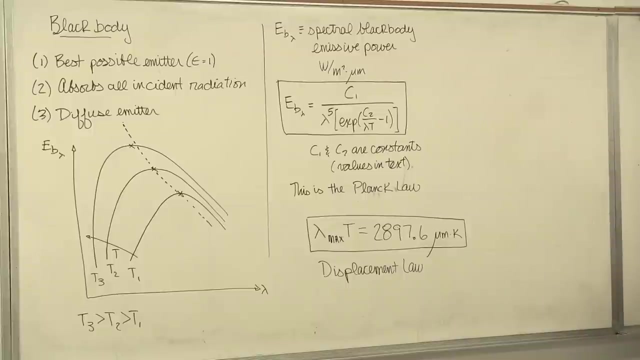 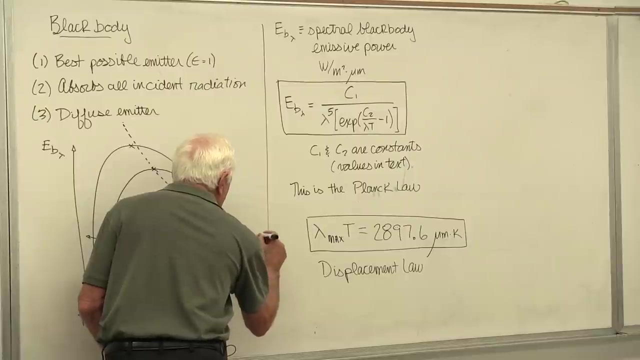 Let's box him in. This is called the displacement law. Let's see what it's telling us. All right, I'm going to put in a temperature of 300.. So if this line right here has a temperature of 300 k, this is what this says. 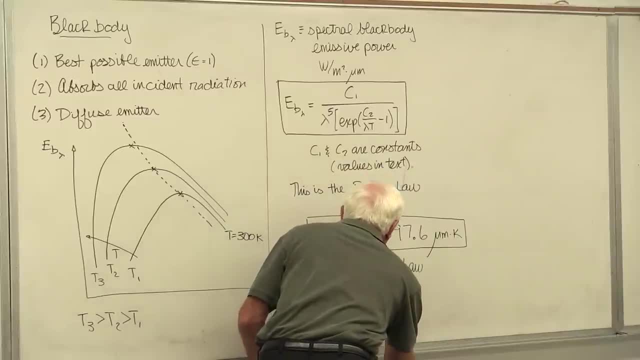 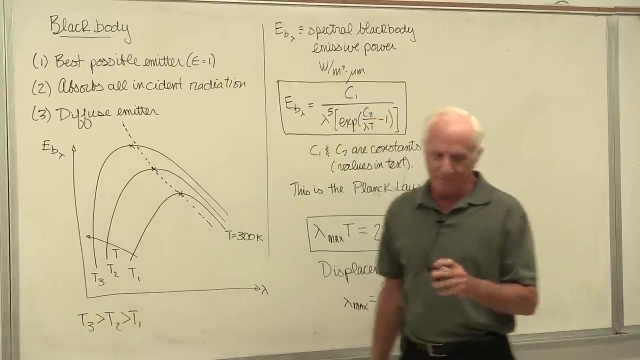 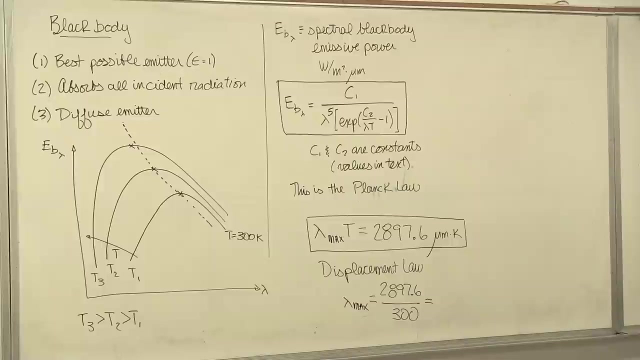 Lambda max equal 28, 97.6 divided by 300.. Now, don't forget, we're in chapter 12 and 13.. Every temperature, every temperature better be an absolute. So you got to shift gears. All right, 28, 98.. 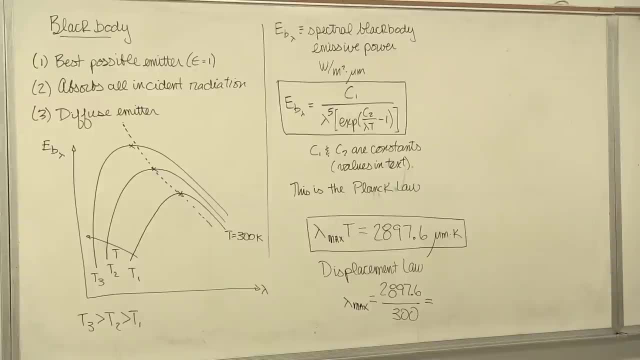 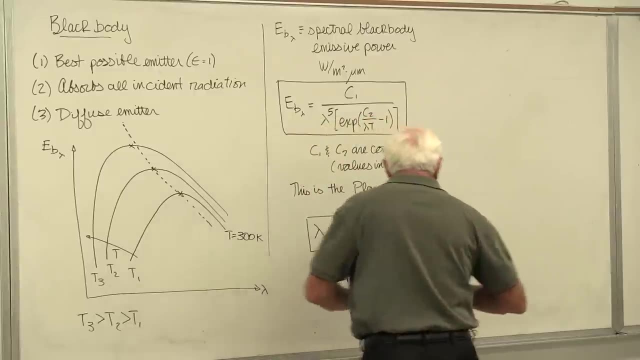 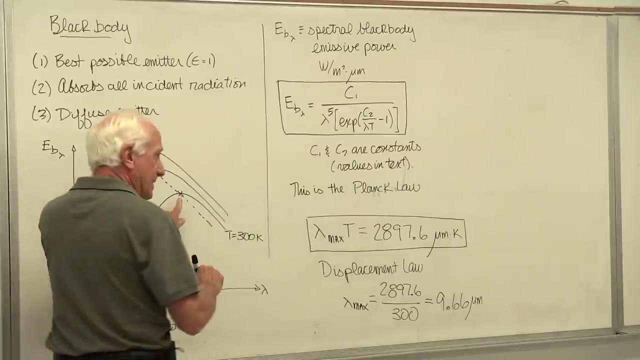 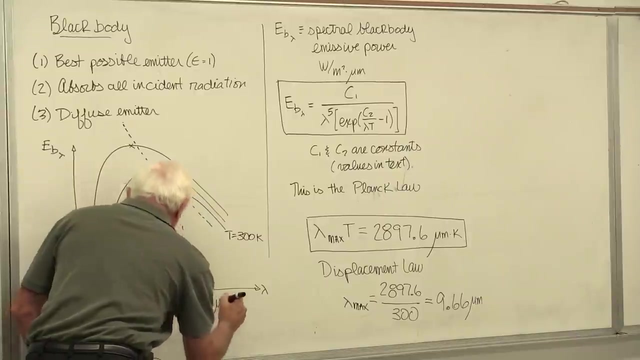 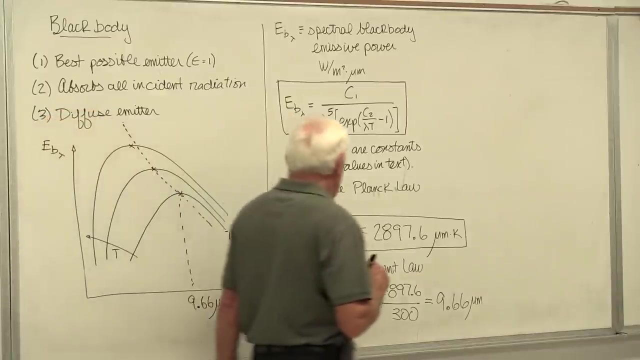 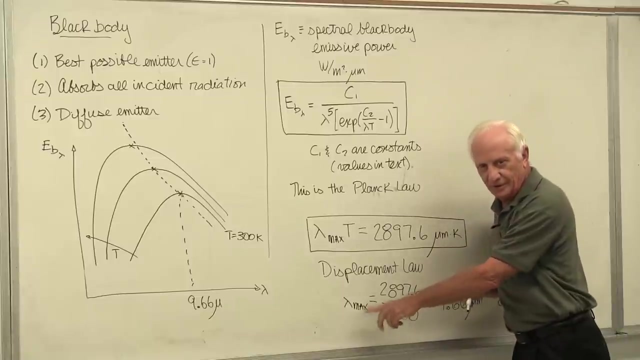 Divided by 300.. 9.66.. Almost Okay. That peak right there occurs at 9.66 microns. So make sure you read that equation right. Don't read it this way. This is the maximum wavelength. No, no. 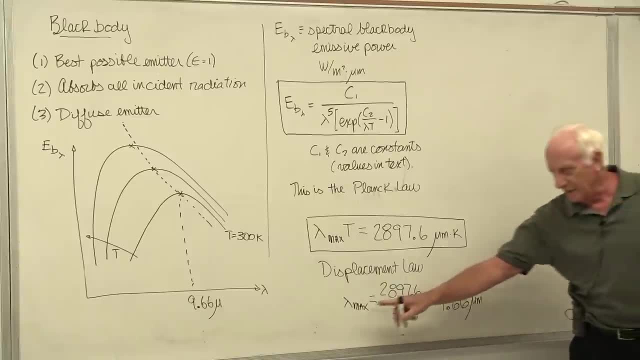 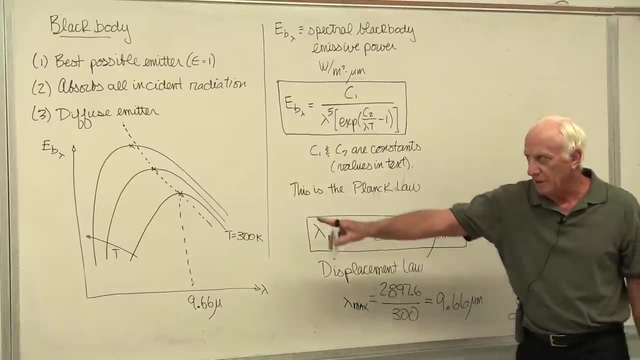 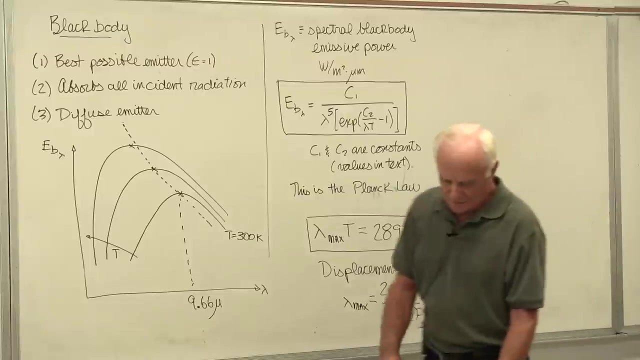 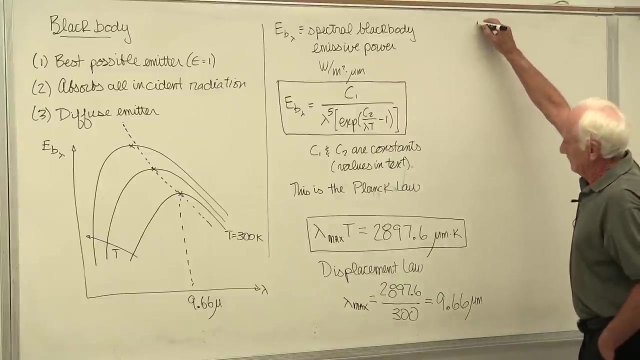 You got it all wrong. It's not the wavelength, It's the wavelength at which the emissive power is a maximum. The wavelength at which the emissive power is a maximum, It's called the displacement law. And then, if you take one particular temperature, 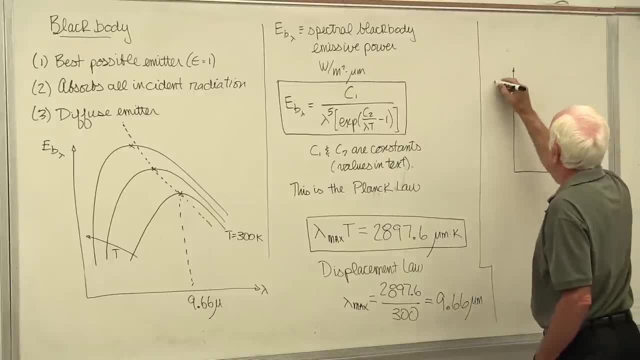 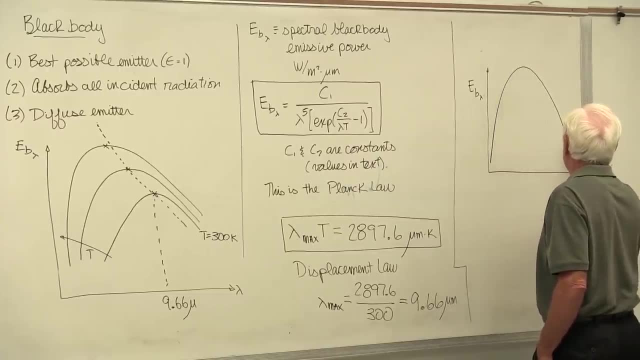 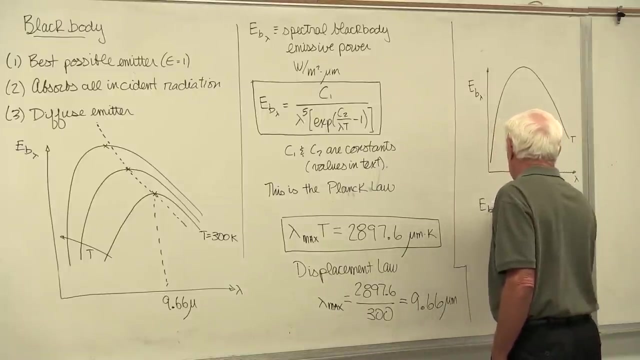 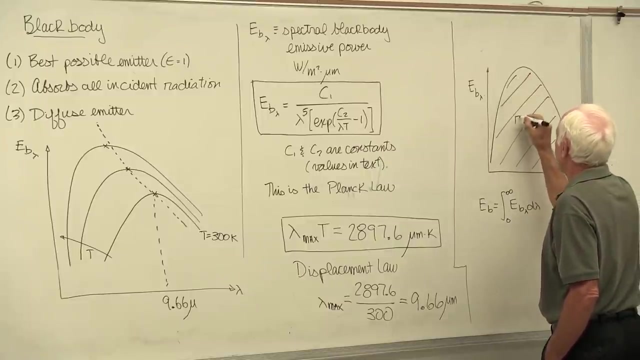 and plot this for one particular temperature, T, and integrate this from over all possible wavelengths, which would be the area under the curve, that's Eb. Integrate it over all possible wavelengths. Boy, does an interesting thing come out When you do that integration, which is 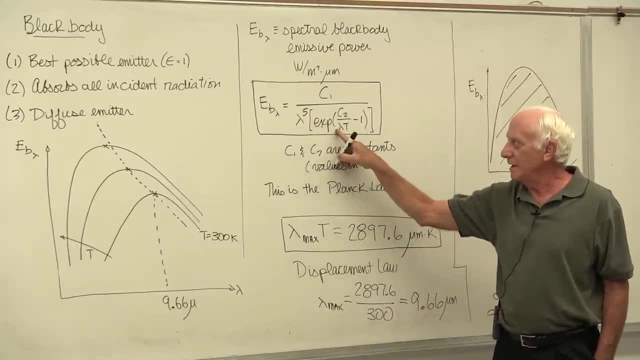 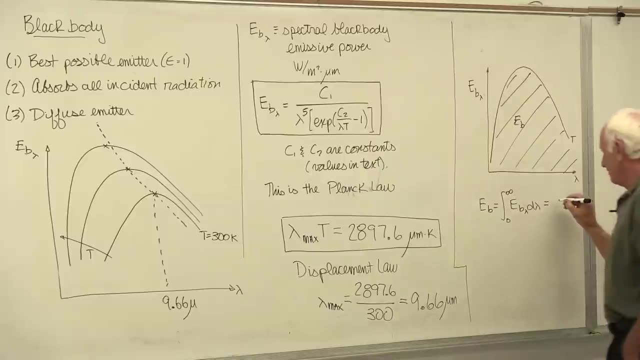 looks pretty nasty. there, There's a lambda. There's a lambda, Go ahead and integrate it. Wow, you know It's not memorized. I don't think You get a very simple result. Hard to believe. Sigma, a constant. 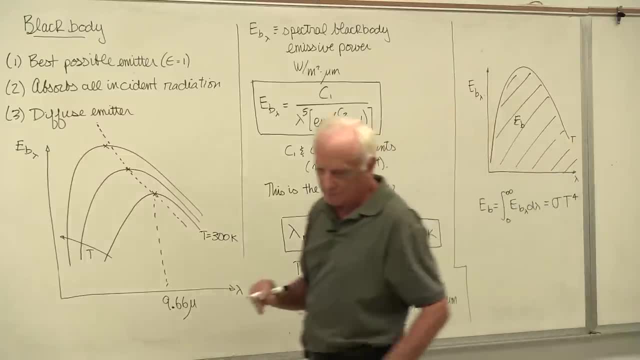 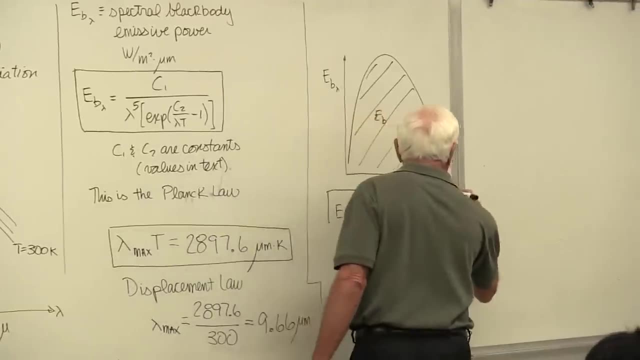 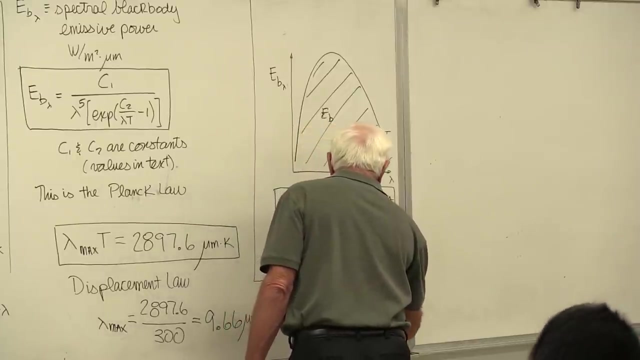 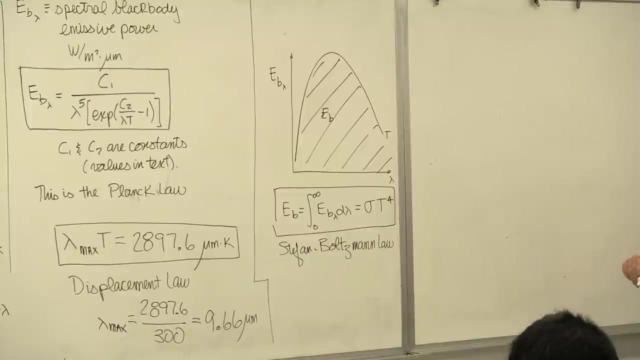 And T to the fourth. That's all it is when you integrate that- We've had that back in chapter one- that the Stefan-Boltzmann law- It's the area under Planck's law curve, The constant sigma. You know what that was. 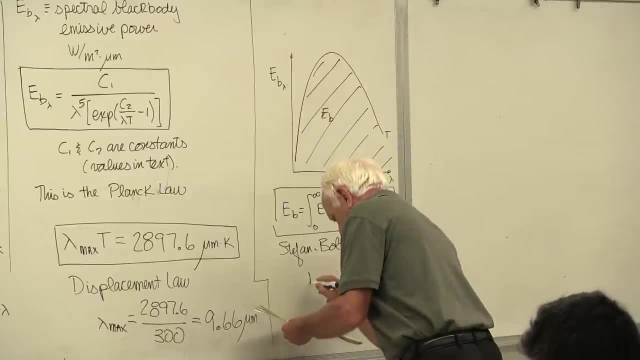 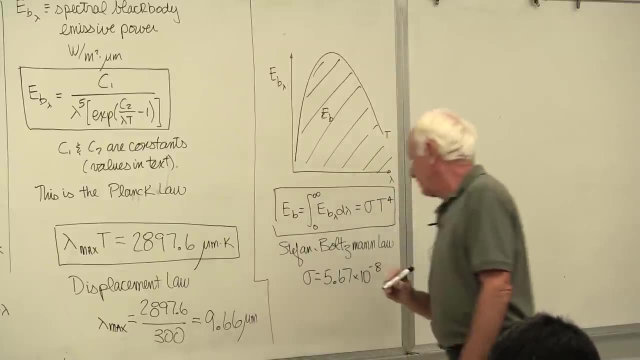 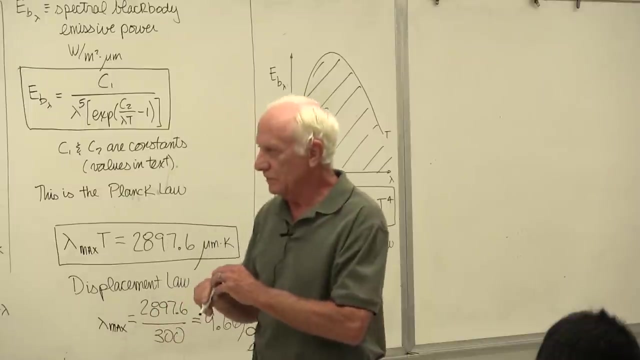 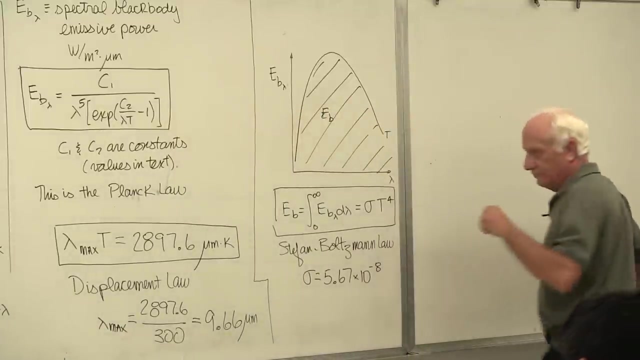 We have that in our notes. I'll put it down anyway, Sigma. Okay, That's the absolute temperature. That's the absolute temperature. Um, You go outside and the temperature is minus 100 degrees Fahrenheit. The surface is icy. Put your hand close to it. 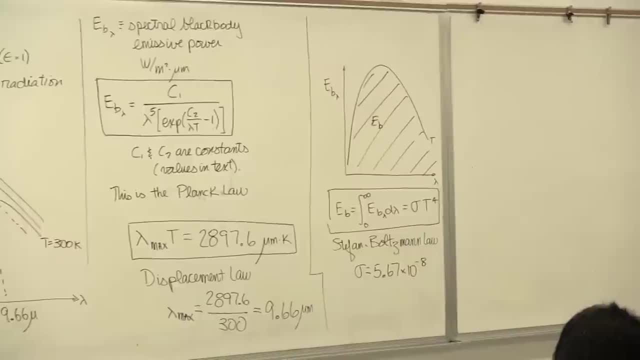 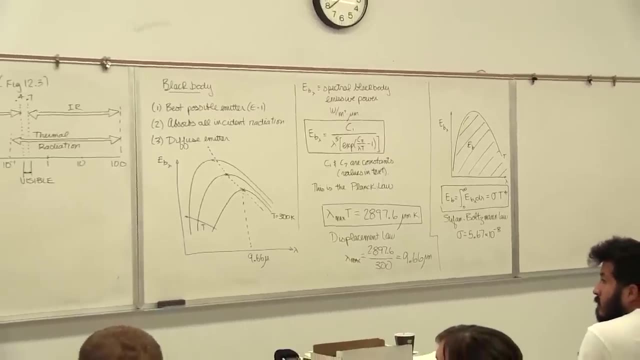 I don't think it's emitting radiation. Temperature is minus 100 degrees Fahrenheit. My hand doesn't feel warm when I put it near the sheet of ice. But is it emitting radiation? Let's assume the ice has a black body. Oh yeah. 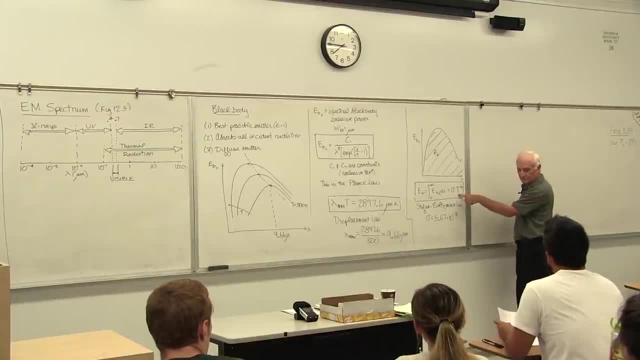 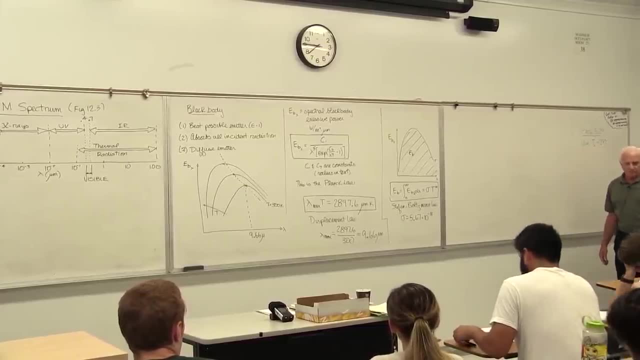 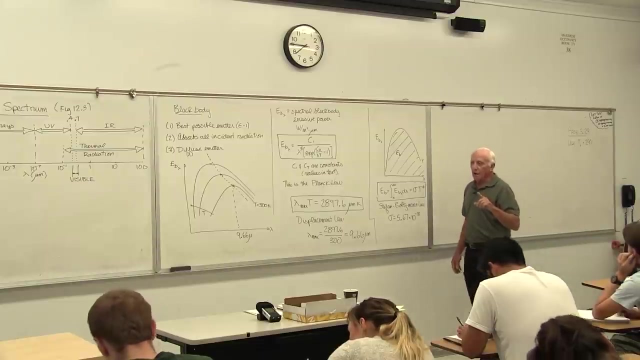 Anything above absolute zero emits radiation, no matter how cold it is. Temperature: One degree Kelvin, One degree Kelvin Just above zero, Is it emitting radiation? Oh yeah, How much? One to the fourth is one Times sigma. How much radiation? 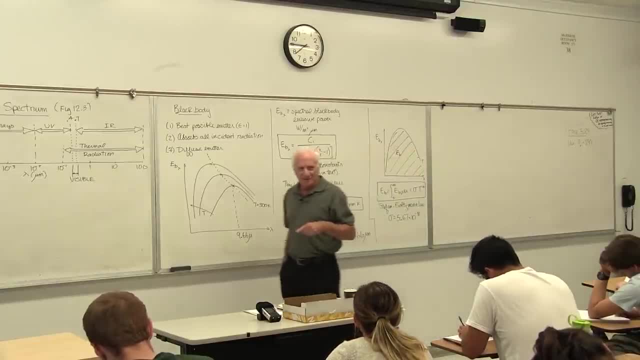 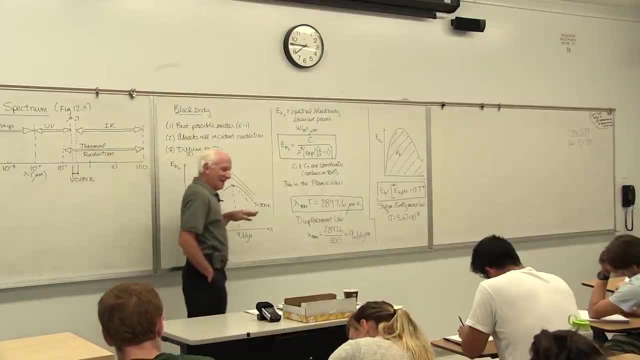 Oh my gosh. 5.67 times 10 to the minus 8.. Watts per square meter- Not a lot, But it is emitting radiation. So the lesson is: every temperature above absolute zero emits radiation. This wall, take one square meter. 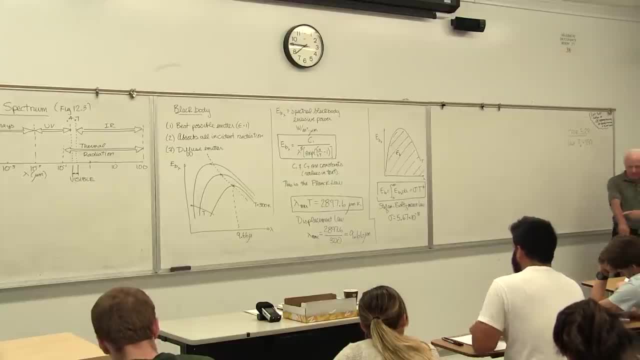 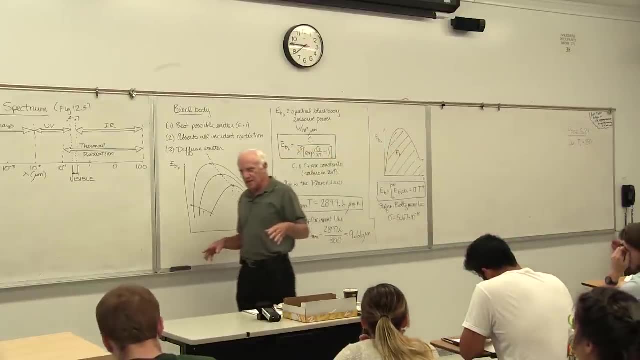 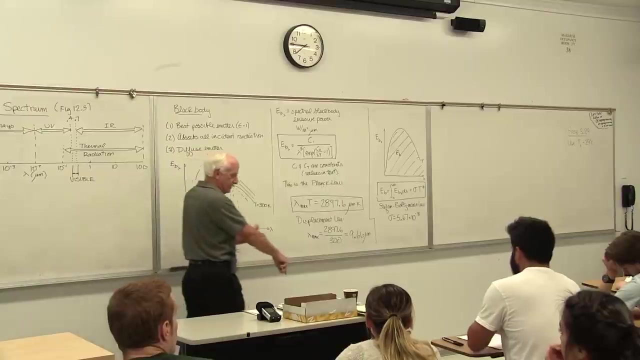 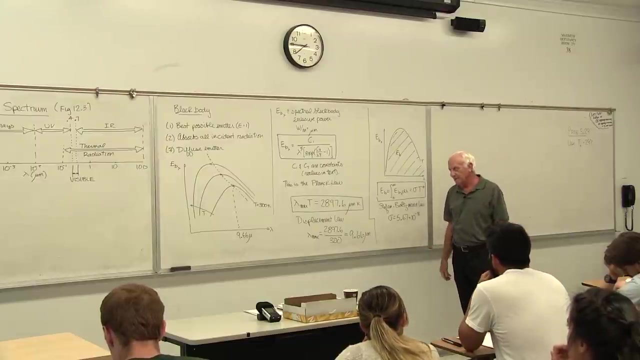 It's emitting radiation. My skin: take one square centimeter, It's emitting radiation. Everything in this room is emitting radiation. Exchange it between here, the front wall, you the floor, the ceiling, the back wall- Radiation Radiation going all directions from our surfaces: my skin, the linoleum, the tile, the acoustical tile, the whiteboard- oh yeah, they're all emitting radiation. 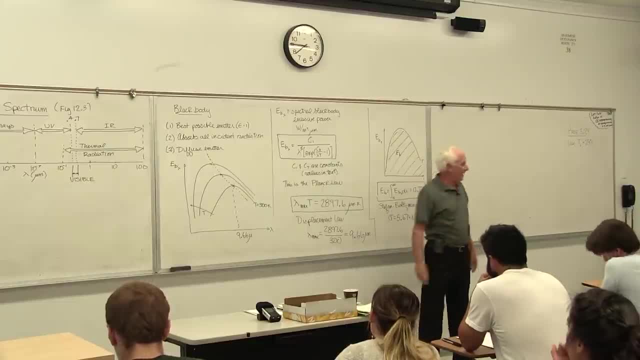 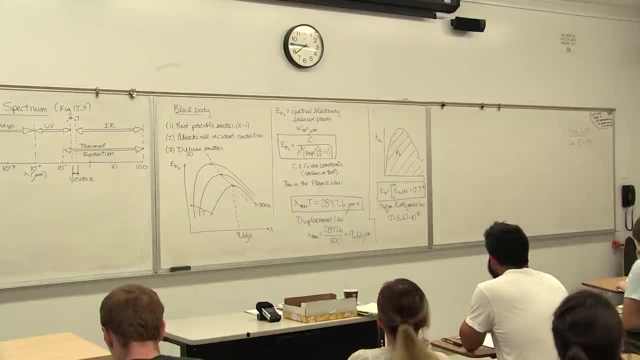 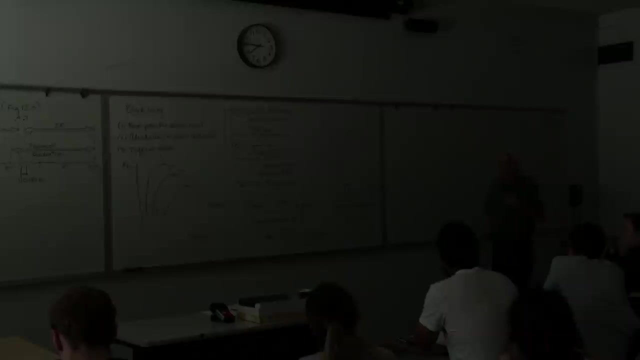 Now if I, if I were to block out those blinds, totally block out those blinds, no natural light, and I turned the lights out in this room, I guarantee you you couldn't see a thing in here. You would be like totally blind. You'd see blackness in front of your, in front of your face. 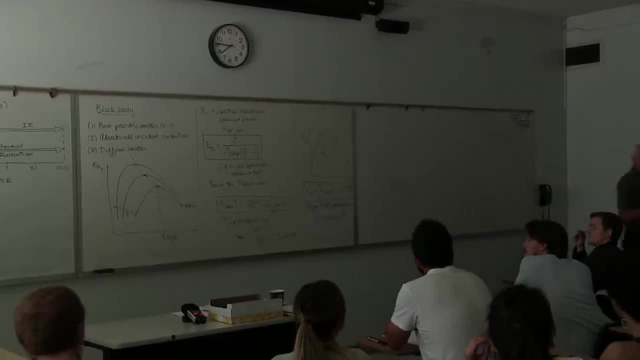 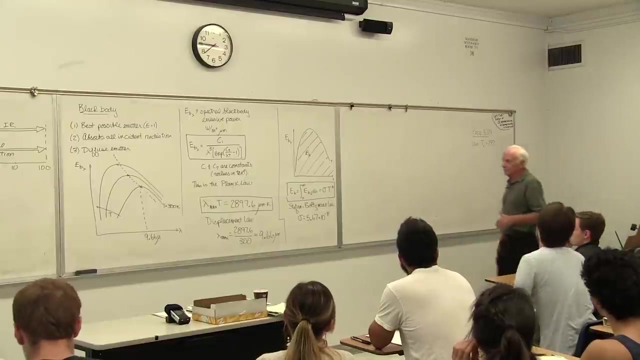 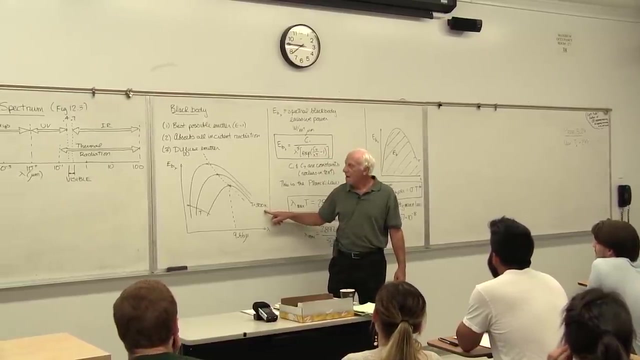 But when I, when I opened the blinds up, you see natural light And I was like, hey, I can see. now It's my friend Joe in here, Yeah, you can see. all of a sudden, You know well what's going on. Well, the room, everything here is about this temperature. 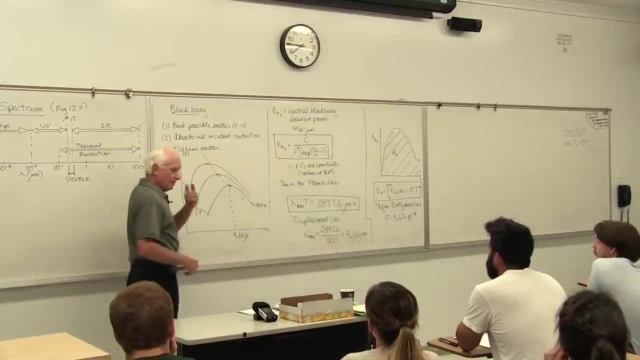 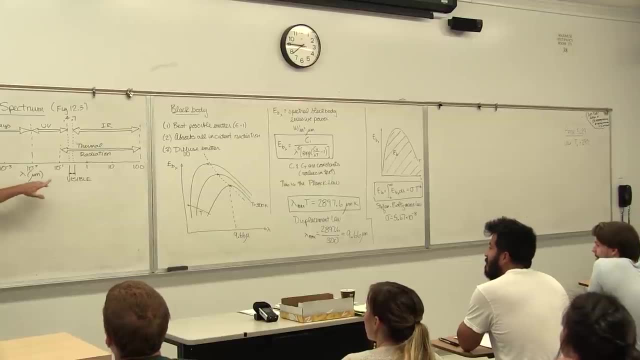 Where is it Where? where are these things in my head? Good detectors, Eyeballs, Good detectors, Look at it. What's the wavelength Maximum Seven-tenths, What's the wall radiating at Ten microns? 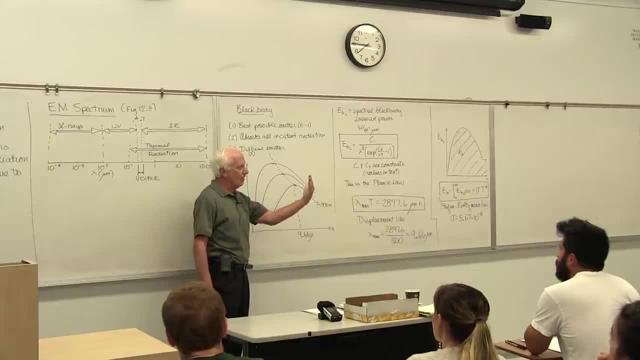 Can I see the wall? Of course I can. Can I see my hand? Of course I can. Why not? Because my hand is a little above 300.. I can't see it. I can only see stuff from four-tenths to seven-tenths. 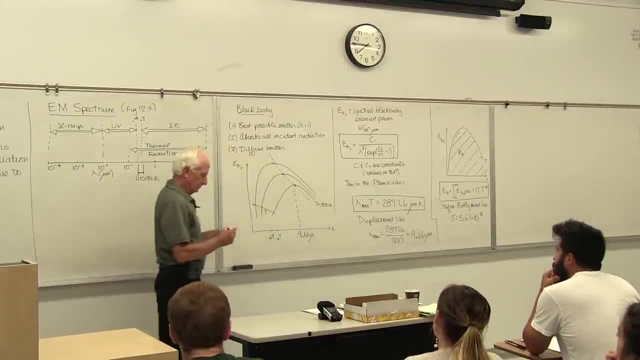 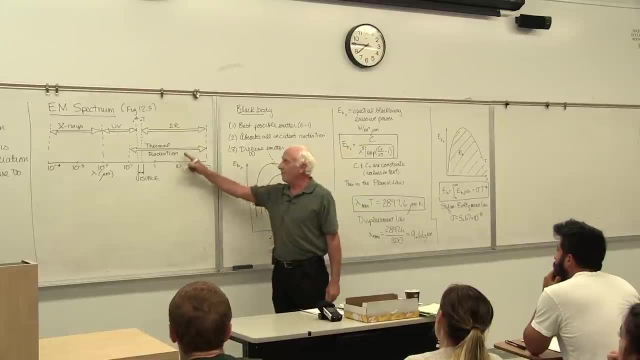 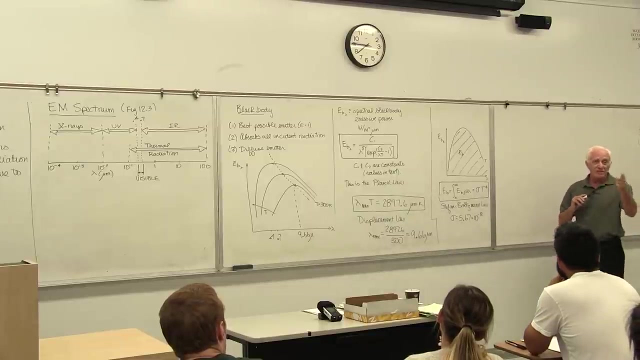 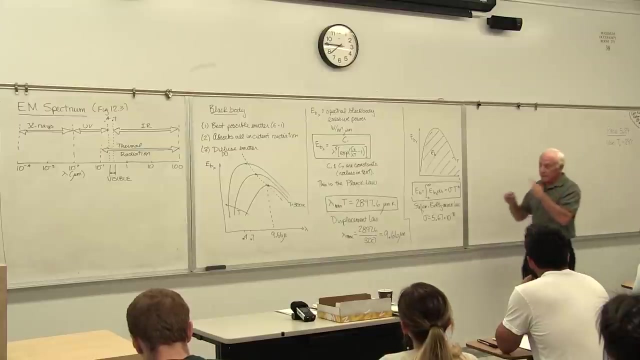 Okay, Yeah, Unless. where does this radiation occur? Look over here Ten. Oh, guess what? Infrared. Unless I put my military infrared goggles on and go out at night, and I'll see you out there at night Because I'm wearing infrared goggles- not my eyes, but something that helps my eyes to see body temperature 300 right here, infrared goggles, Yeah. 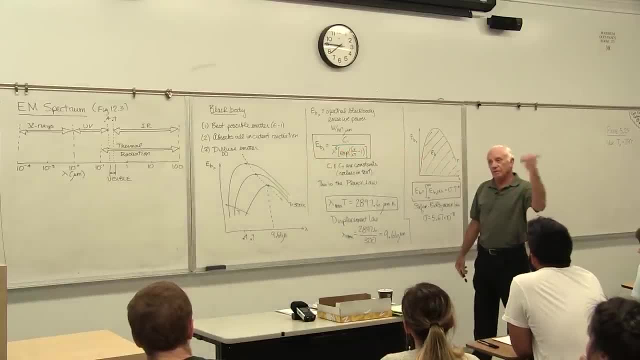 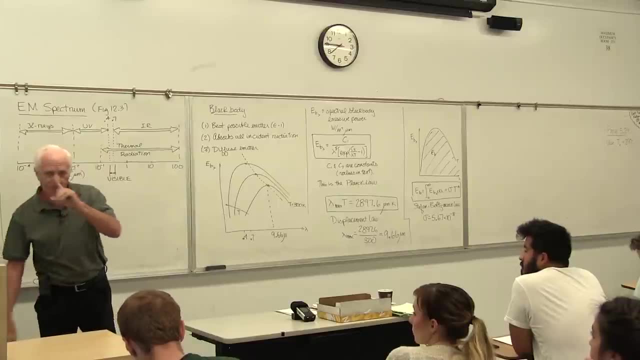 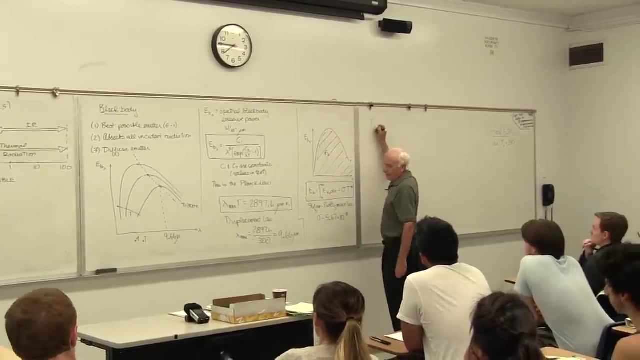 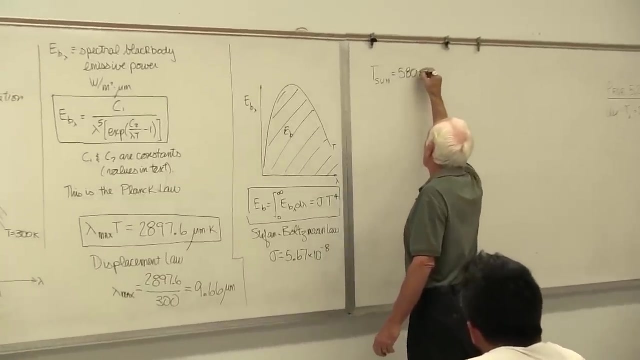 Uh-huh. If I turn the lights out and open the blinds, I'll see in here. Why? Because natural light comes through that window. Natural light. People have found out that the equivalent black-body surface temperature of the sun, the equivalent black-body surface temperature of the sun, is about 5,800 Kelvin. 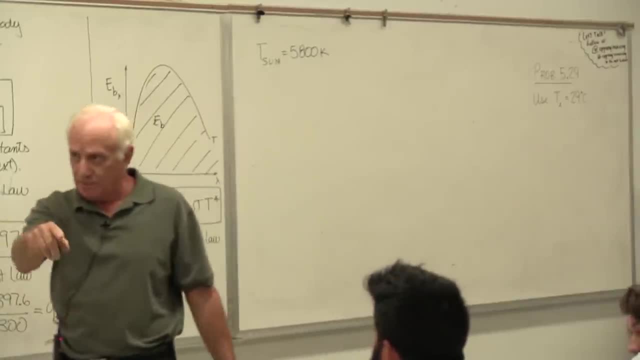 So when that radiation comes through that window and strikes that desk, it's about 5,800 Kelvin. So when that radiation comes through that window and strikes that desk and strikes your body and strikes the floor, it comes to my eye. It's from the sun. 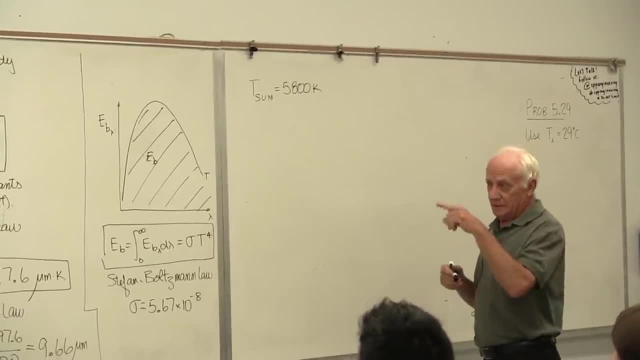 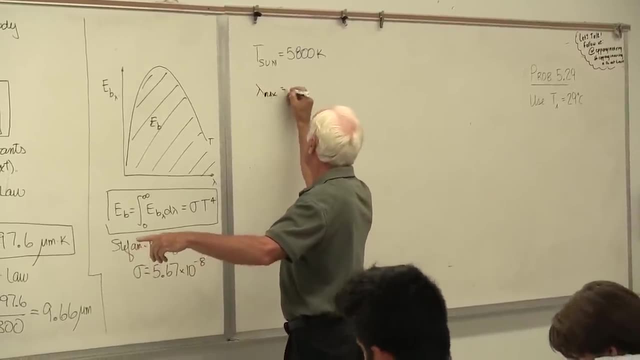 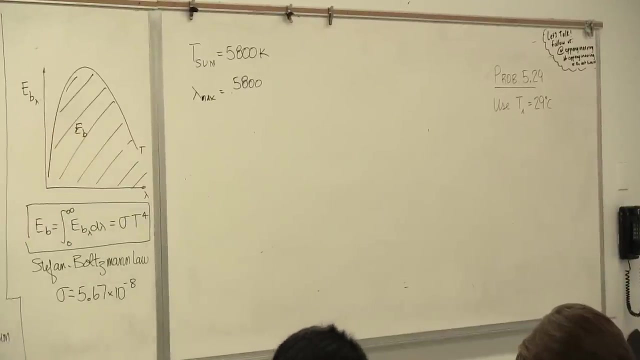 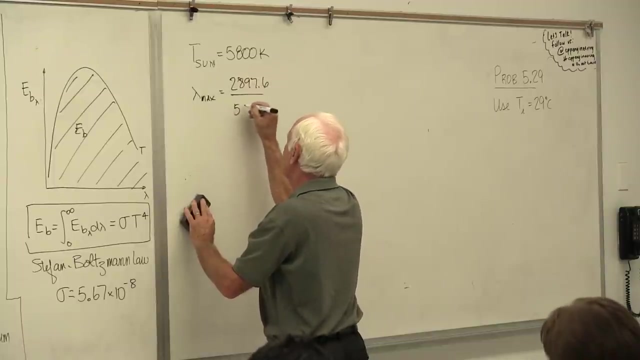 If these lights be. now Let's see where it is. Lambda max T. Lambda max 5,800.. Uh, oh, not 5,800.. 2897.6.. 2897.6.. Divide it by 5,800.. 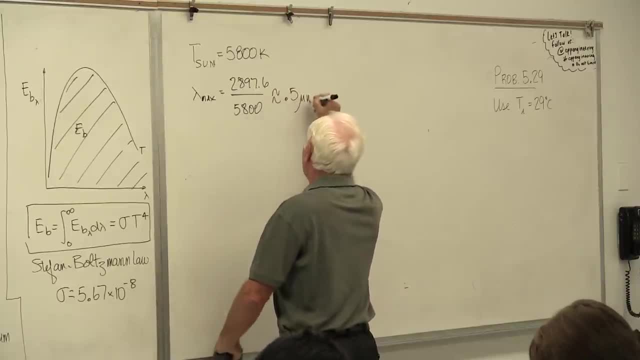 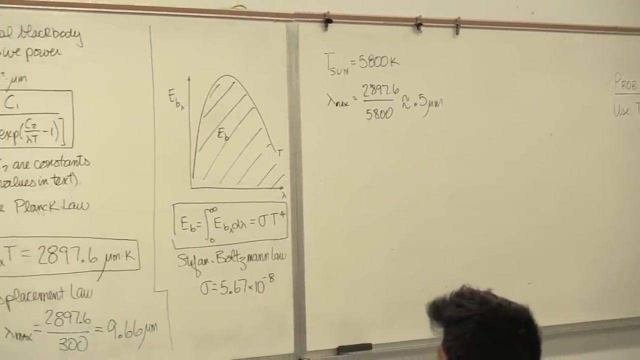 Oh, boy, that's. I have the mic on, So here's the graph. Here's the temperature, the equivalent temperature of the sun, 5,800 Kelvin. right here, Where does the maximum occur? Oh, surprise of surprises. 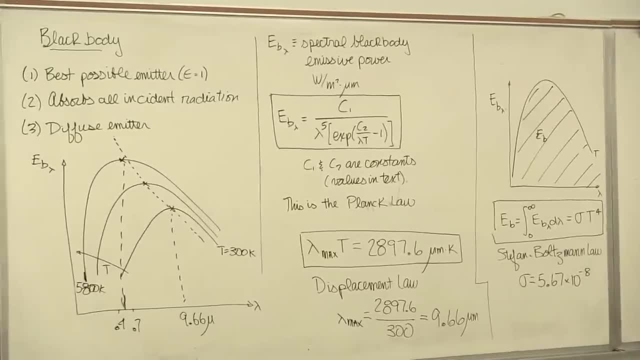 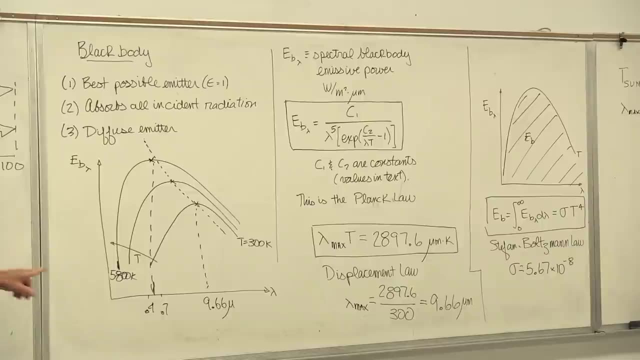 Right in the middle of my transducer's maximum sensitivity. It's called my eyes. So when the lights are out and through the window comes natural light, of course I see you and the walls and my hand and the desk, Because my eyes are sensitive in that range and the peak emission falls right in the middle of that range. 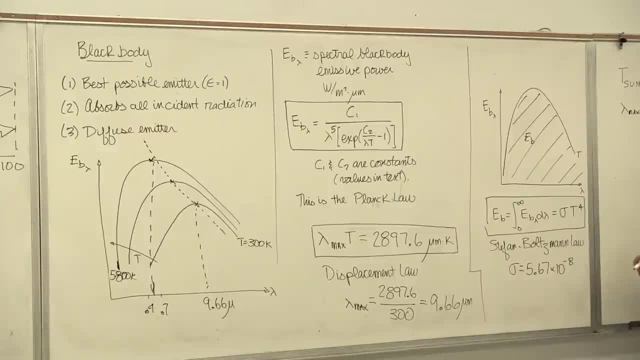 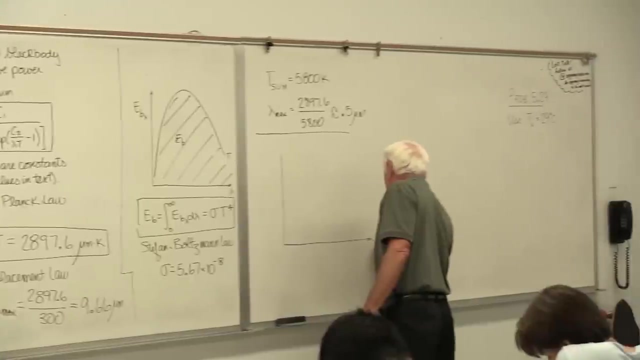 So that tells why we can see in this room with the lights out. Okay, Okay, Back over here again now. All right Now. So sometimes we're interested in not finding the total energy emitted, but we're interested in finding how much energy is emitted between wavelengths of zero and a lambda called lambda one. 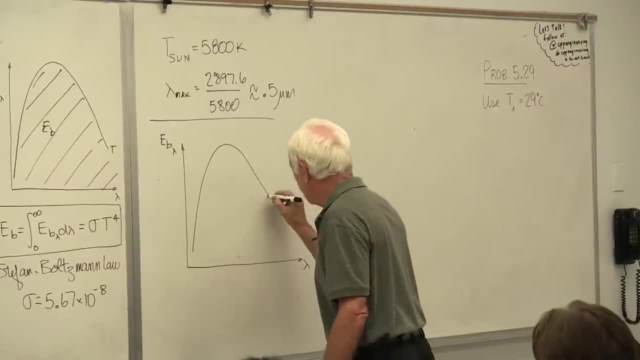 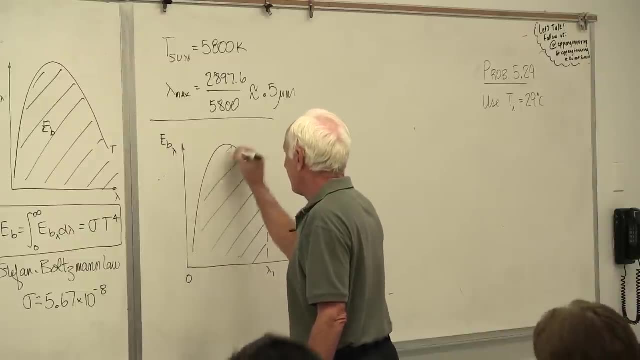 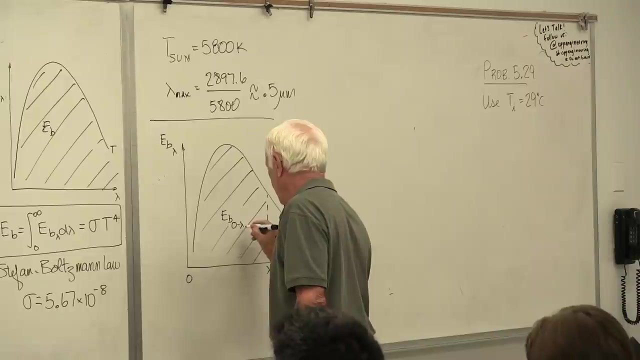 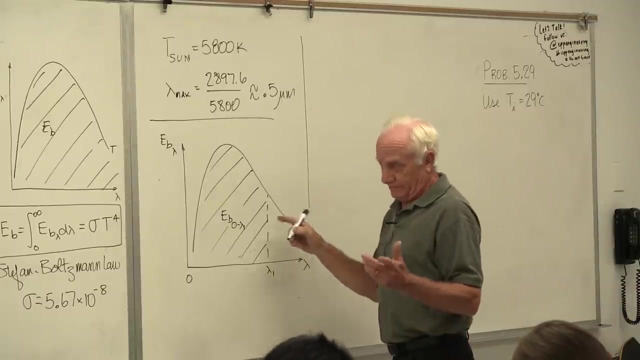 So here's my curve again. Now I want to go from zero out to lambda one. So that would be EB zero to lambda one. Okay, The work. no, you have to integrate this big long expression platform. It's been done for you once and for all. 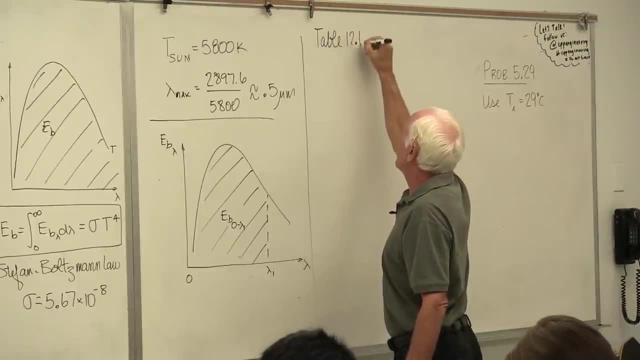 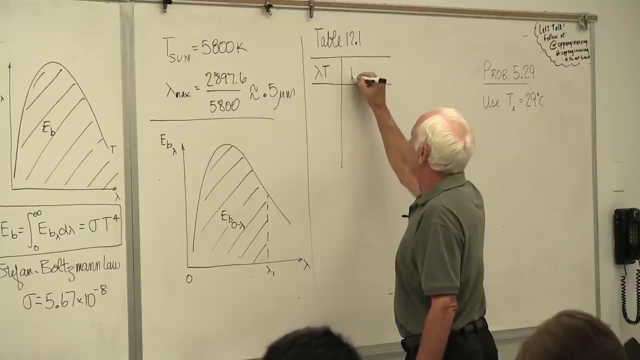 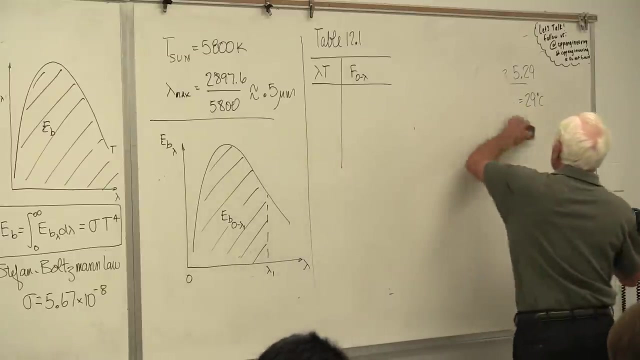 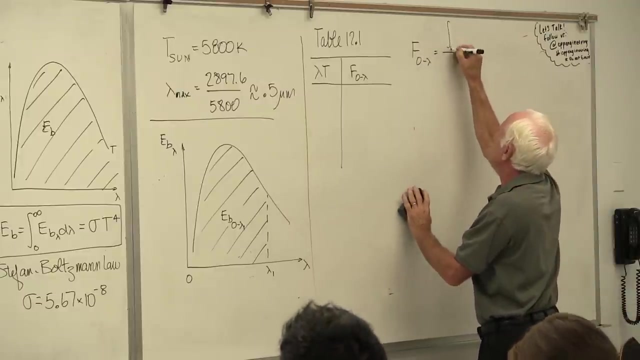 So you go to table 12-1.. The first column is titled lambda T- absolute temperature. The next column is F zero to lambda T. F stands for fraction. It's the integral zero to lambda. EB. lambda D lambda divided by integral zero to infinity: EB lambda D lambda. 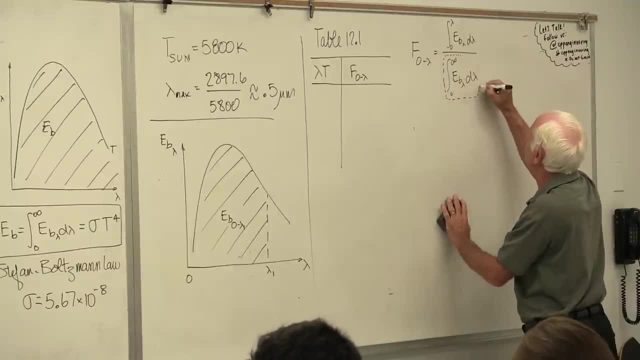 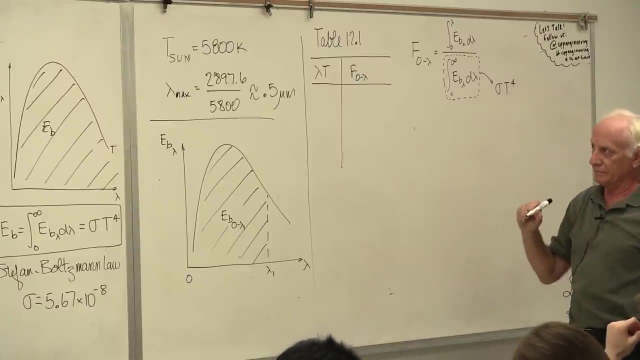 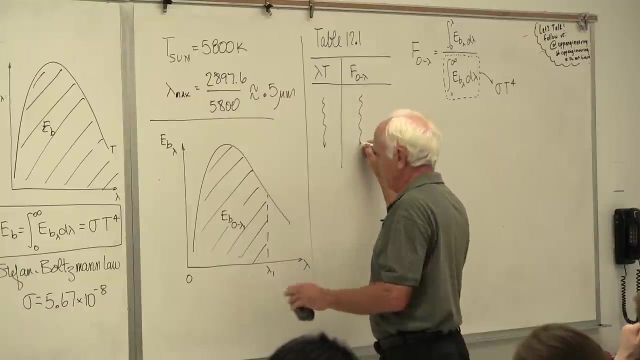 Of course this denominator steps up. It's F and Boltzmann law, That's just sigma T to the fourth denominator. There it is. So in this table I'll just put one value down so you get to see the flavor of the table. 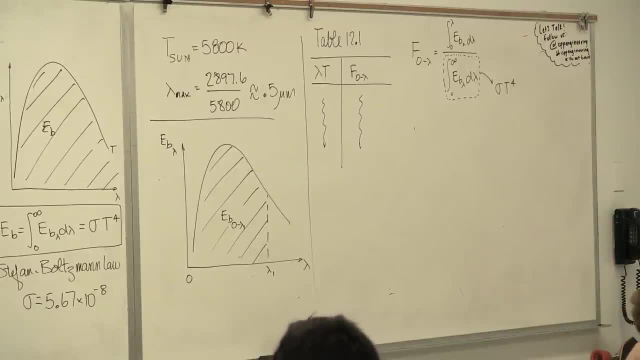 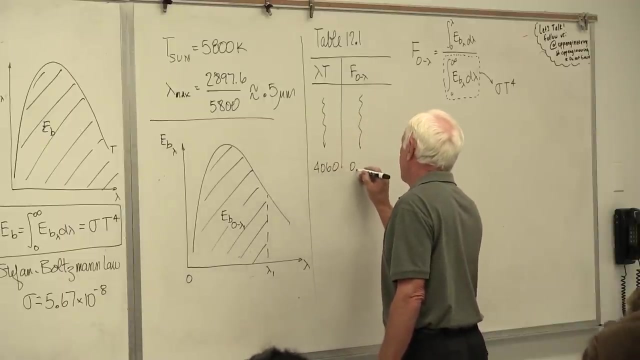 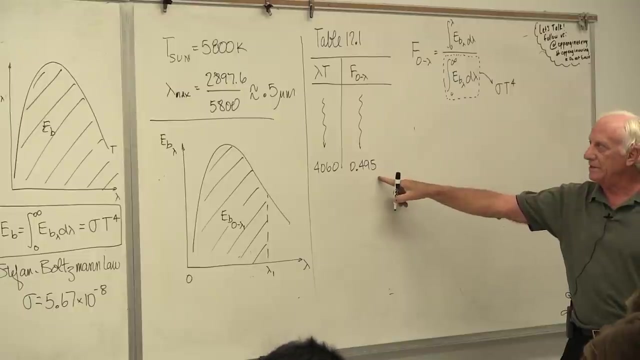 Let's see Table 12-1.. We'll take a lambda T value of 40,, 60, and it's 495.. 40, 60, and 0.495.. So that means 49.5% of the radiation falls between zero and that lambda value, whatever that might be. 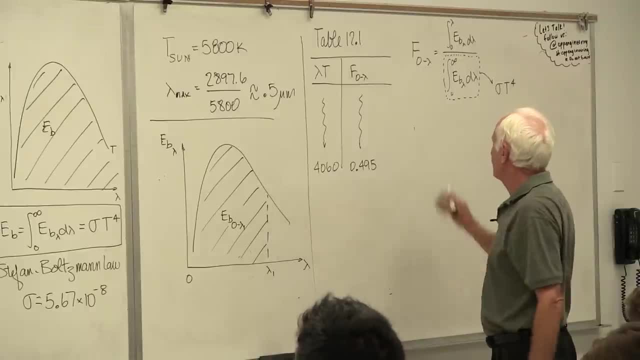 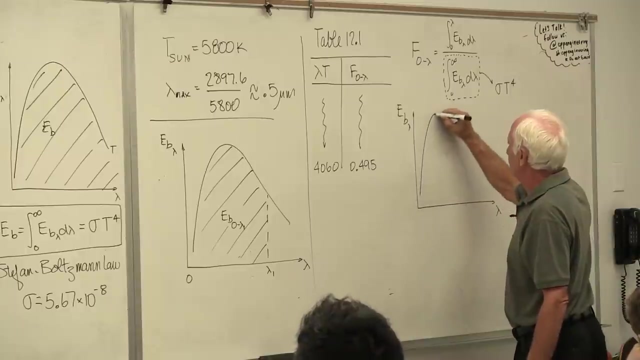 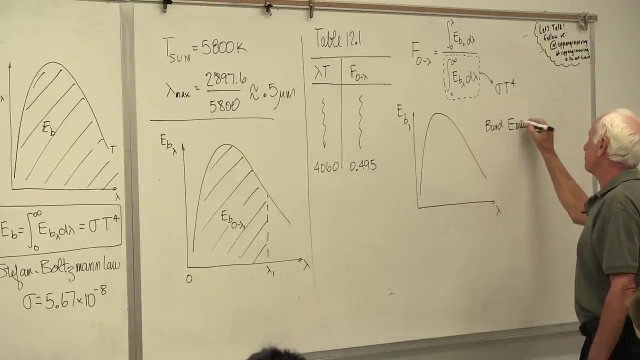 All right, So you use table 12-1 to find this. We want to find the fraction of the emissive power that lies between two wavelengths called band emission, Band emission. So here's lambda 1 and here's lambda 2.. 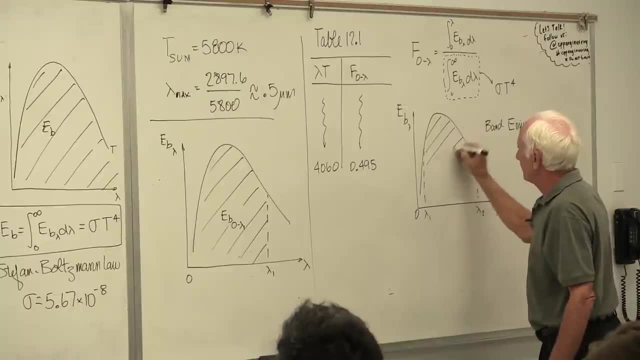 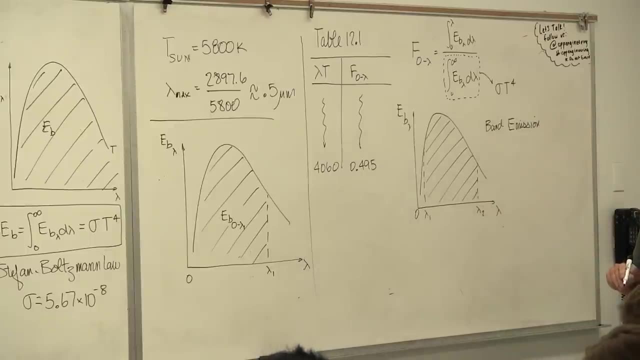 And I'm going to find out how much emission occurs between those two wavelengths, a band between two given wavelengths, The fraction of energy that falls between wavelengths of lambda 1 and lambda 2, you can look at it and it makes sense graphically. 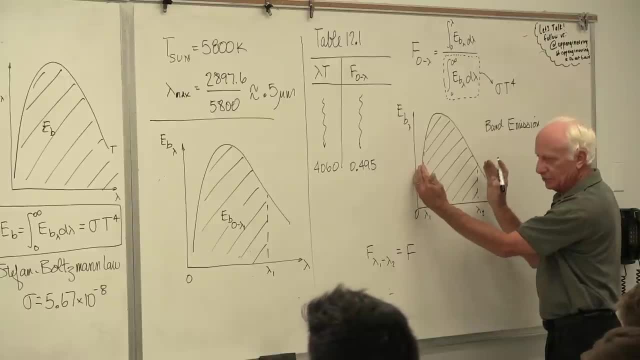 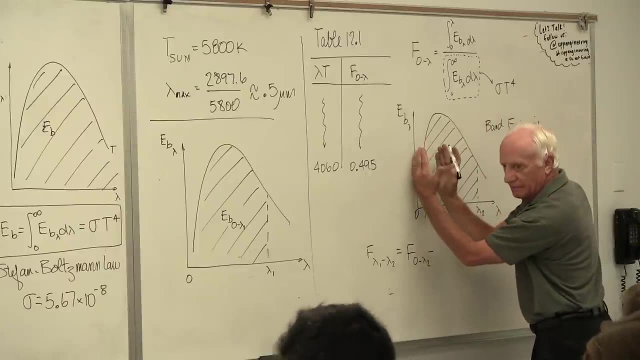 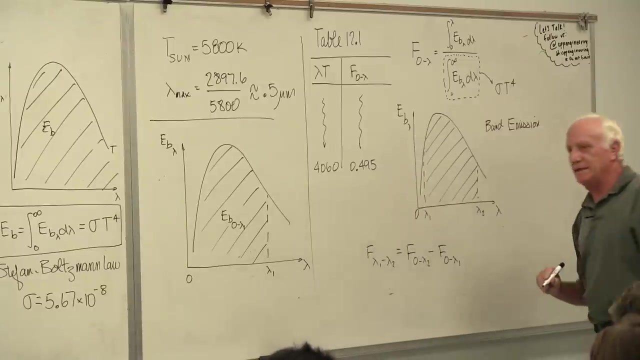 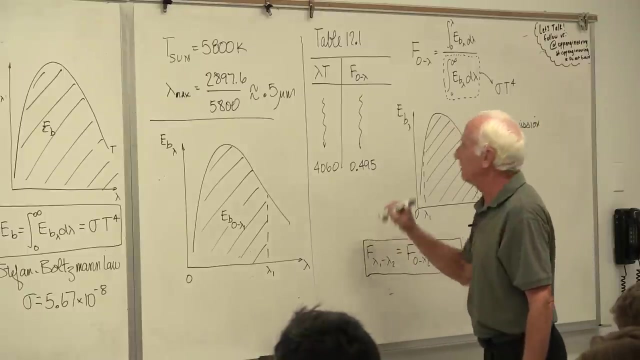 Take the fraction that falls from zero to lambda 2. And subtract off the fraction from zero to lambda 1, this piece, And that gives you the band emission, the fraction from lambda 1 to lambda 2.. So again you use table 12-1 to find a fraction like that. 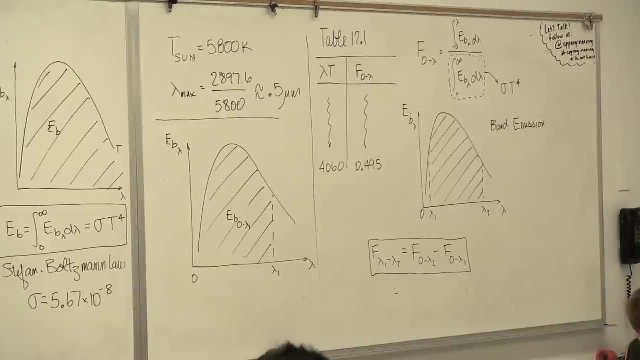 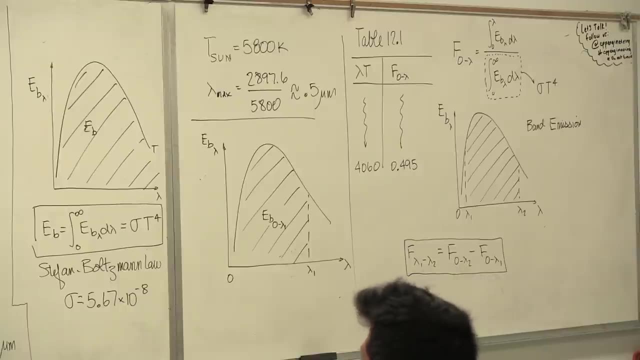 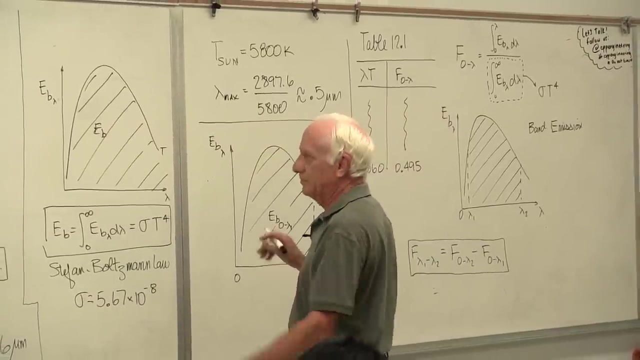 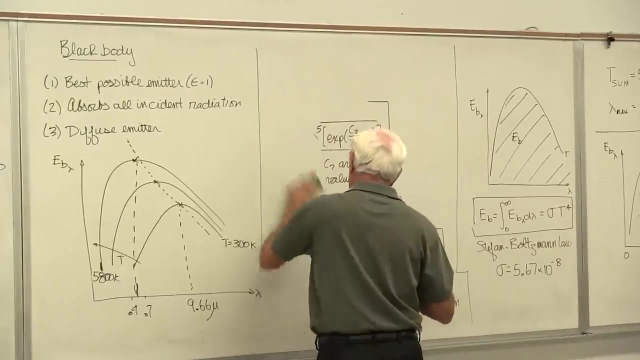 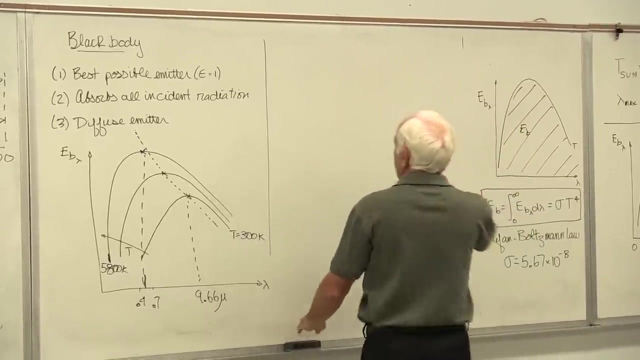 Okay, Let's take a look at an example. then Let's see I'm going to save that. maybe I think I can erase this. I'll put it right here. I don't need this anymore. I'll save this, Okay. 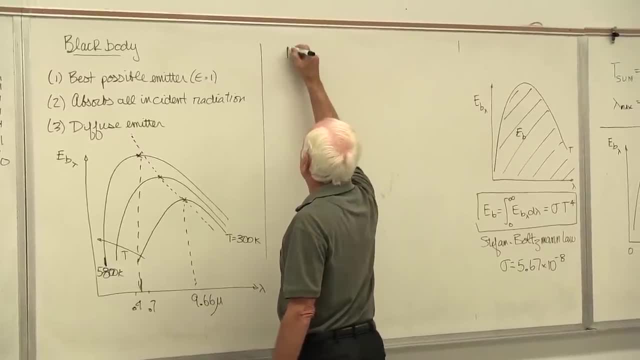 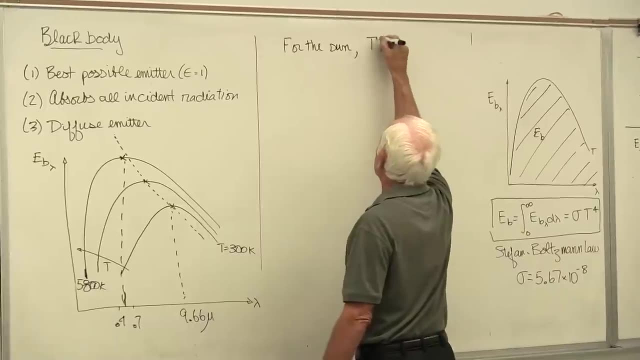 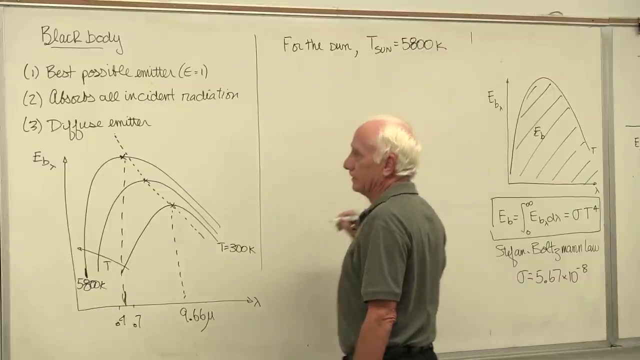 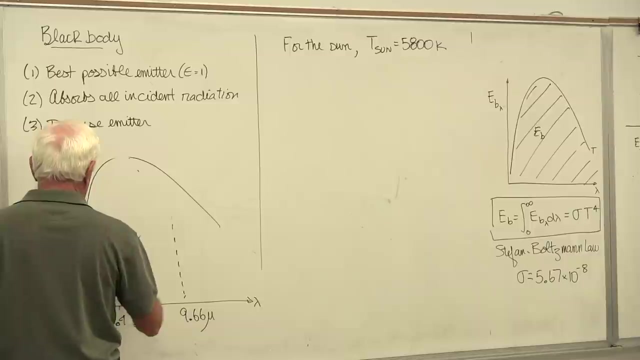 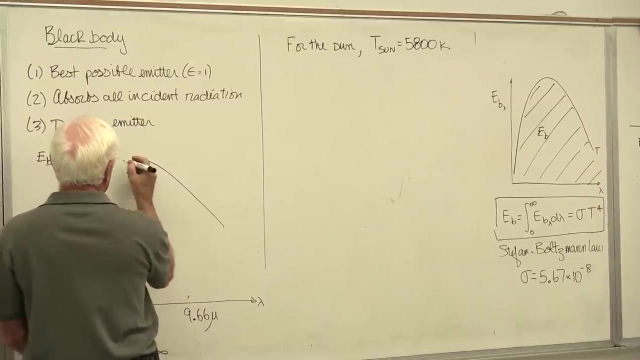 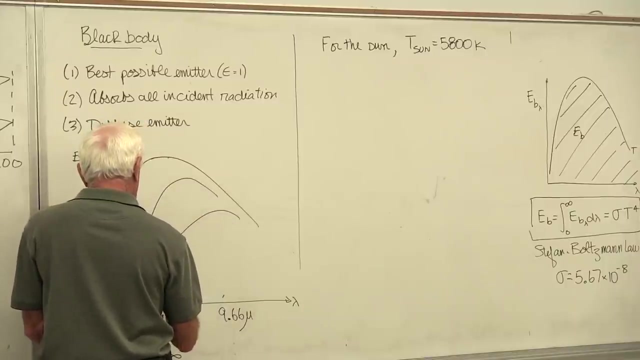 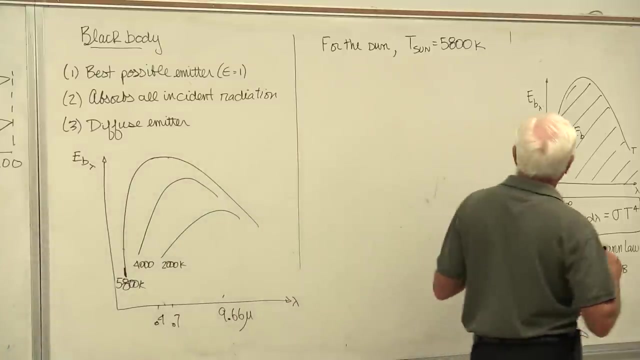 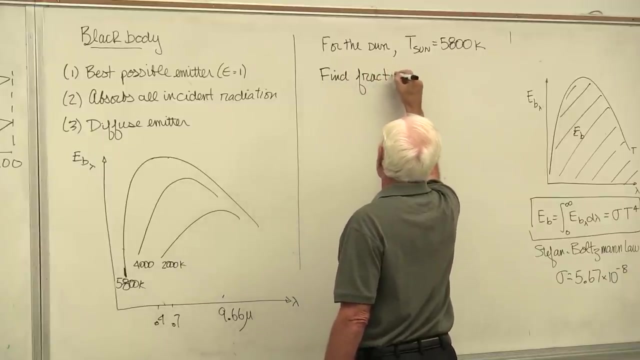 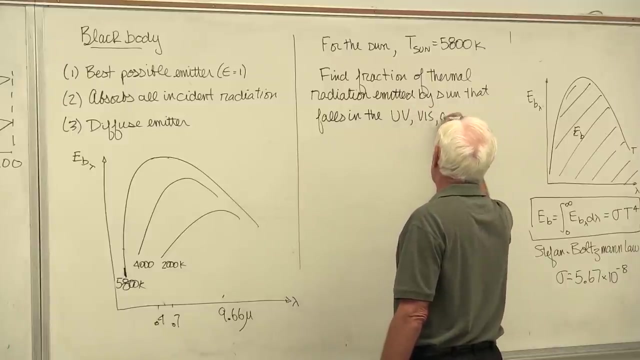 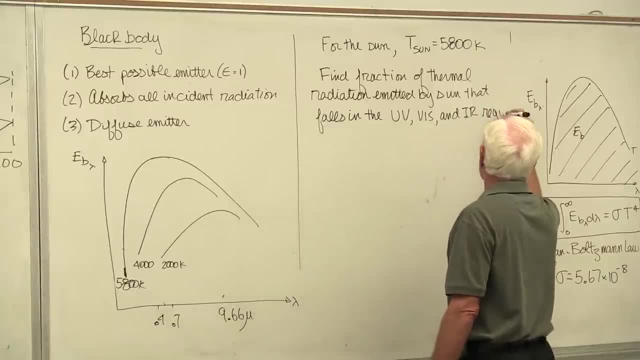 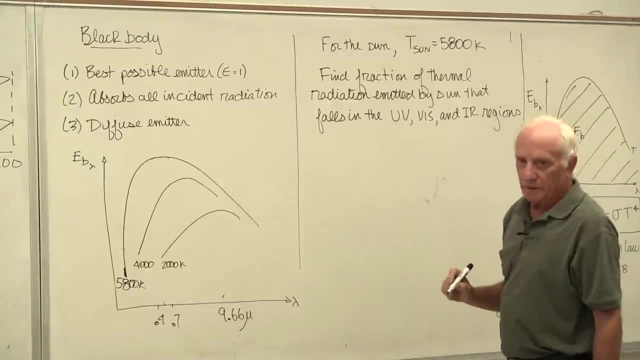 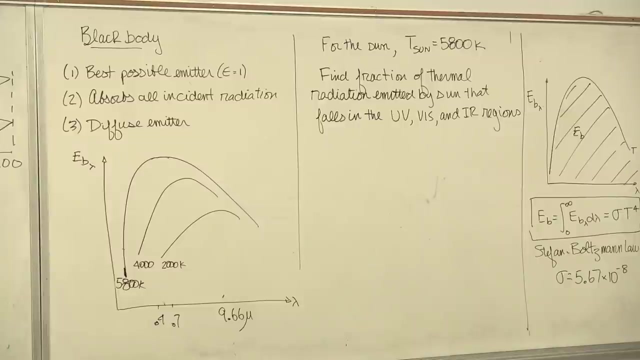 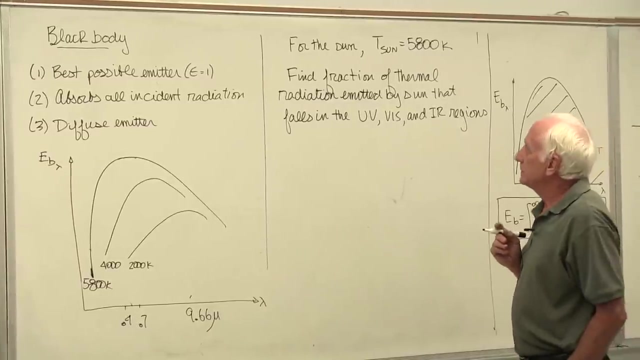 visible and infrared regions. visible and infrared regions. Okay, Don't forget, I said that for us, the sun is being modeled as a black body, Because you know, because you know, at 5,800 Kelvin. maybe I missed it. 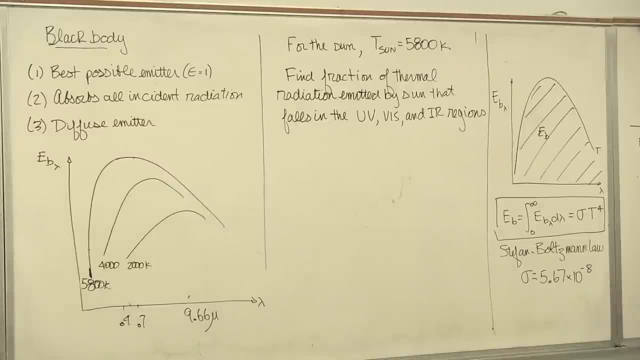 but I don't think they sent a probe to the surface of the sun and landed it on the sun's surface and put a probe there and said: okay guys, the temperature is 5,800.. No, I didn't miss it. 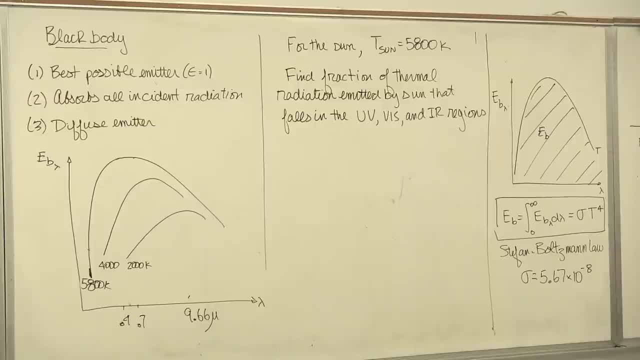 They didn't send a probe into the surface of the sun. First of all, I'm not sure there's even a surface of the sun to stand on. So who made this up 5,800?? Well, they sent a satellite up in orbit. 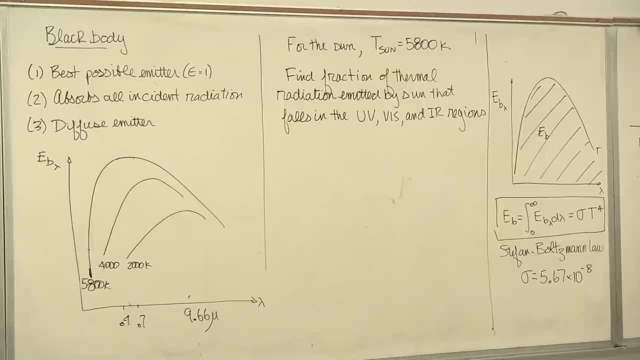 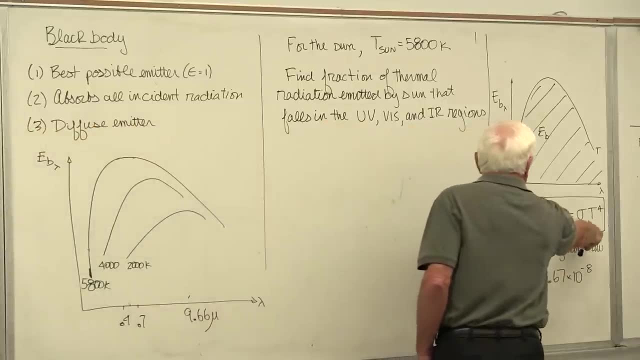 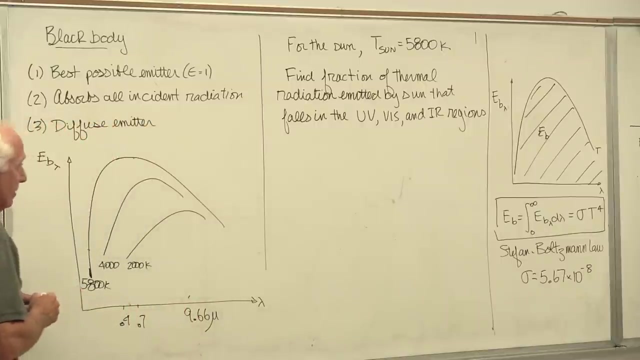 The atmosphere. they pointed its detector at the sun and from that they deduced how many watts per square meter, so on and so forth. Here it's right. here, Assuming the sun is like a black body, They got the emissive power of the sun. 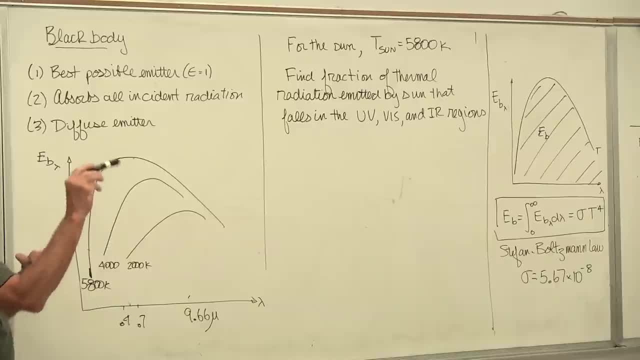 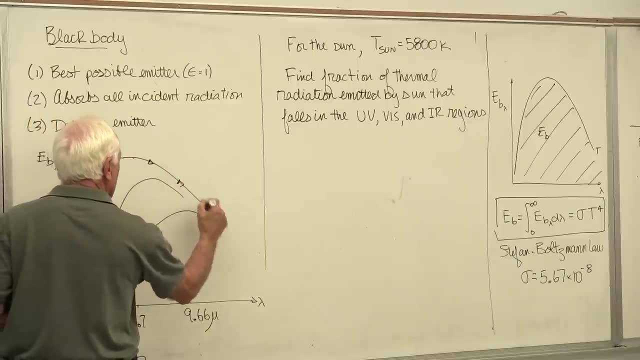 as a function of wavelength, Put different wavelength filters in the transducer And then they plotted data. And lo and behold, if you plot the data and there's graphs in the book that show that They said: gee, it doesn't fit the 2,000 K curve. 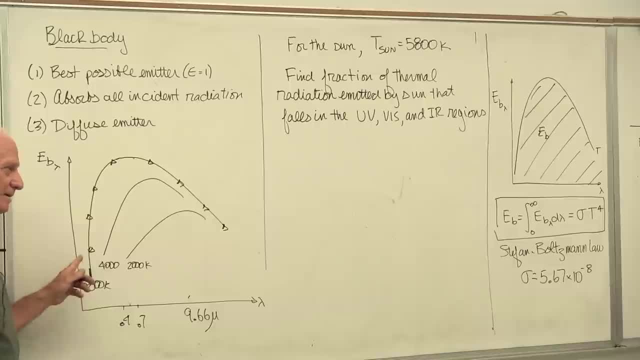 It doesn't fit the 4,000 K curve, but look at that: It almost fits perfectly the 5,800 black body curve. Therefore, we engineers will assume that the sun behaves as if it were a black body at an equivalent temperature of 5,800 degrees Kelvin. 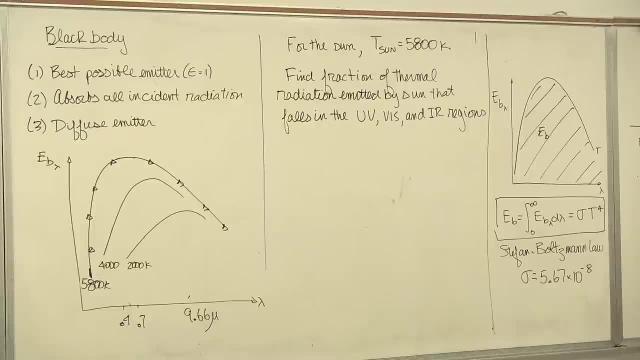 How? By deductions from a satellite in orbit of the Earth's atmosphere. Okay, that's the history. All right, back to this again now. All right, we've got to do the stuff here. Okay, here it is. Here it is. 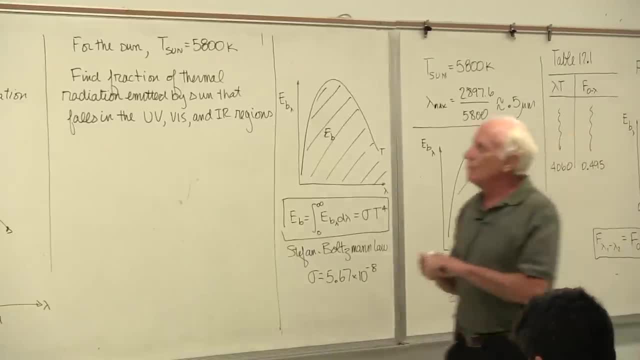 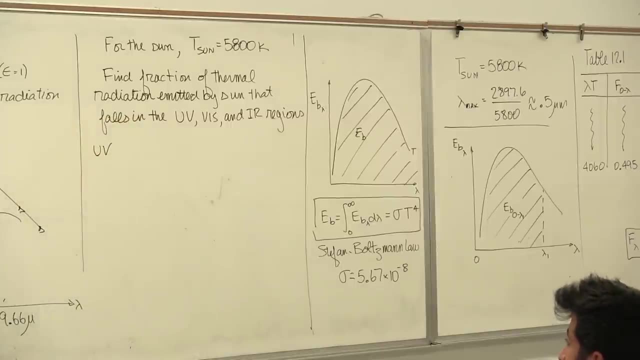 Band emission. I want to go: Okay, let's put it down. Where is UV? Okay, UV, Right there, Don't forget. now, only in the thermal radiation. It says it: right there. Thermal radiation- Okay, from fingertip to fingertip. 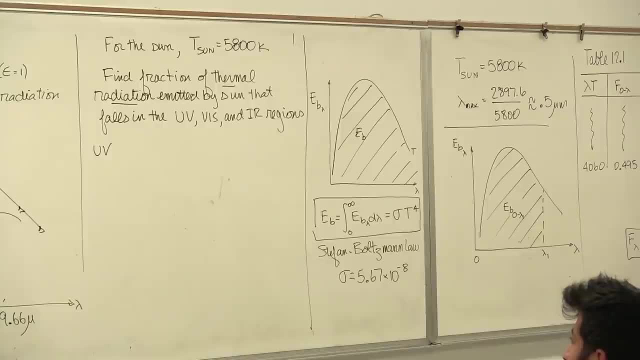 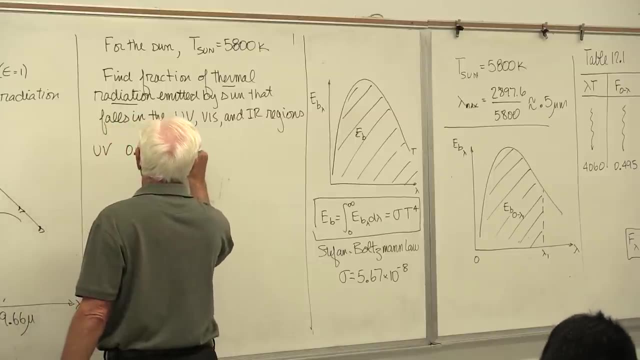 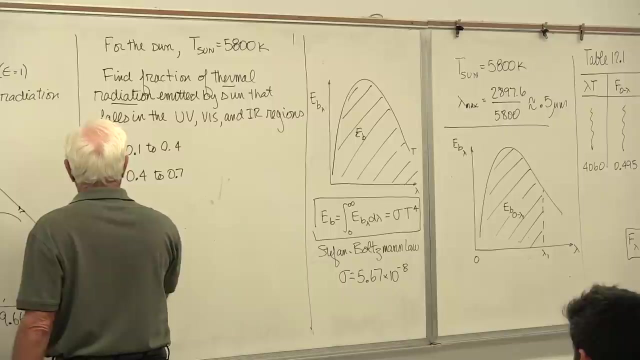 Where is UV there? From 1 tenth to 4 tenths, The 10 to the minus 1.. Okay, 1 tenth to 4 tenths Visible, 4 tenths to 7 tenths Infrared, 7 tenths to 100.. 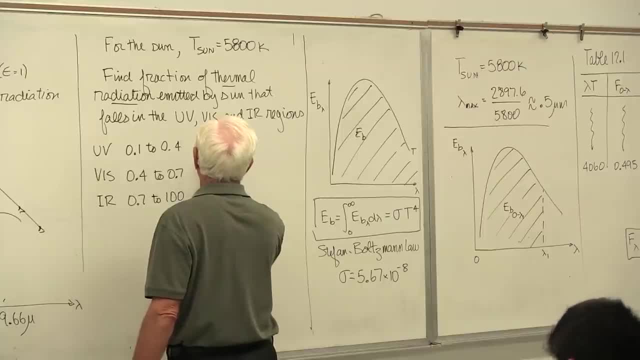 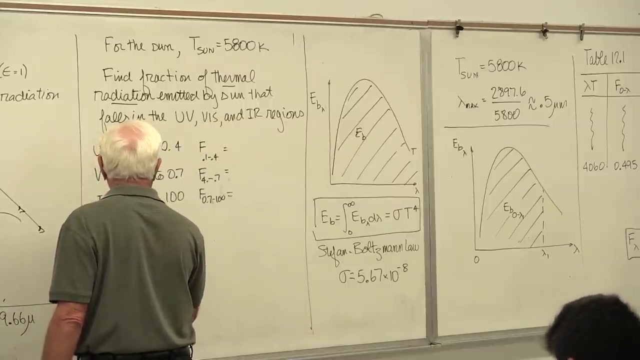 Okay, fraction 1 tenth to 4 tenths. Fraction 4 tenths to 7 tenths. Fraction 100.. 7 tenths to 100.. Okay, let's do lambda 1t. The first lambda is 1 tenth. 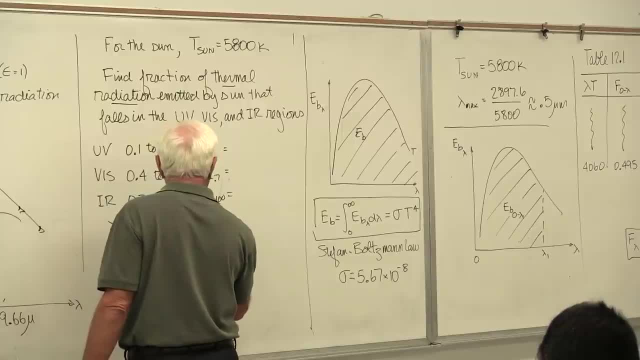 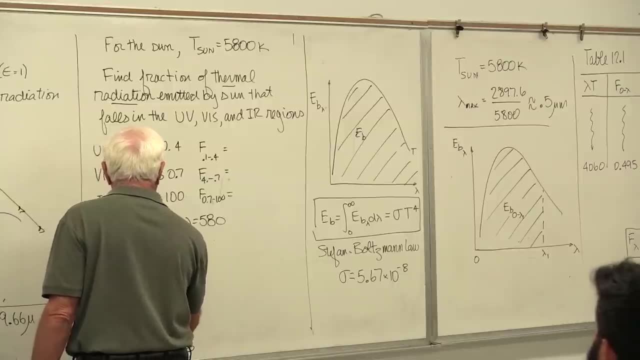 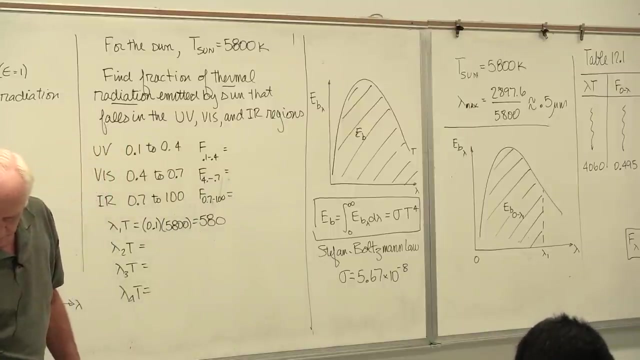 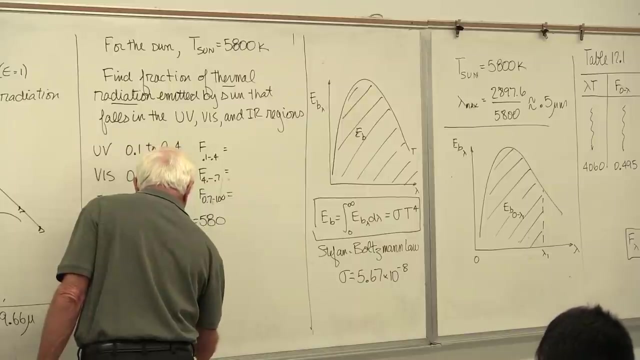 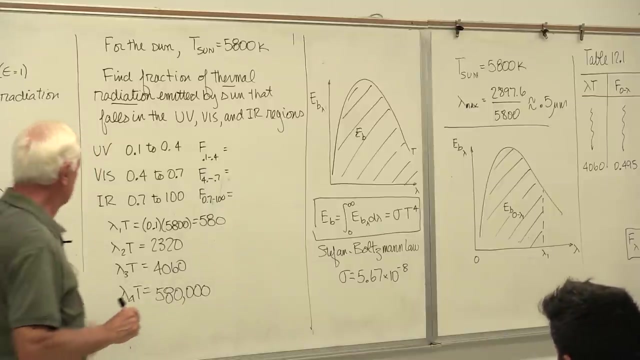 Times: 5,800.. 580.. 2t lambda, 3t. lambda 4t. Okay, let's see 2320.. 4060.. 580,000.. Got it Okay, There they are The lambda t's. 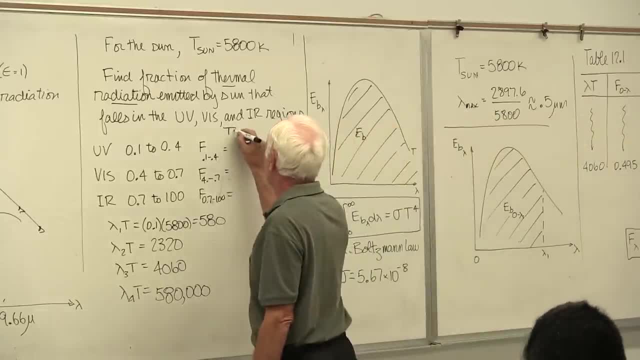 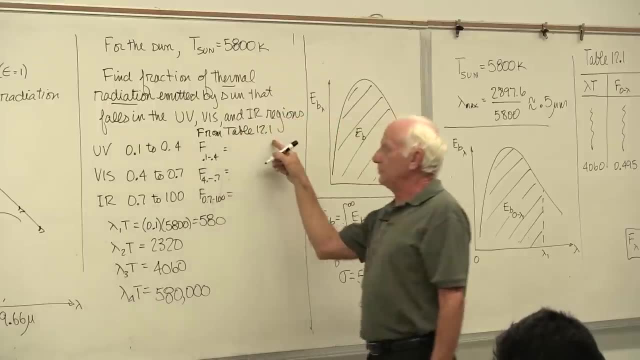 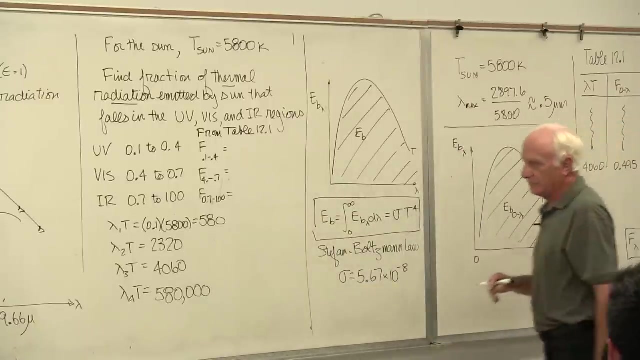 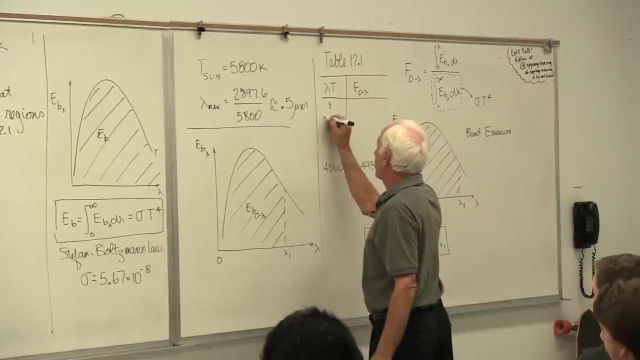 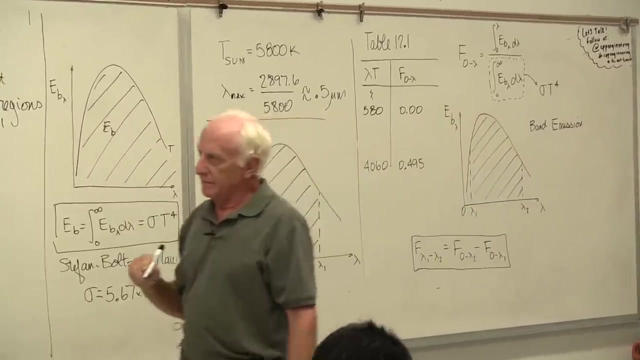 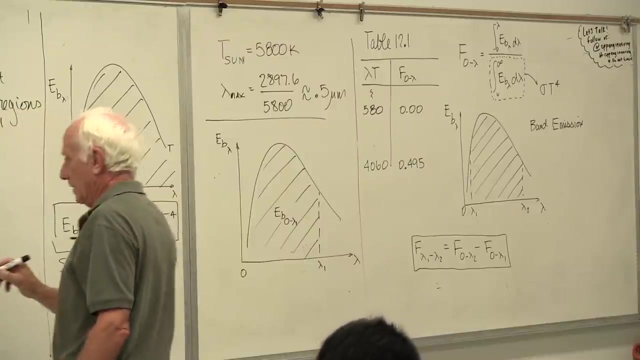 Go to table 12-1.. From table 12-1.. Go to the first lambda, t 580.. 0.00.. Fraction is 0.. From wavelength of 0 out to our 1 tenth 2320.. 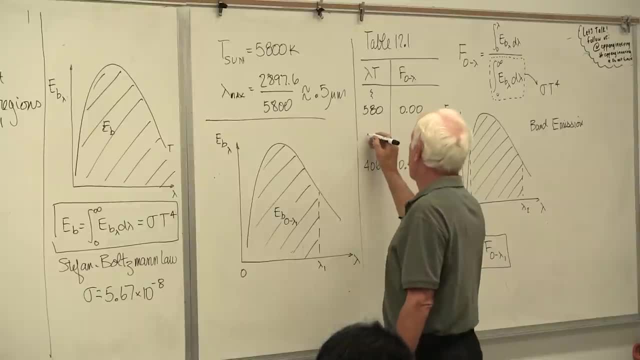 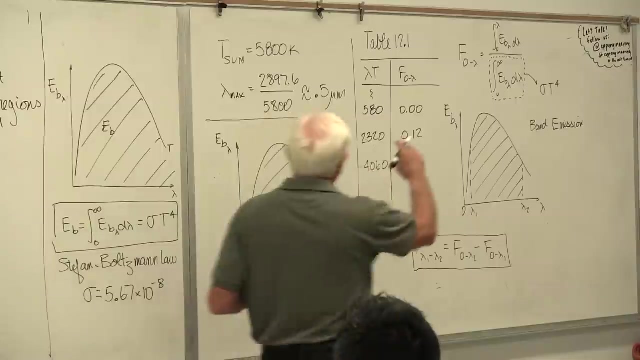 2320.. Fraction 0.12.. 0.12. 0.12. 0.12.. Fraction 0.8.. 580,000.. Go to Table 12-2.. 580,000.. 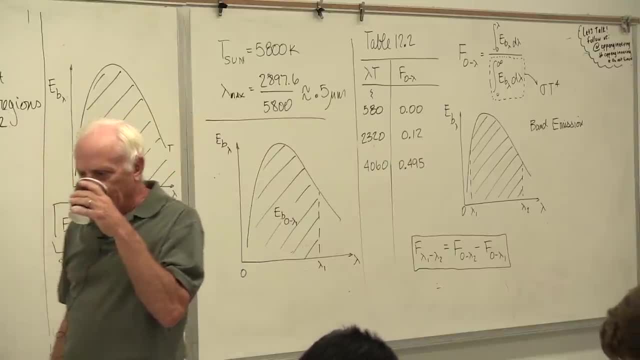 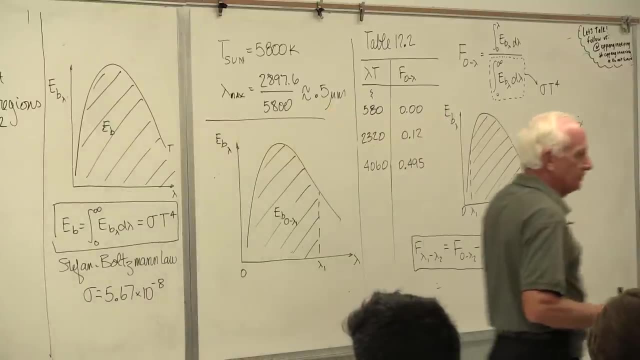 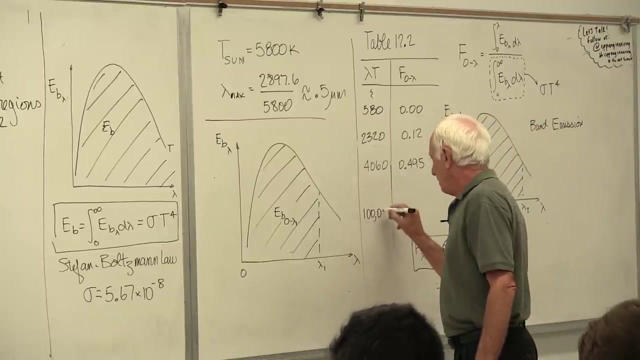 Go to Table 12-2.. You won't find it: 580,000.. It's not in the table. It's not in table 12.. There's no 580,000. But there is 100,000.. Yep, 100,000. 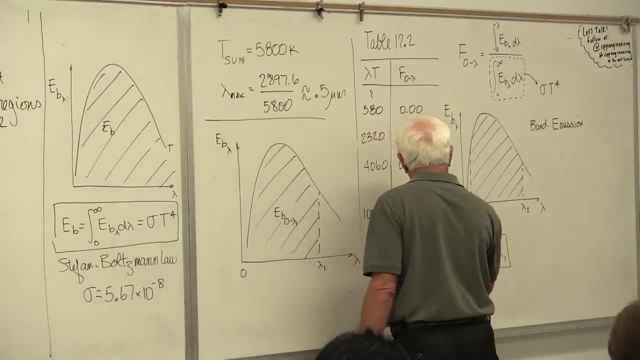 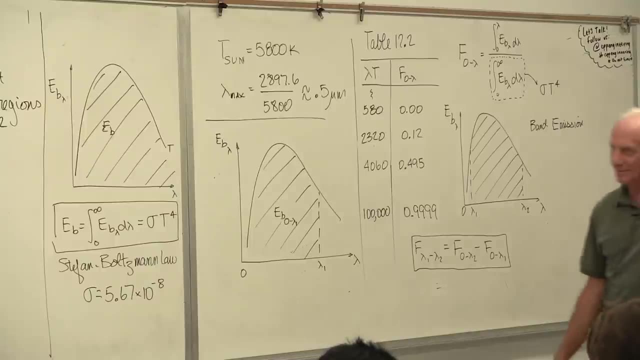 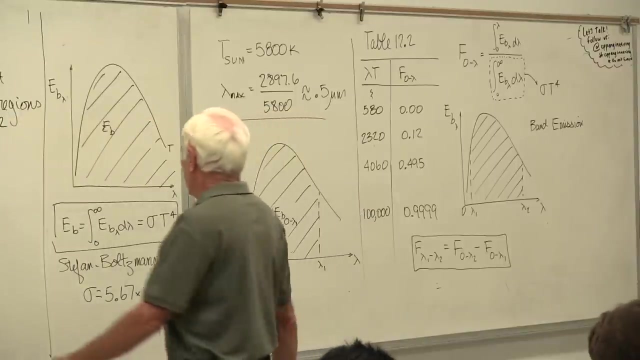 Good news. Four, nines in a row. So guess what? anything above 100,000 is Okay. The answer is 1.. The fraction here is 1.. Okay, We don't need this. So now we'll find these fractions. 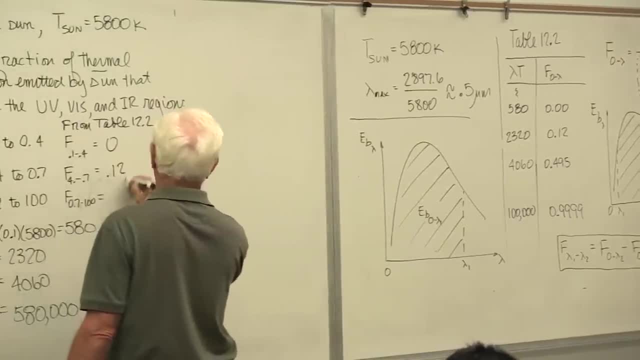 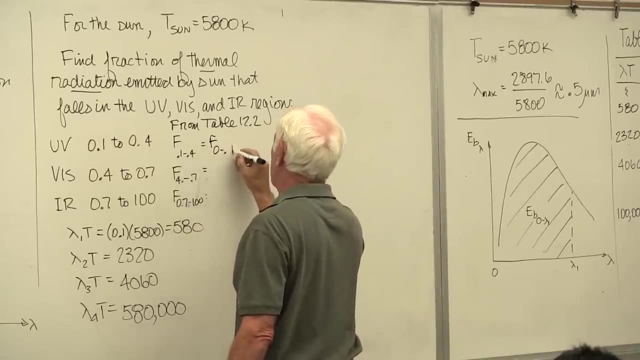 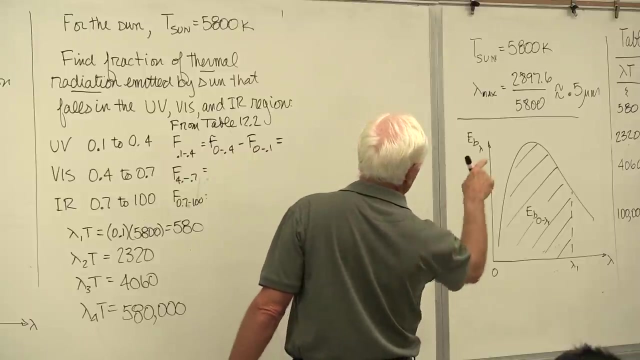 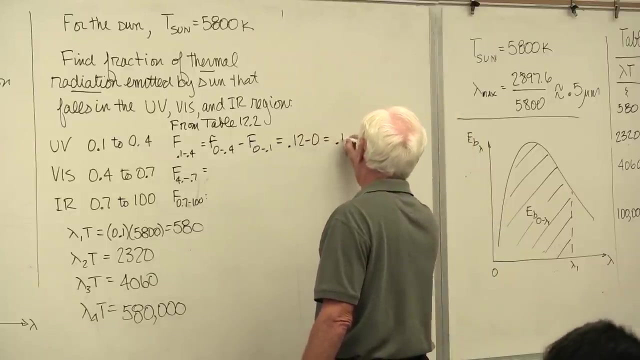 Okay, 0.1249. Oops, Not there, Pardon me. Fraction from 0 to 0.4, minus the fraction 0.1.. 0 to 0.4.. Our fraction was 0.12.. 12%. 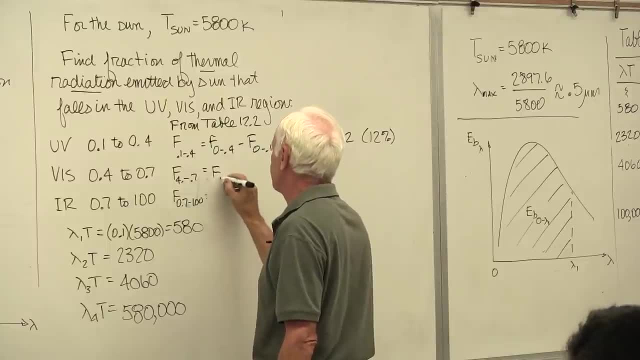 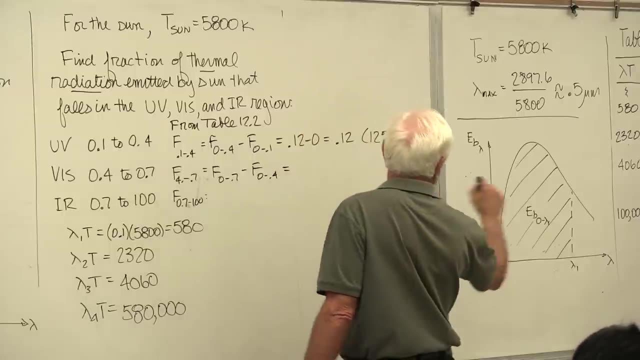 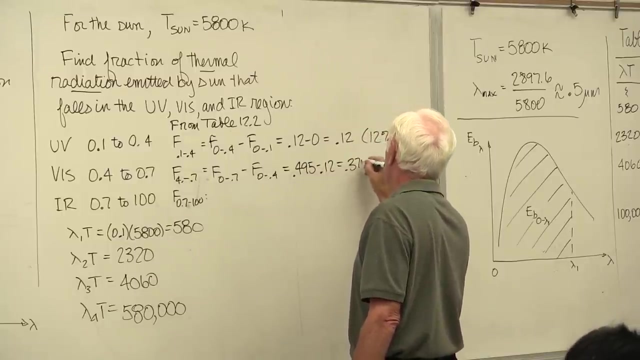 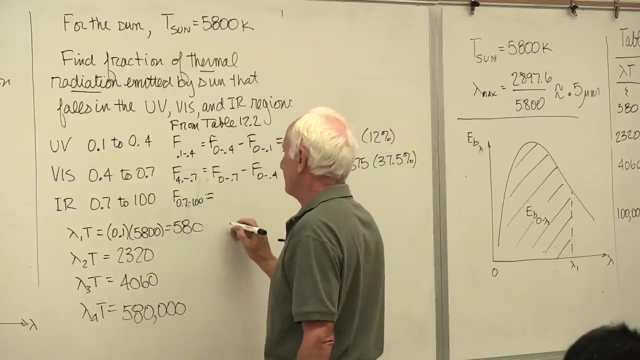 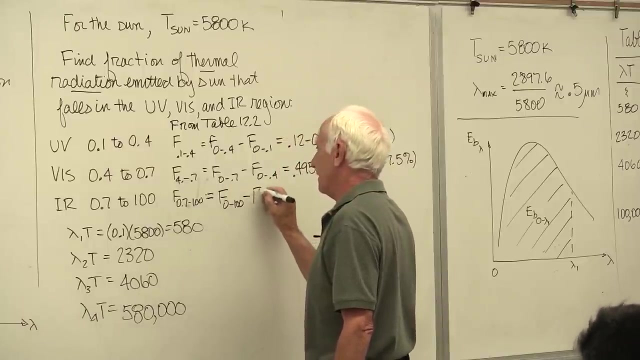 Fraction 4 tenths to 7 tenths: 4.95.. Minus .12.. 37.5%. Fraction 0.7 to 100.. 100.. Okay. Fraction 0 to 100.. Minus fraction 0 to .7.. 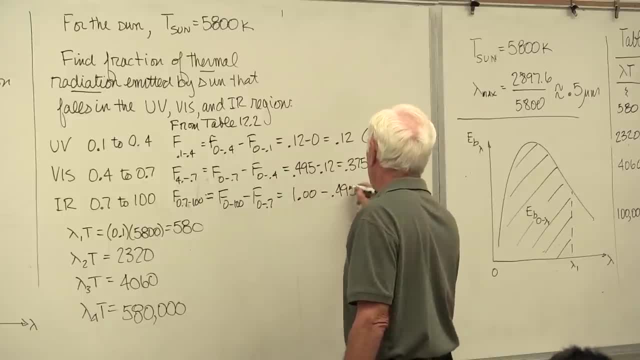 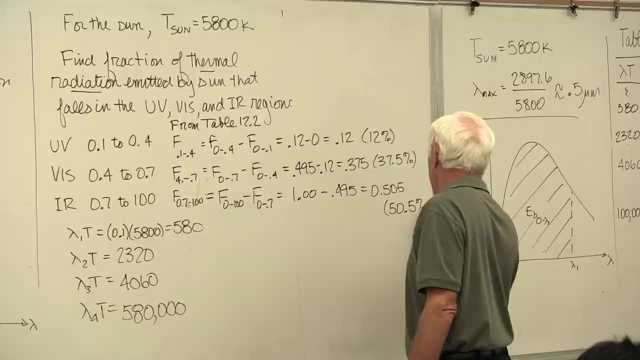 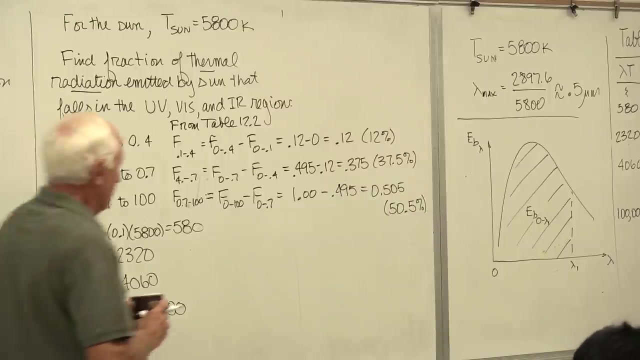 1.0 minus .495.. So of the sun's radiation, if you model the sun as a black body at 5,800 degrees, the biggest piece of it is in the ultra infrared region: 50.5% of the sun's energy in the thermal. radiation region is: in the infrared, 12% in the ultraviolet, 37.5% in our visible spectrum. so our eyes are only sensitive to 37% of the energy emitted by the sun in the thermal radiation band, Not the majority, no, 37.5%. 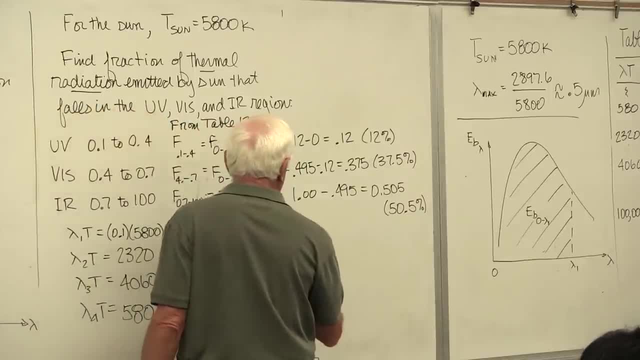 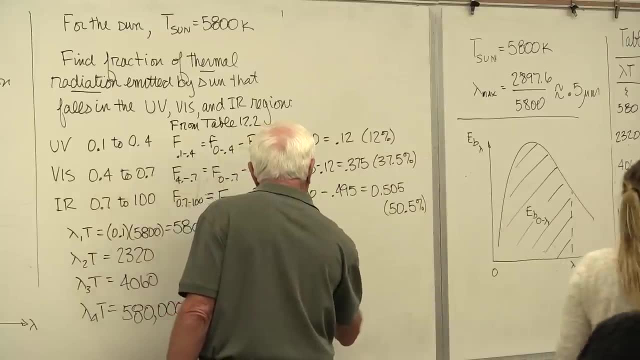 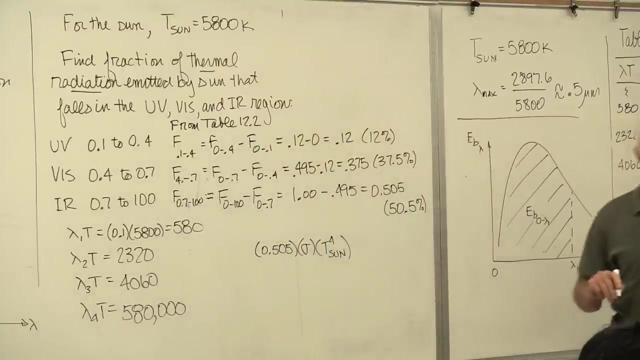 If you want to find an actual number, then you can take the 50.5,, 0.505,, multiply it by sigma t, sun to the fourth, And that tells me how many watts per square meter leaves the sun's surface. Okay, 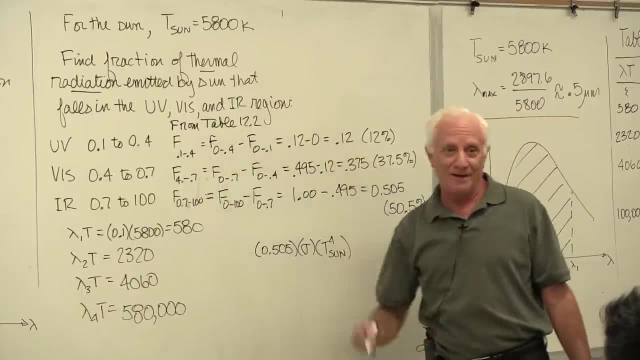 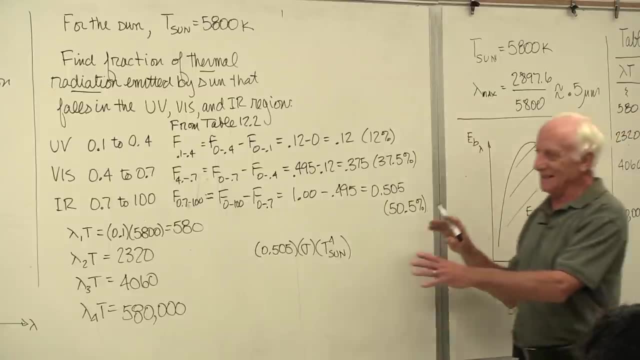 Raise that sun's temperature to the fourth power. Wow, is it big? How? about 5,800 raised to the fourth power? Yeah, that's a big number, a big number. That's how much energy is contained in the infrared region emitted by the sun. 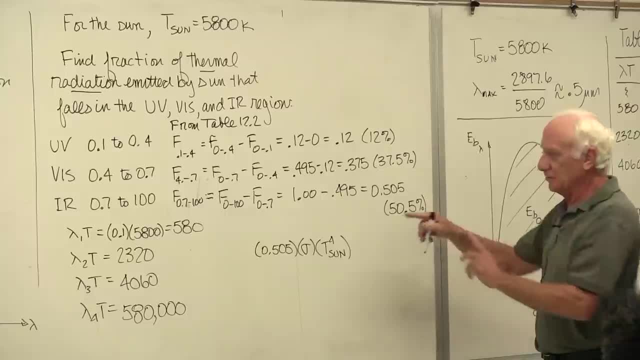 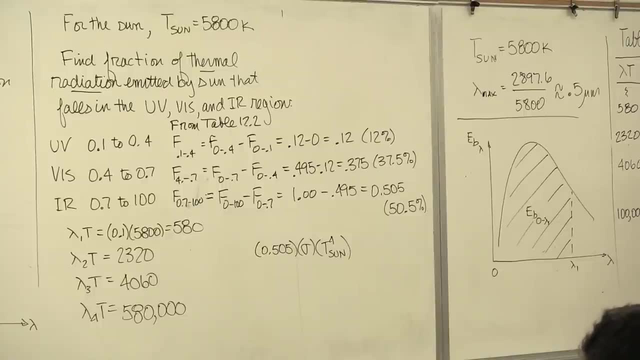 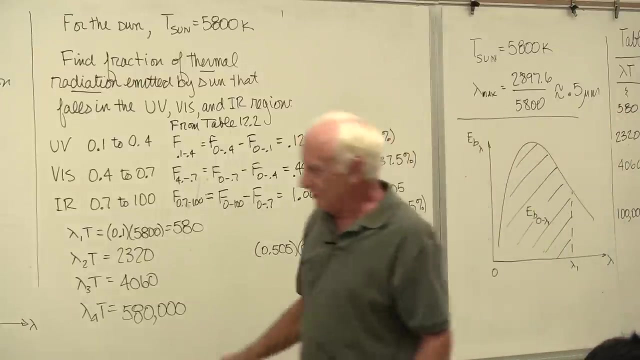 You take the fraction and you multiply it by sigma t to the fourth. Okay, So that's where it is right here. That's where it comes from, right here. Take the fraction, multiply it by sigma t to the fourth. Okay, so that takes into account how you use table 12-2 to solve band emission problems. 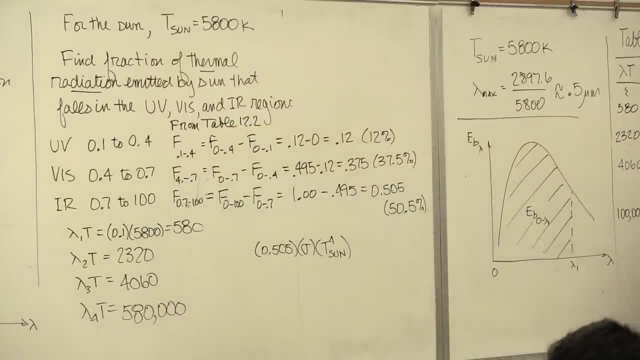 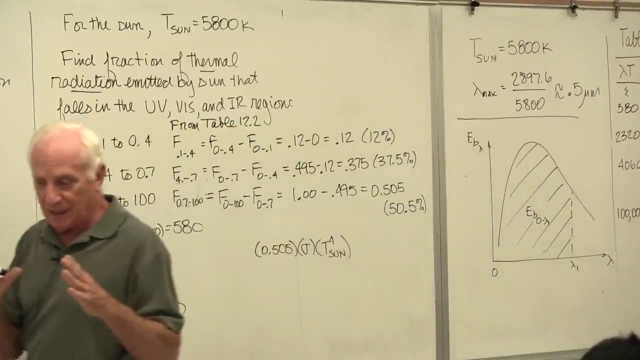 Band emission becomes important sometimes if you're dealing just as one, for instance, if you're dealing with solar cells. solar cells only respond to a part of the solar spectrum And it's important to know what that is so you can find out what the output of the solar 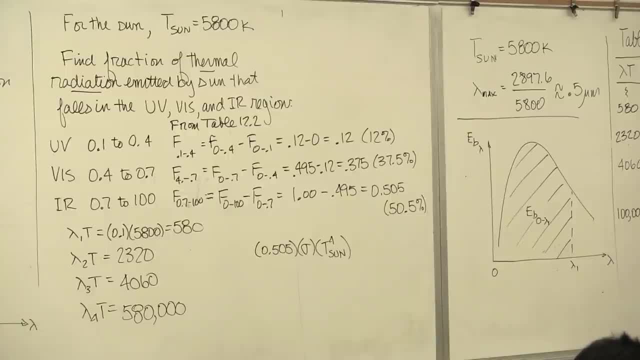 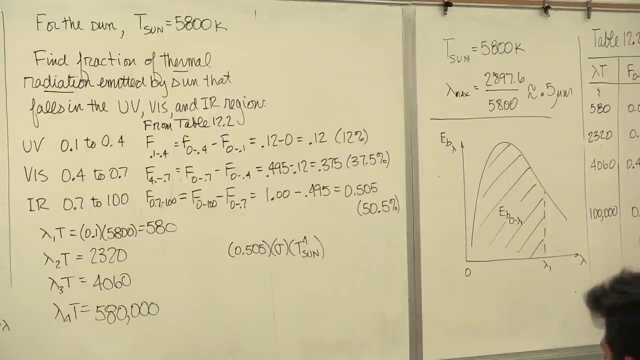 cells is So you? first of all, it's band emission. They only operate between certain wavelengths, lambda 1 and lambda 2. And from the sun, there it is, Find out the fraction, and so on and so forth. Okay, let's take a look then at, by the way, if you ever get confused in this material. 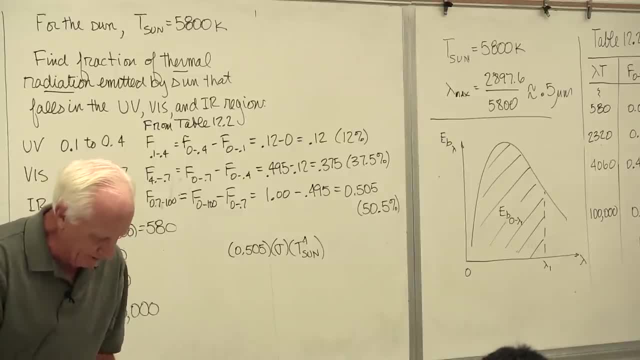 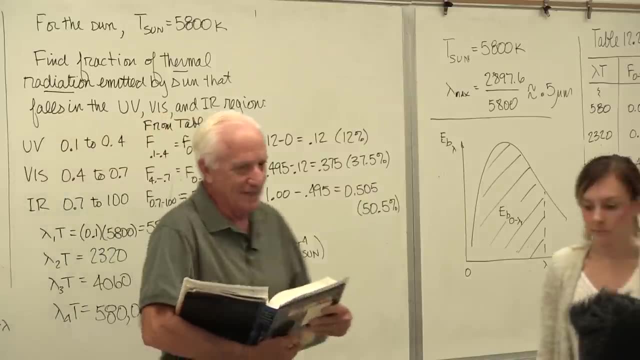 chapter 12, I'll say it is probably, without doubt, the most difficult chapter in all of heat transfer to understand and comprehend. It is It's very difficult to read. It's very important to take good class notes because if you try and read this, it requires. 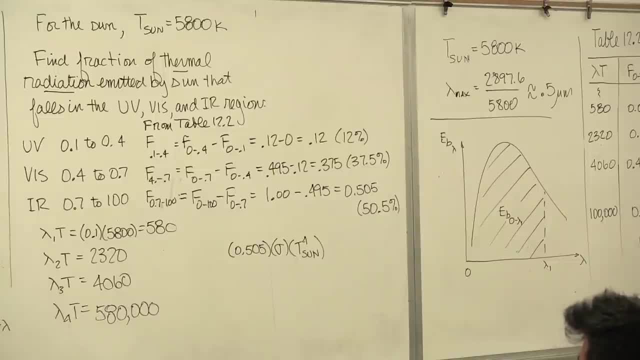 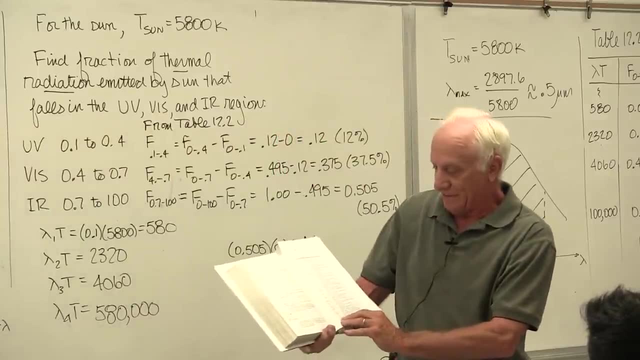 a lot of concentration, a lot of concentration. If you ever get confused about what words mean, go to table 12-4 at the back of the chapter. There are 24 definitions of words, 24 definitions of what the words mean. 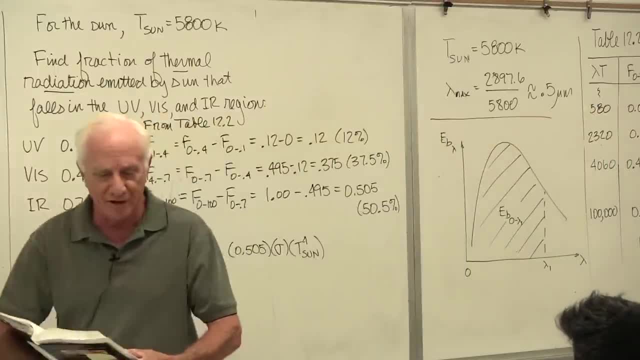 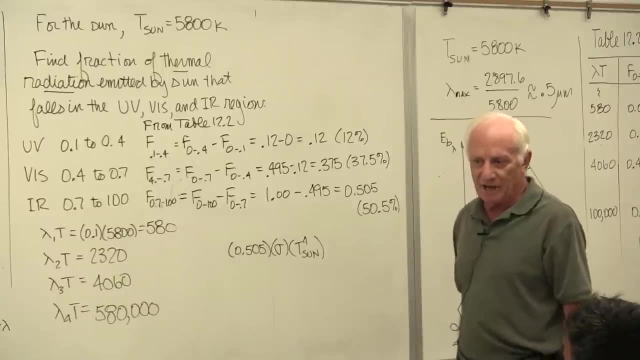 What does the word spectral mean? What does the word diffuse mean? What does the word gray surface mean? Oh yeah, irradiation, radiosity. it goes on and on and on and on. Yeah, it's a language. You have to learn the language of radiation first before I can talk to you. 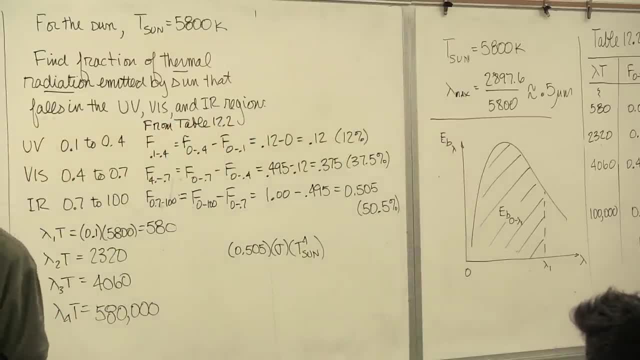 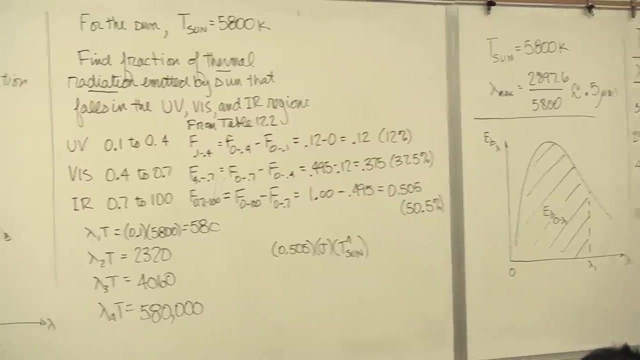 Otherwise it doesn't make any sense to you. You have to learn the language. Okay, let's talk about when radiation strikes the surface, what can happen to it. I'll put that over here. So we have an incoming beam of radiation hitting a surface. 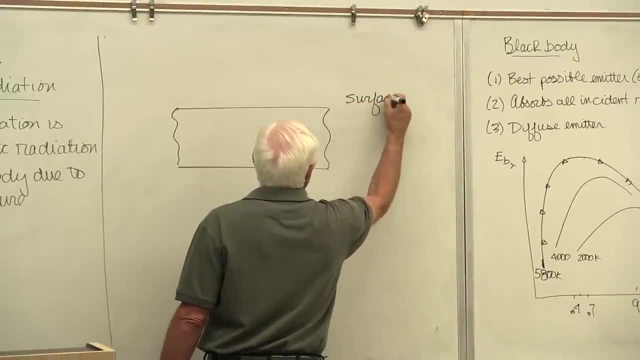 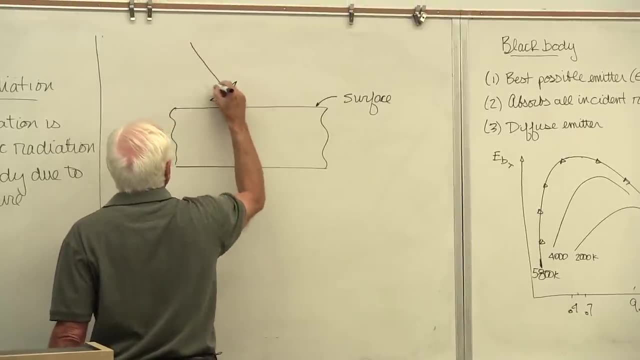 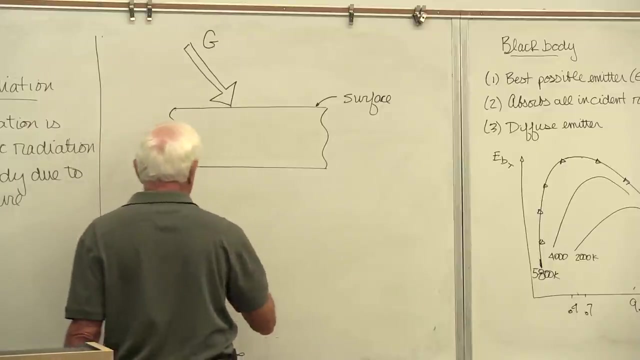 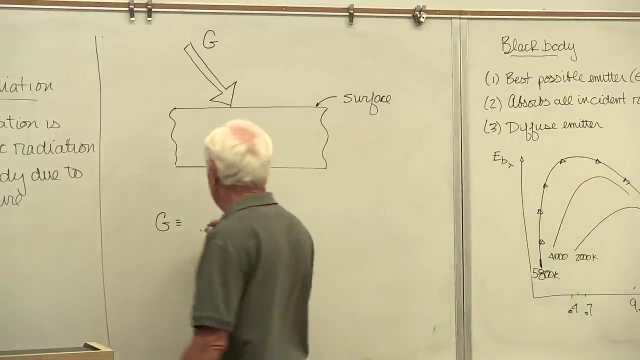 This is a surface, It's a thickness. right here, Radiation comes in, it strikes the surface, It's called G, G is called the irradiation And we can give it. we'll just call it the incoming radiation, Our incident, the incident radiation. 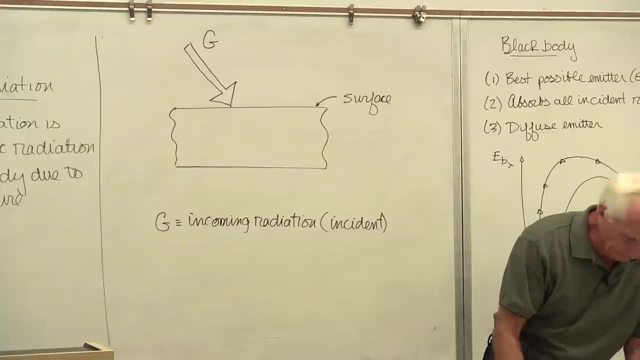 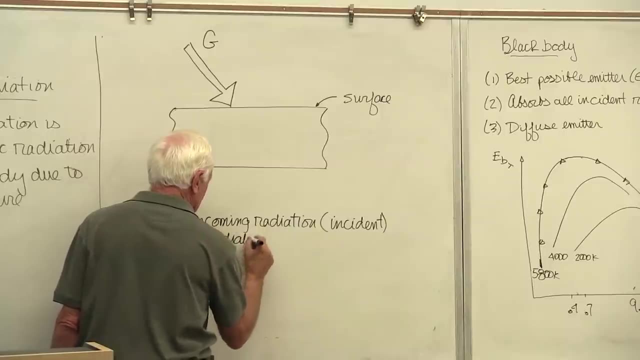 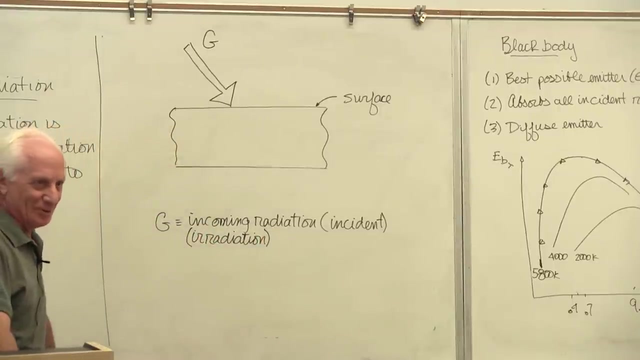 So we have this incoming beam of radiation. There's another word, I'll put them all on here: Irradiation. So if you see any one of those words, whether it be incoming radiation, incident radiation or the irradiation, that's G. 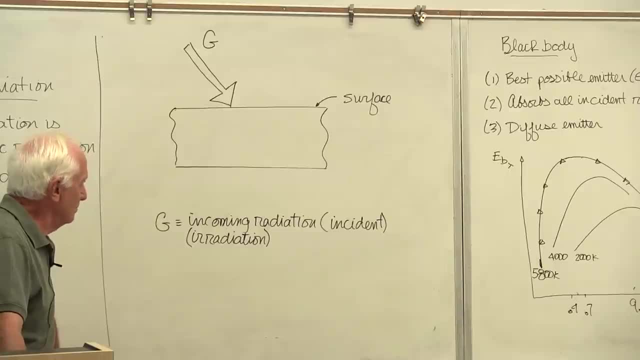 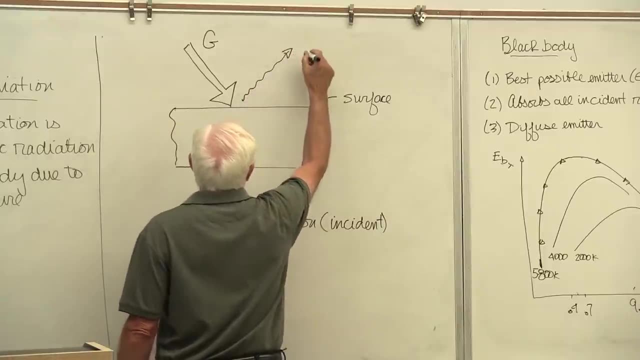 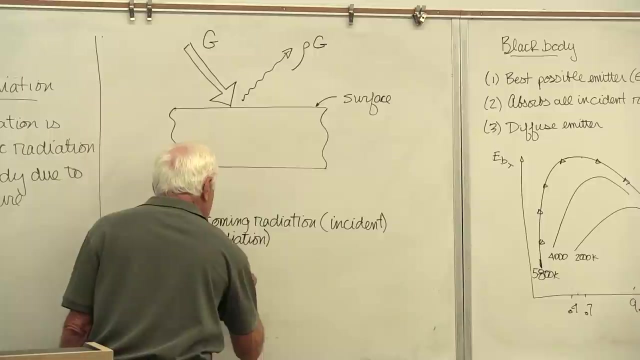 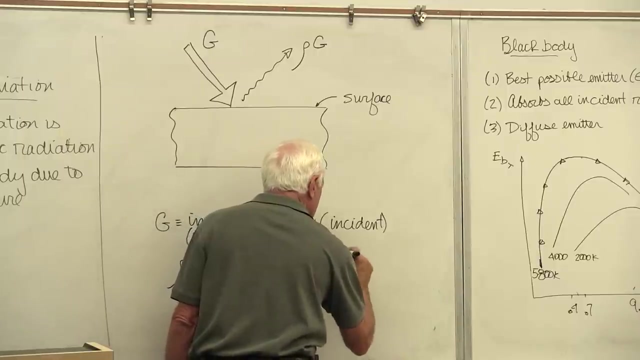 That's what comes into the surface. Once it comes into the surface, it can do several things. Number one is it can be reflected. Reflected is rho, Rho is the reflectivity. So rho G is reflected energy, Rho is the reflectivity. 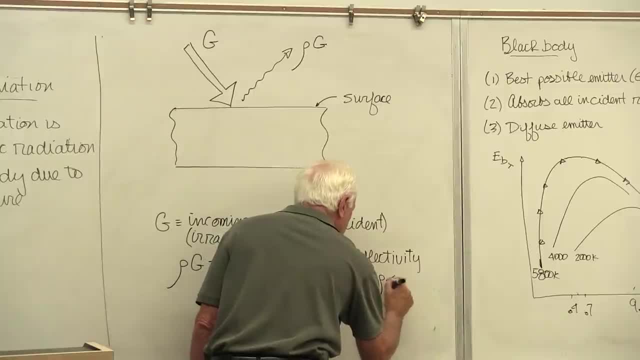 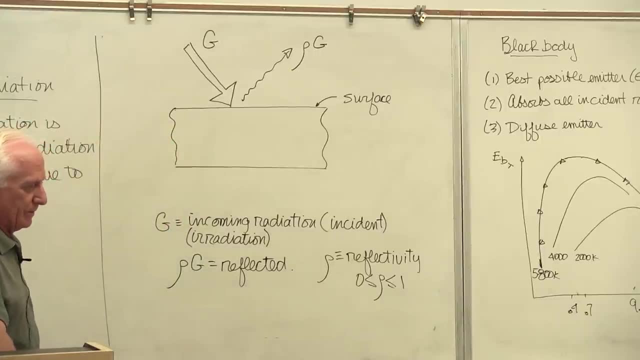 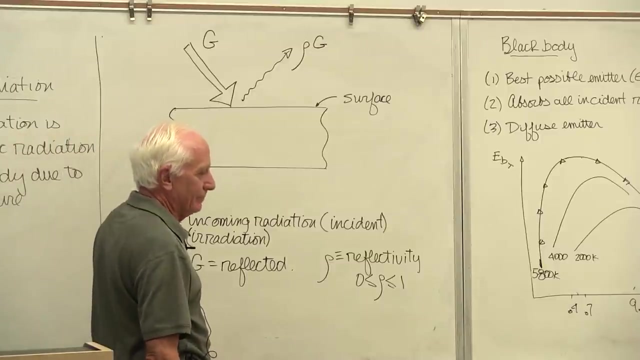 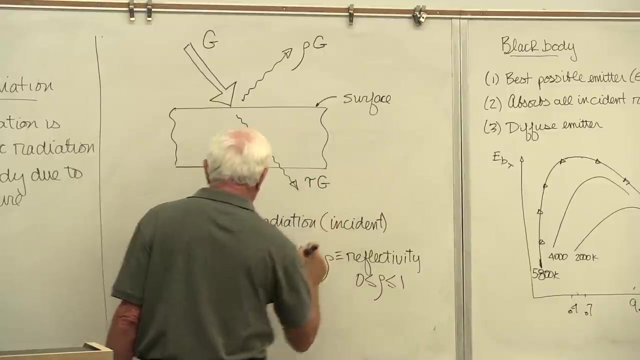 Its values. it's dimensionless. Its values are between zero and one. One means everything is reflected off the surface. Zero means nothing is reflected off the surface. Okay, Some radiation can just go through the surface And the result of that is a curve with a spin. 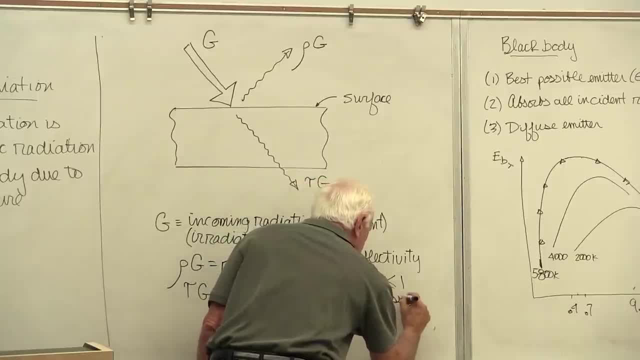 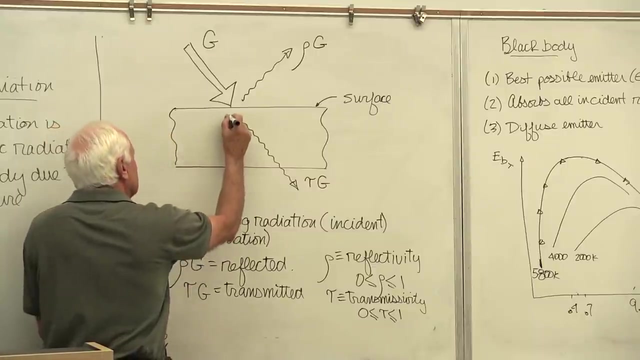 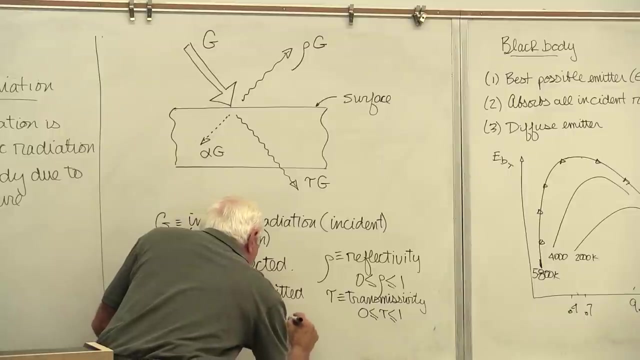 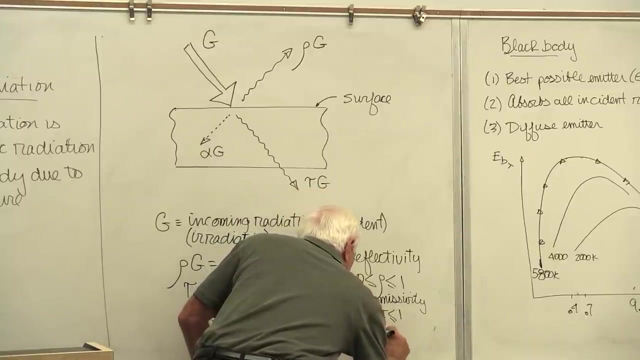 So it's Üb. U is transmitted. μ times G, So γ is transmitted, and 1.. Finally, some radiation can be absorbed in the surface: alpha times g. And alpha is dimensionless absorptivity. Its value can be between 0 and 1.. 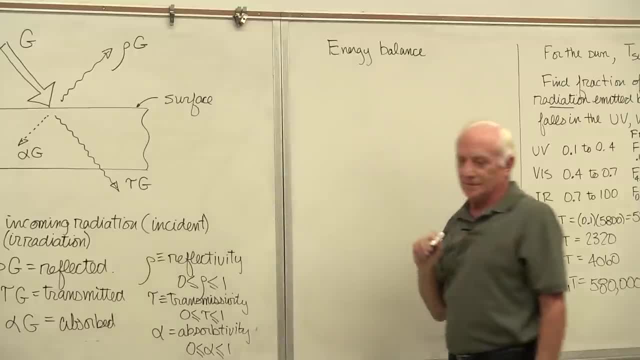 When the incident, energy comes in, where can it go? Well, the energy distribution is: what comes in is g. Again, you've got to watch these symbols. What does capital E mean? Emissive power- how much it emits. What's capital G mean? The incident or irradiation- how much comes into a surface. 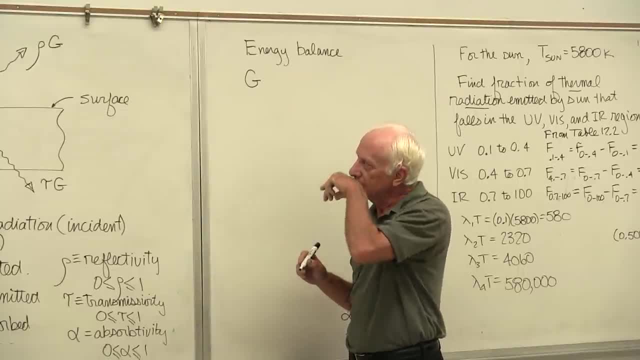 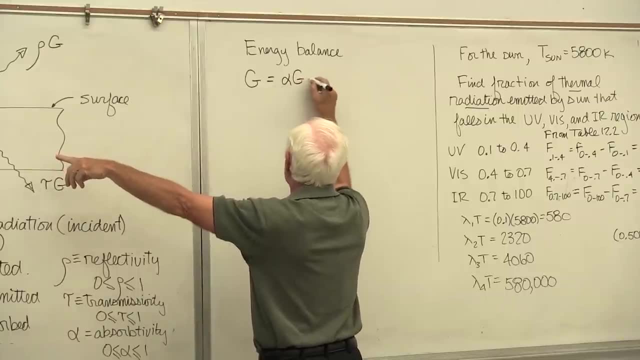 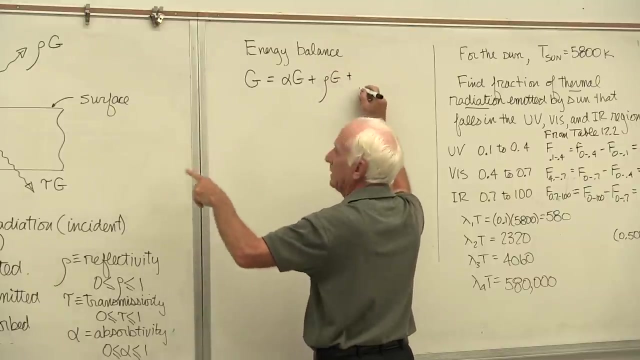 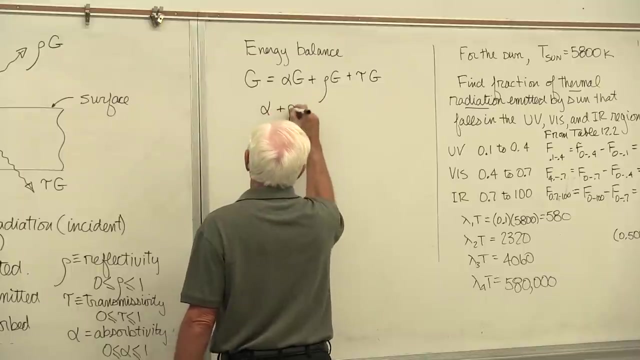 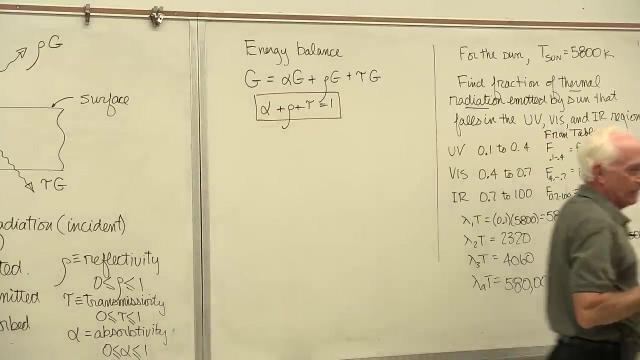 G comes into a surface, Capital E goes out of a surface. Where does that energy go? Well, number one: it might be absorbed. Number two: it might be reflected. Number three: it might be transmitted. Divide through by g. When you add those three properties together, you get 1.. 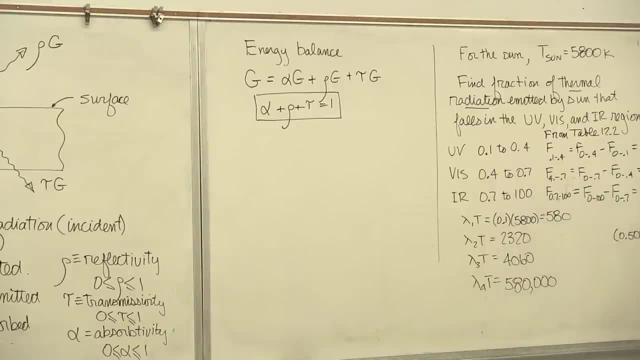 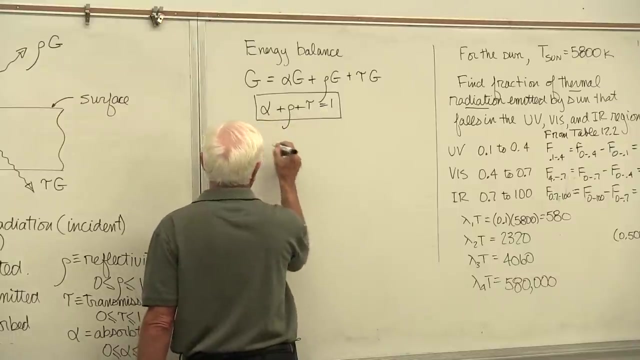 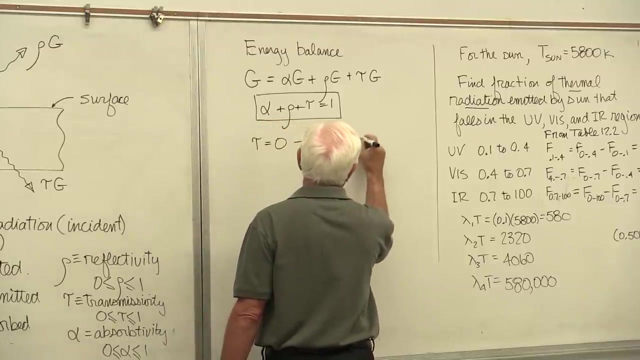 When you add them together, you get 1.. If I know two, I can calculate three. If I know two properties, I can calculate the third. Okay, Let's talk a little bit about Tau. Tau equals zero Opaque surface. Opaque surface means nothing gets through. 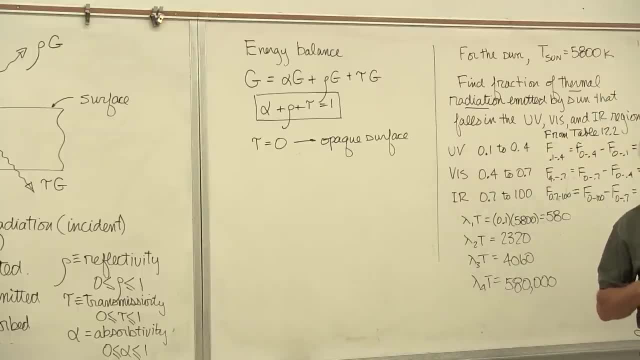 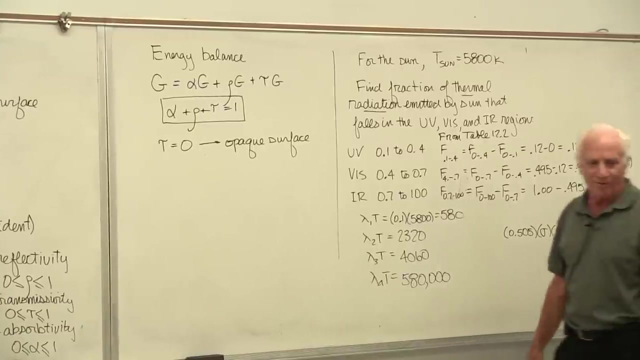 Concrete wall here With my eyes. I can't see anything in the hall. I can't even see fuzzy figures of people out in the halls. Is that a person I see there? No, no, I can't see a thing. Conclusion: I can't see a thing through that wall. That must mean tau is zero. 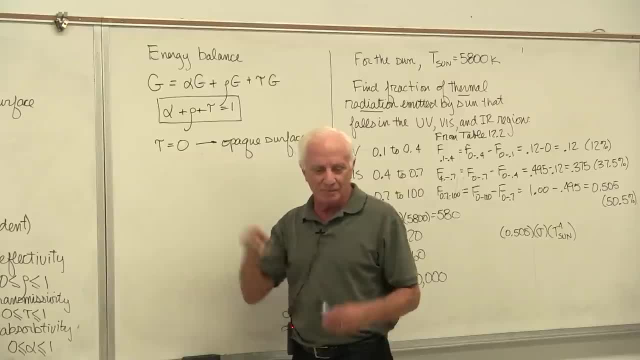 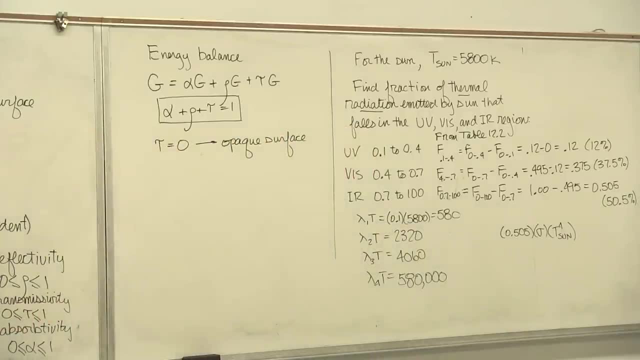 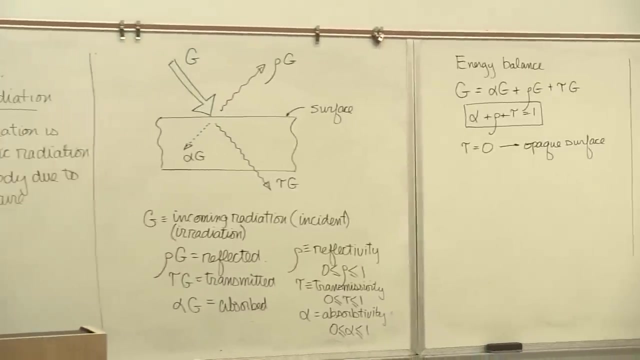 No radiation in the visible part of the spectrum came through that wall. to my eyes, That's just the visible spectrum. Okay, This over here is a solid surface. It's called glass. The purpose of glass is to let light through. We want natural light in the room to help. 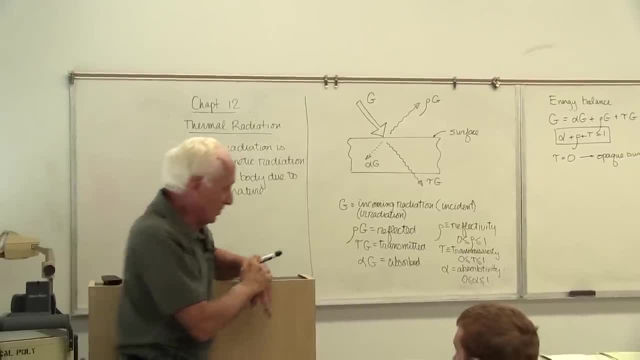 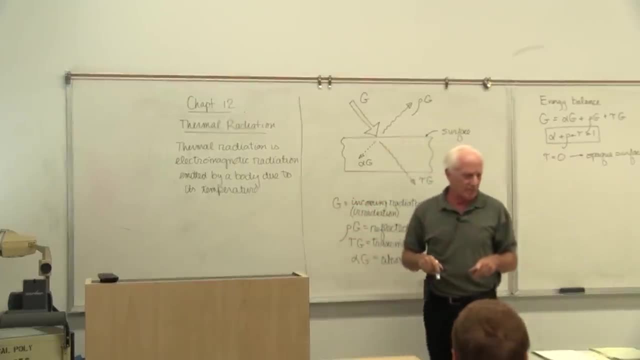 with the lighting situation. What do I want? An opaque surface? Of course not. That wall is opaque, That glass. I want to have a high transmissivity. I want sunlight to come through there. So I want a high value of tau, Over 90%, hopefully. 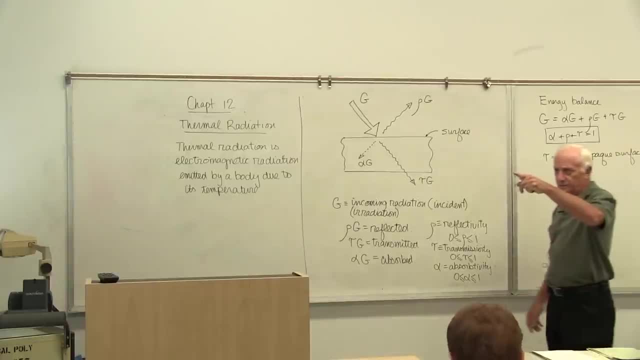 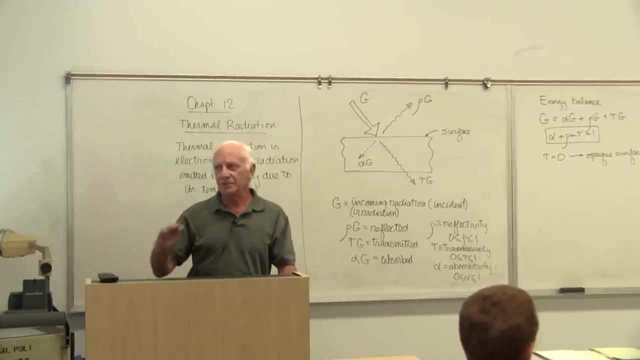 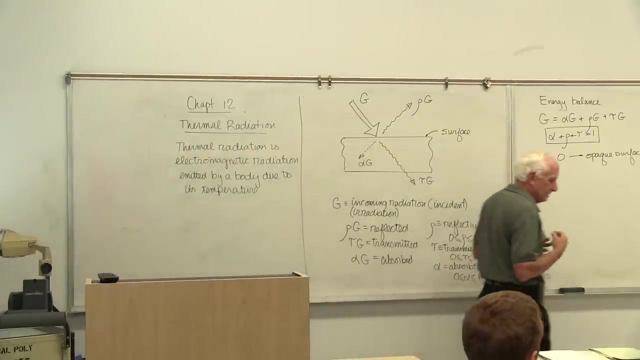 When the sun strikes. that and, by the way, not just the direct sun. There's no direct sun on that glass right now. That's all reflected solar energy. That reflected solar energy has the same wavelength distribution as the sun. It's being reflected. Okay, so that's. 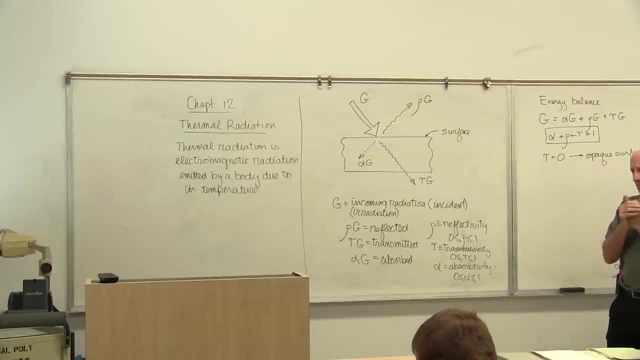 what's coming through the window is reflected sunlight. It has the same wavelength distribution. Is there any reflection? Oh yeah, There's reflection off glass. You can buy anti-reflective coatings for glass with what's called anti-reflective coatings to cut down on the reflection. but 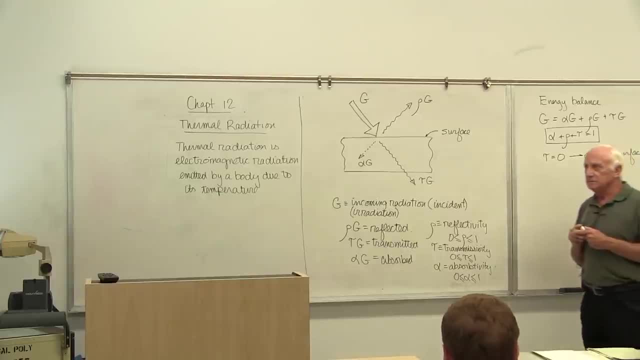 there is reflection off that glass from the outside. Sometimes on some solar collectors on roofs they're not reflecting that glass, But sometimes they're. Sometimes sometimes The neighbors complain because at certain angles of the sun- sunrise or sunset- they 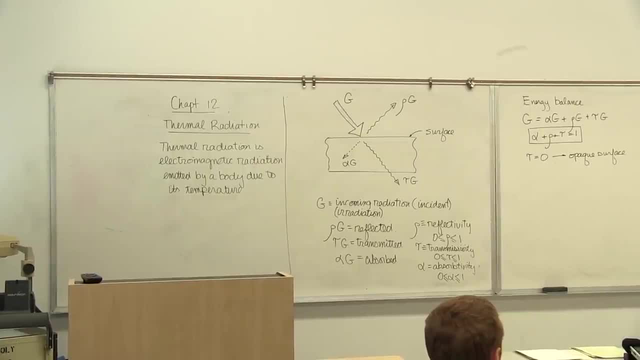 can get blind in their backyard because of the reflection off of those solar panels. So you want to cut down that reflection? So yeah, there is some reflection, Not a lot. This guy should be over 90%. That guy is a few percent. 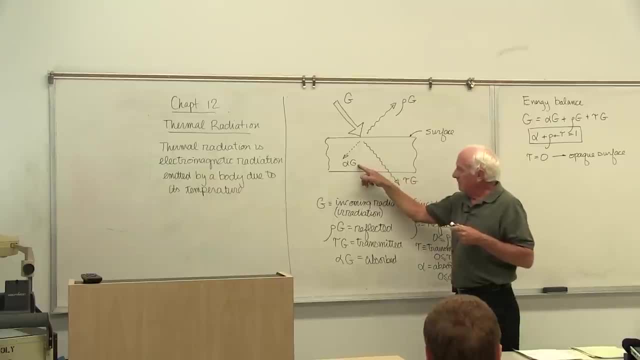 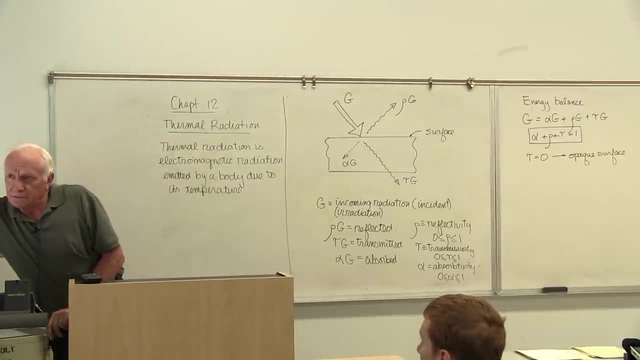 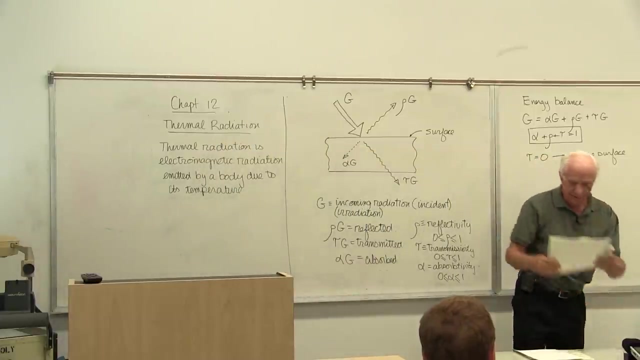 Say: yeah well, is anything being absorbed in that glass? Oh yeah, That's not expensive glass. There's iron in that glass, Iron in that glass, And if you hold that glass or sheath that glass up in here to the light, if you see. 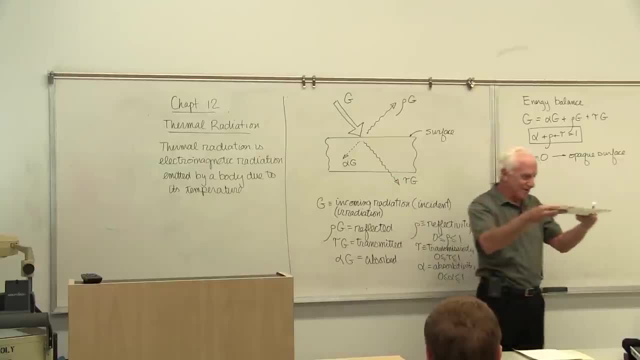 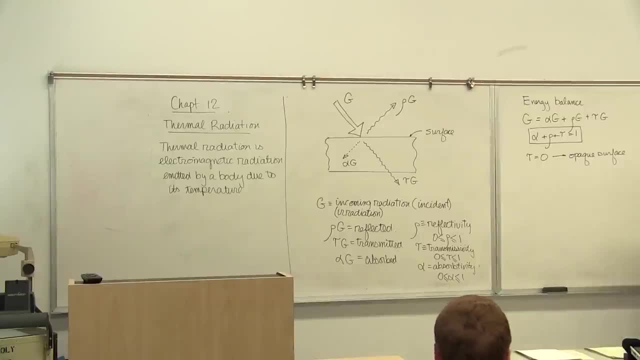 You're going to have to do a lot of things. You're going to have to do a lot of things. You can get glass with low alpha. You can buy low alpha glass. It costs more. Is it worth it? I don't know. 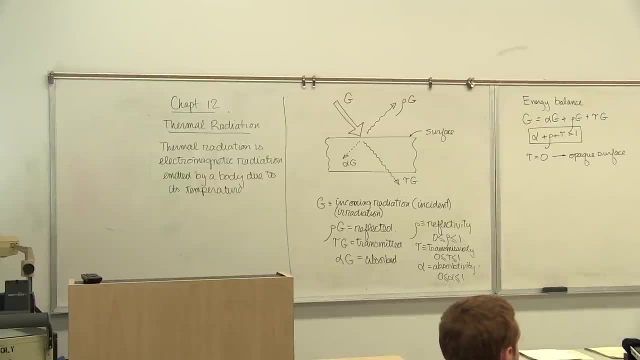 It would be economics. Is it better for a solar collector? technically? Oh yeah, It lets more sunlight through to hit the absorber plate, but it's going to cost you more for that special glass. The glass is called water white. 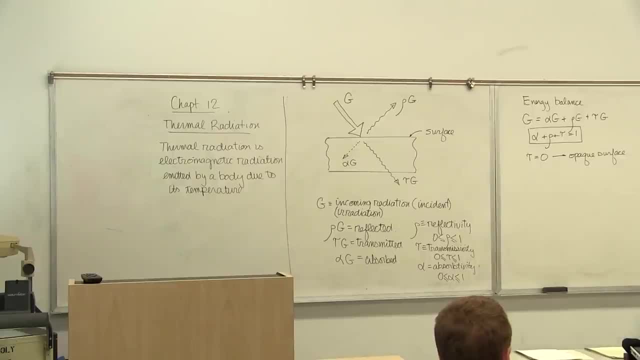 Water white. It's so white there's no green tinge to it. Hold on edge, look at it. There's no green tinge on the edge of the glass. Water white glass, Yeah, so it cuts down on that guy right there. 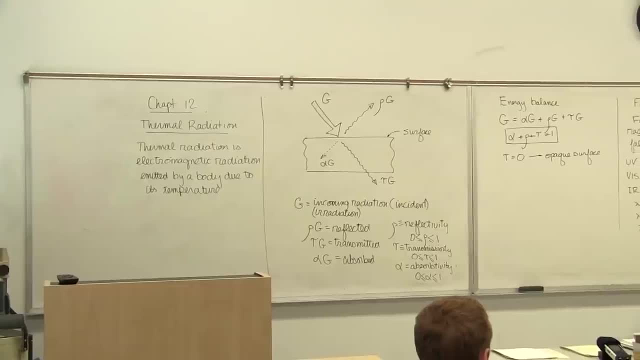 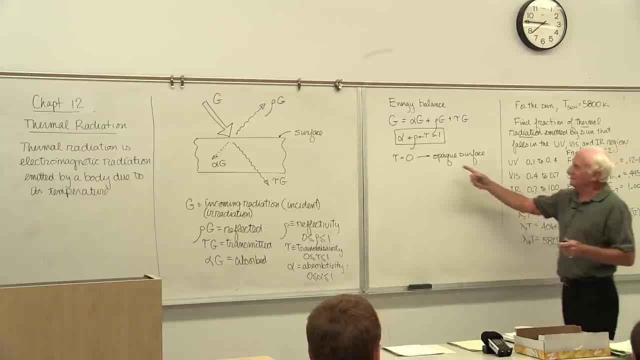 So that's what this gives you. It's called surface properties. Surface properties: There are three surface properties, okay, here in this equation: Alpha, rho and tau. If tau is zero, it's an opaque surface. Okay, so let's do one more. 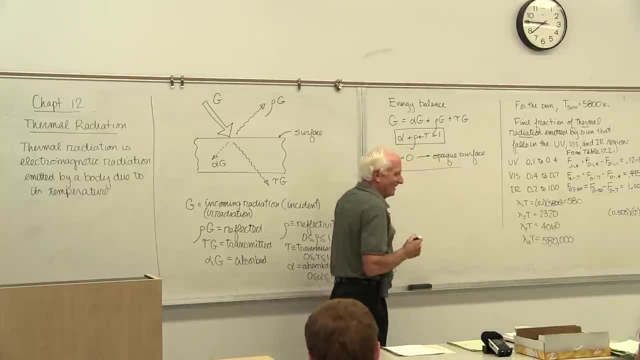 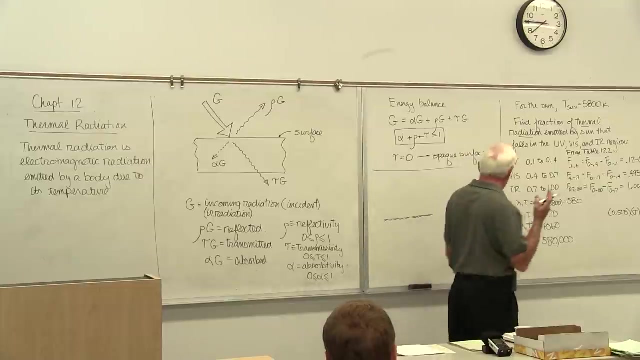 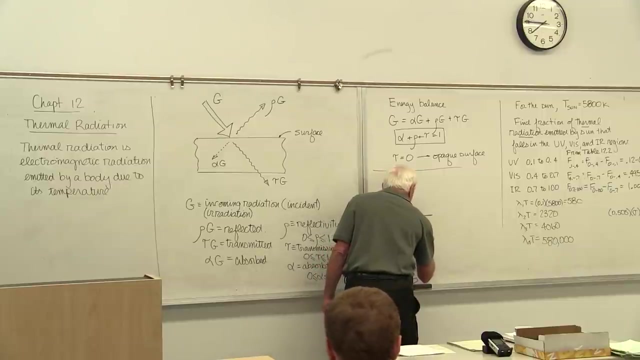 Let's look at when surface emits radiation. we had that black body, one, two and three. one, the best emitter. two, the best absorber, absorbs all energy. Three was a surface is diffuse. Okay, so what is a diffuse emitter? okay, diffuse emitter. 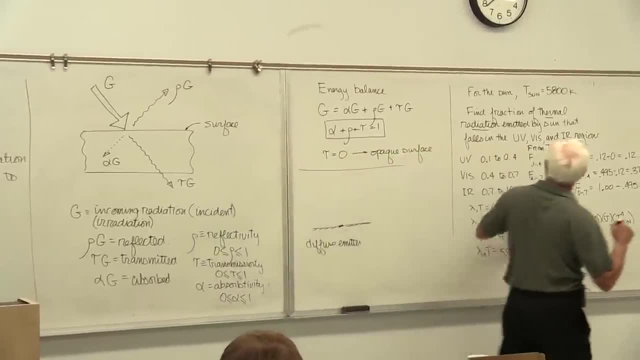 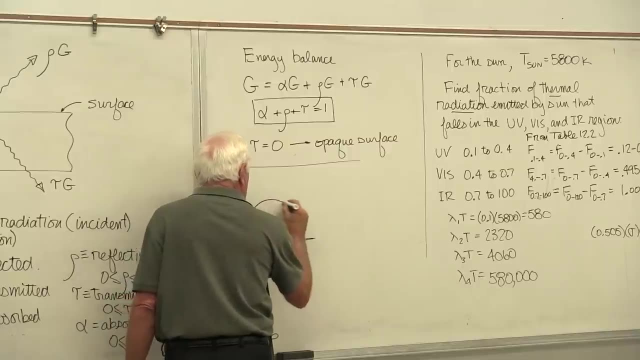 When it emits radiation like this stuff right here. okay, when it emits radiation. diffuse emitter means it emits equally in all directions. There's no preferred direction of emission. It's the same in all directions. above the surface, That's a diffuse emitter. 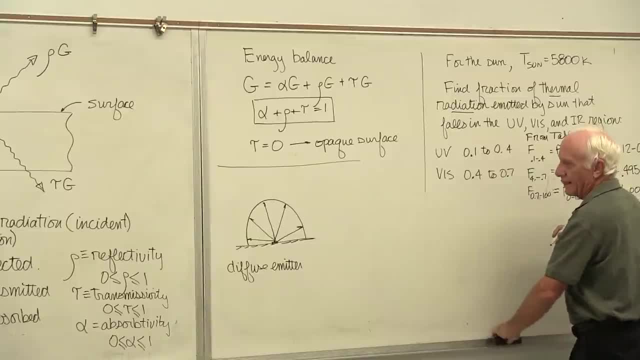 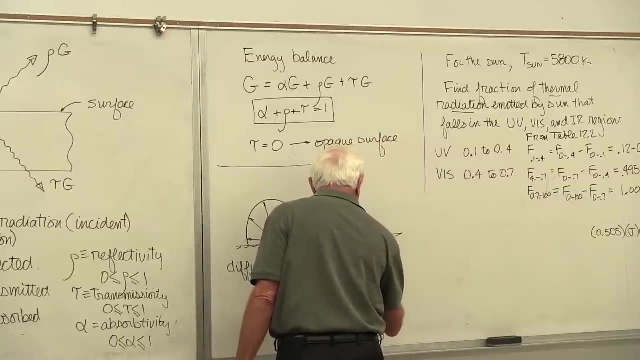 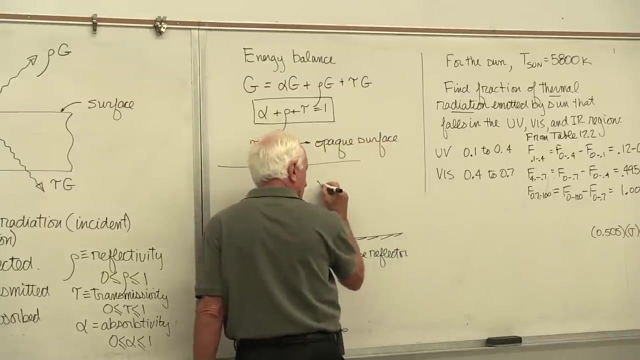 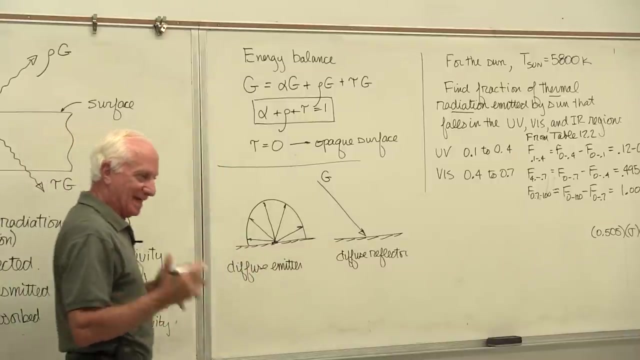 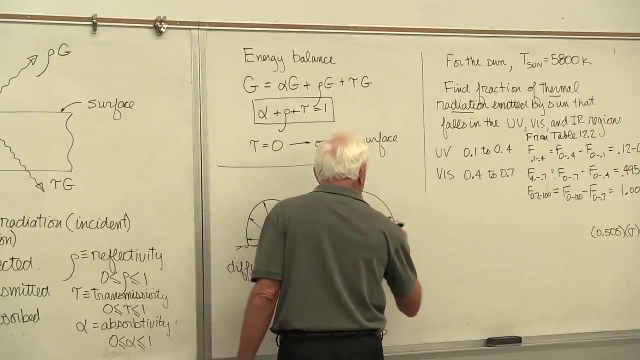 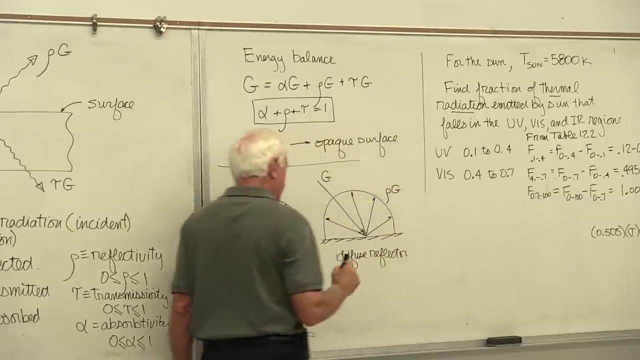 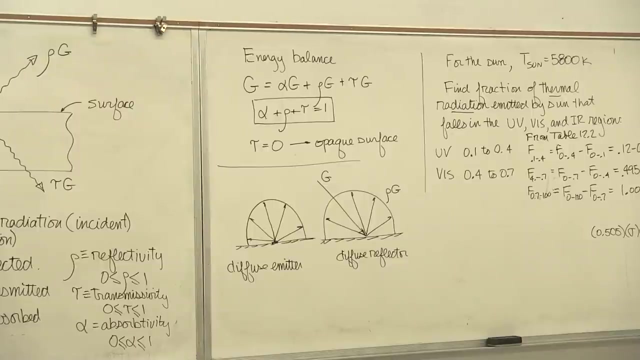 Now you can also have a diffuse reflector. Okay, So in comes the radiation beam G and then, when it's reflected, looks like this: It has no preferential direction. rho G, That's a diffuse reflector. Excuse me, what would be an example of a diffuse reflector? 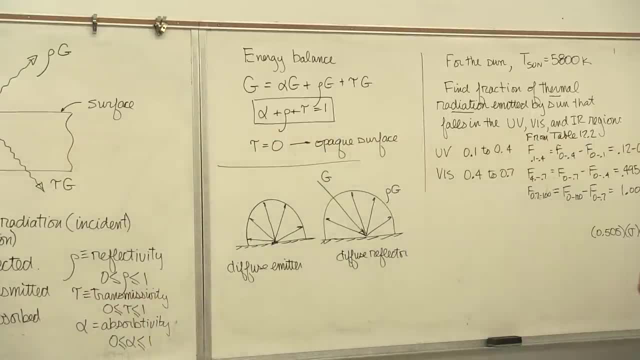 Yeah, yeah, I might have you hang on until when, is it? I'm not sure. let me think, if I I've got, yeah, I'm going to do examples, but I'm not sure I'm going to do it right now. rather, 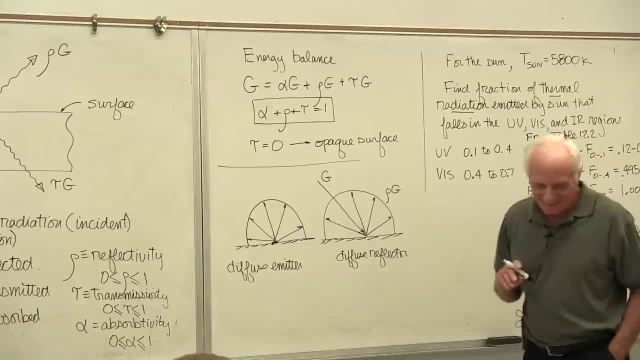 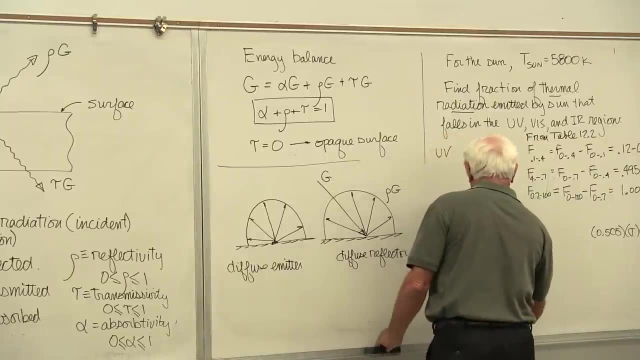 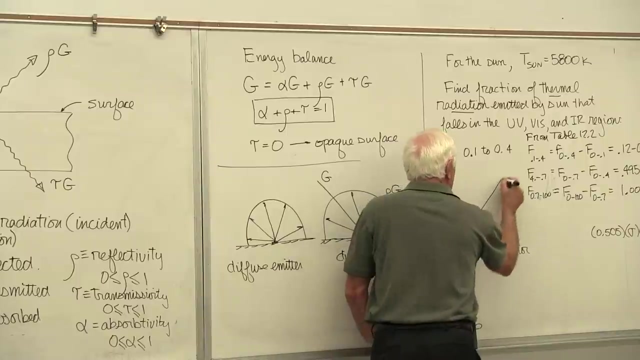 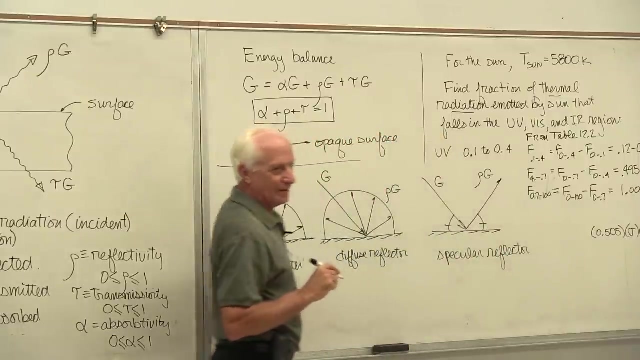 than when I do the next step. Yeah, I've got time, we'll do it. Okay, let's take this one. This is a specular reflector. Uh-oh, the angle of incidence equal the angle of reflection. That's specular. 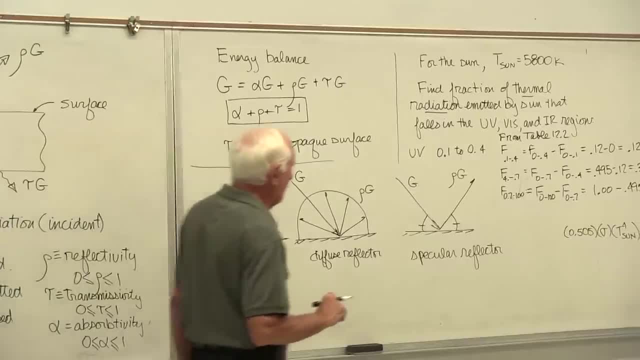 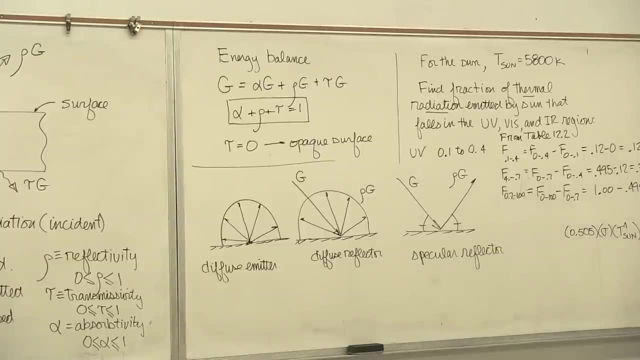 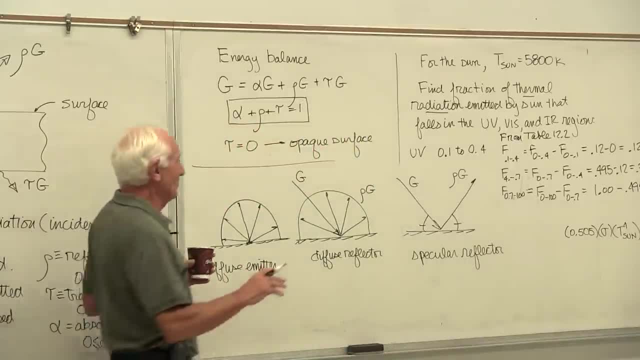 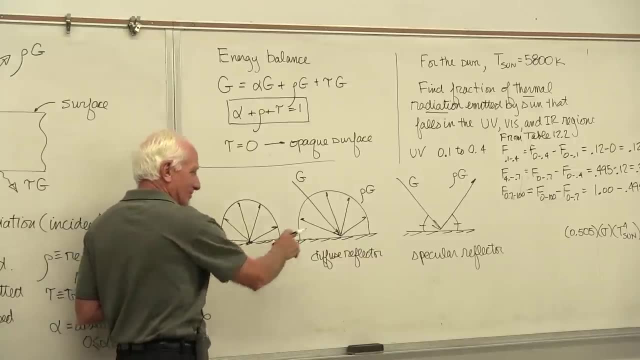 We don't in this book. in this course we don't look at these guys. In this course we'll only look at diffuse emitters of radiation. Okay, see emitters and reflectors, Because when you do this kind of here, it mathematics. 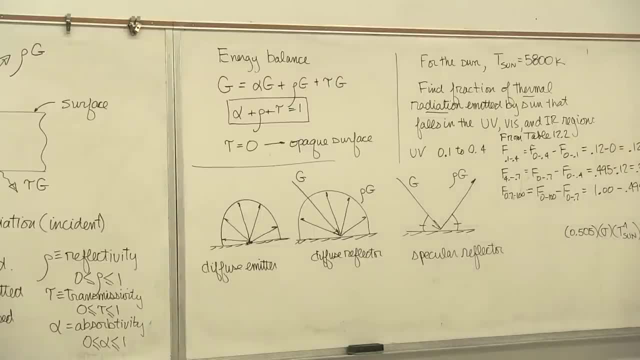 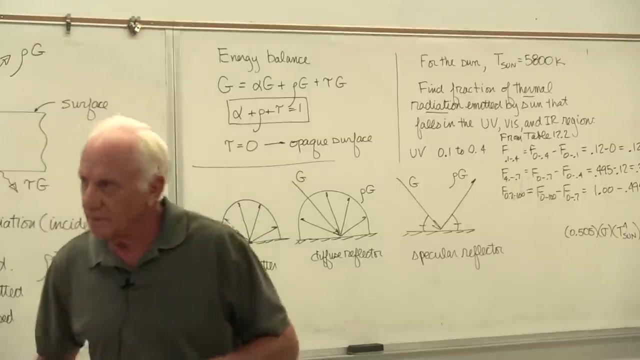 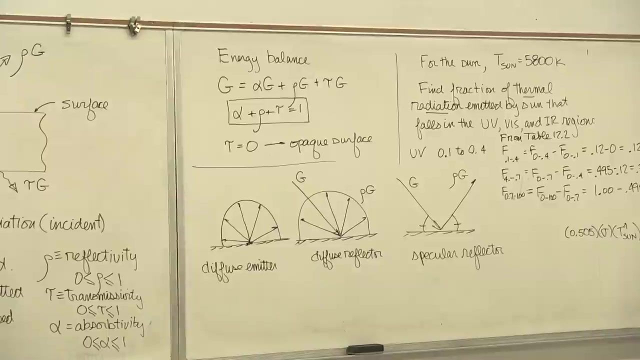 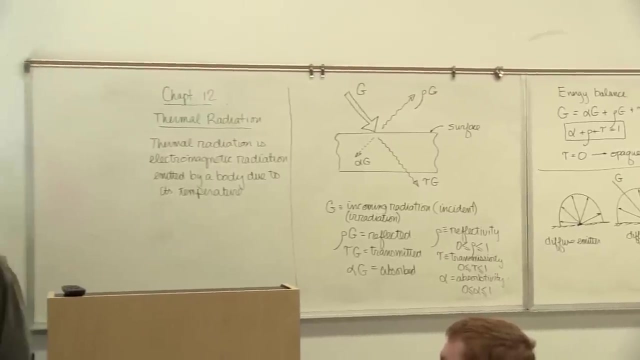 goes up dramatically. Save that for the graduate class. Specular reflective surface like mirrors. Here's clear glass. I can see right through it. I can see people walking. I can see trees, leaves. I look down here. I can't see people walking. I see nobody out here. Oh, I see. 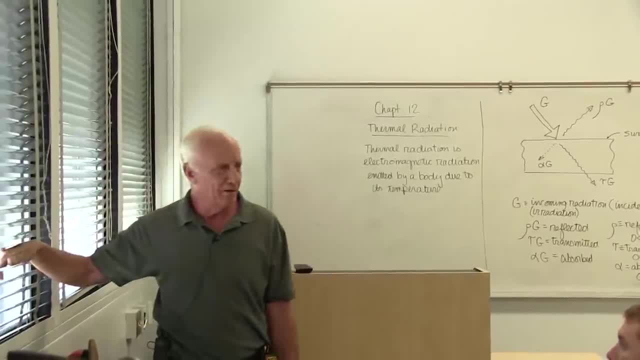 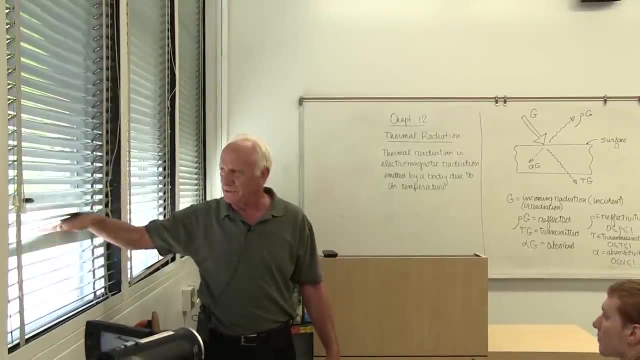 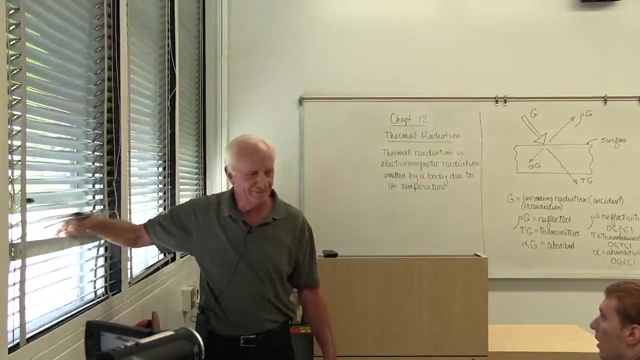 a white haze like fog. Why did they put that in the window? Why did they put that in building nine here, And that's glass up here and that's this. Listen to this glass, Listen to that glass. Oh yeah, there's a difference. That glass. 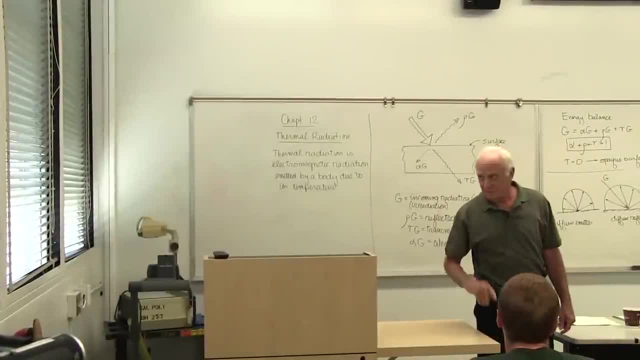 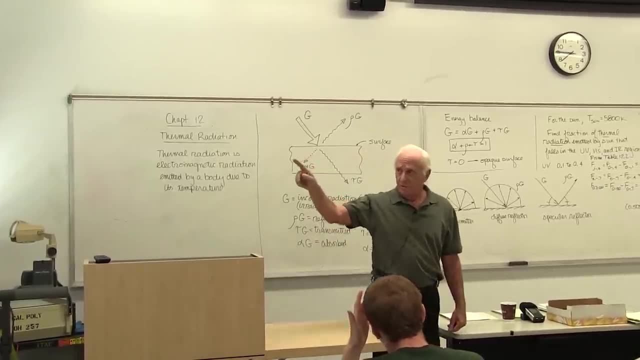 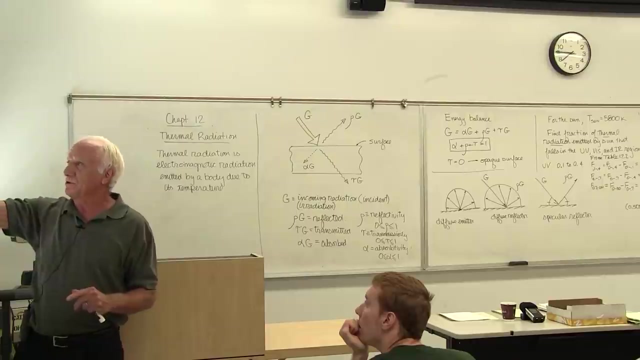 has little bumps on it. And what that glass is, that's a diffused transmitter. A diffused transmitter. Afternoon, you can pull these blinds up. You can pull these blinds up. Afternoon, the sun comes through here near sunset. Those Sycamore trees were probably 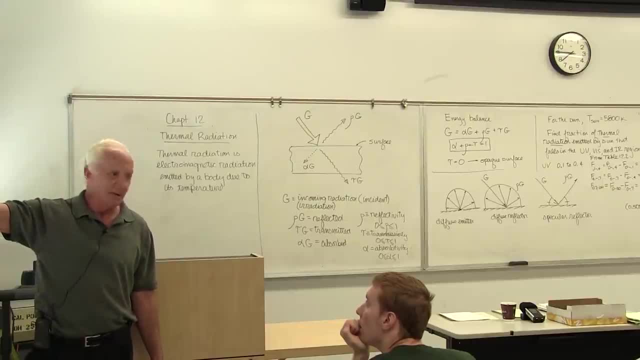 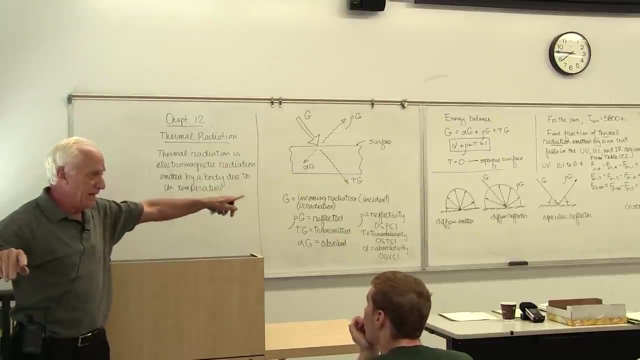 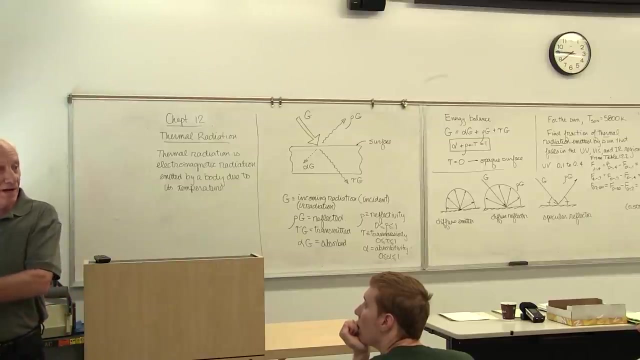 five foot tall in 1964, when this building was built. When that sun would set in the southwest over there, the sun would stream through here and make that board blinding and your eyes blinding. So you, so you put the blinds up and stop right here. Now you've still got. 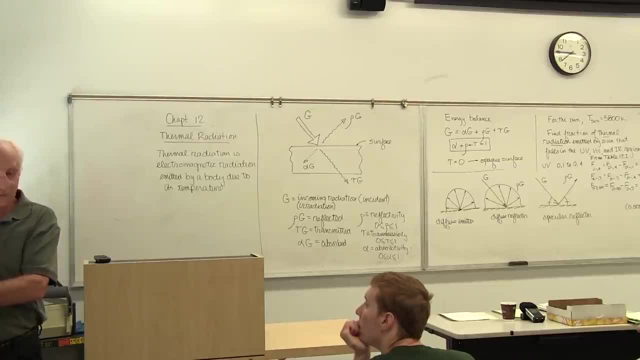 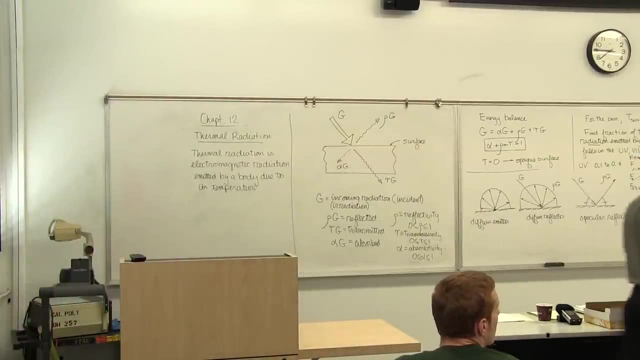 natural light coming through, but you don't have blind spots in this room. This is a diffused surface. Why is that wall painted that rather than a glossy, glossy paint? Why is that nothing glossy? Because when the light strikes it, we don't want it to be mirror-like. I don't want to see my face in that wall. 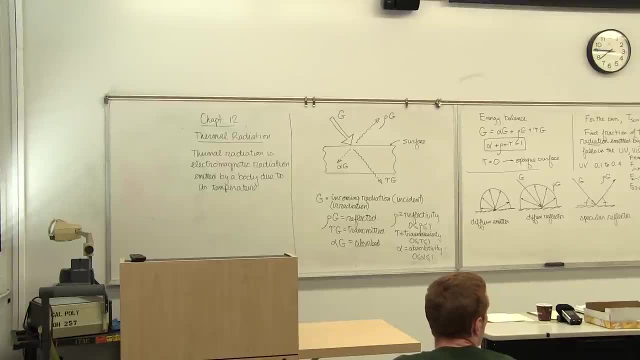 No, That's a diffused paint. Diffused, Call it flat. if you want to go to a paint store, Call it flat paint. Diffused, Gloss paint. I can see almost my face. It makes the shape of my face. Yeah, that's what the word. 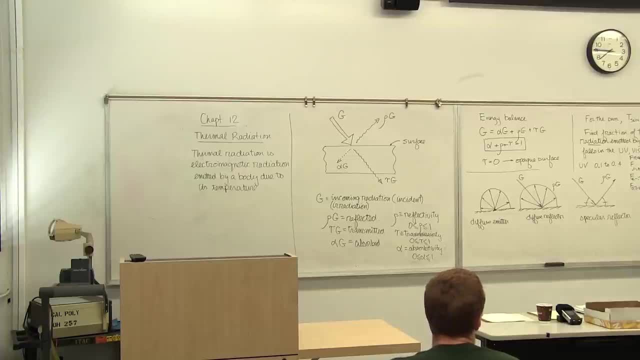 diffused means You've washed your car today. The prediction is for light sprinkles on Thursday. You've got your collar washed, polished. Look at that. Look at that hood man. There's my face, and it sure is pretty. 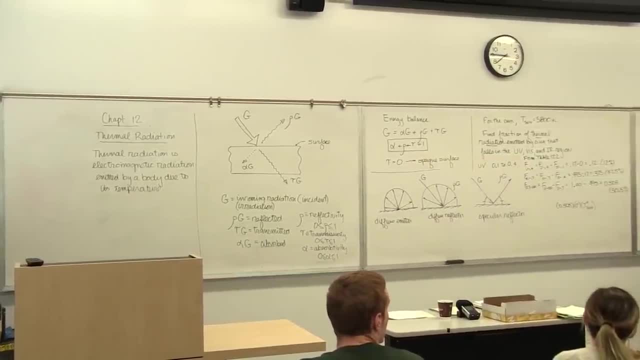 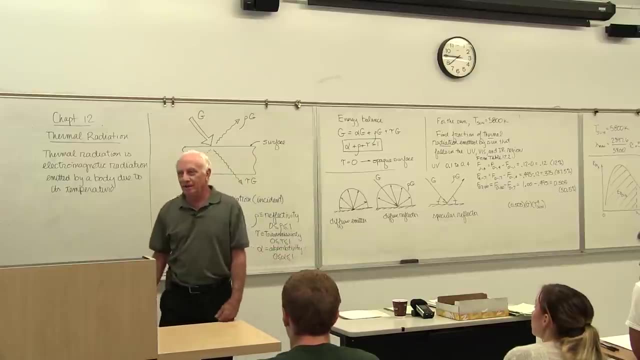 Yeah, What's the idea when you polish your car? You want a specular reflector, You want a mirror-like finish. And along comes Thursday, Here come the sprinkles And you go out and they say, oh my gosh, I'm gone, I can't. 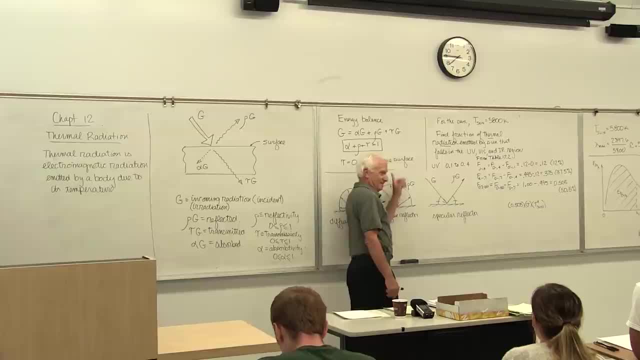 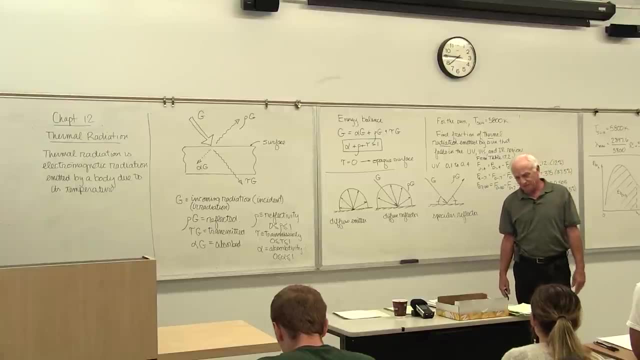 see my face anymore. Guess what it is now. Sun strikes the surface, Boom Spreads the light out. There's no more mirror light. Oh gosh, I've got to wash my car again. That's the example of diffused versus specular. 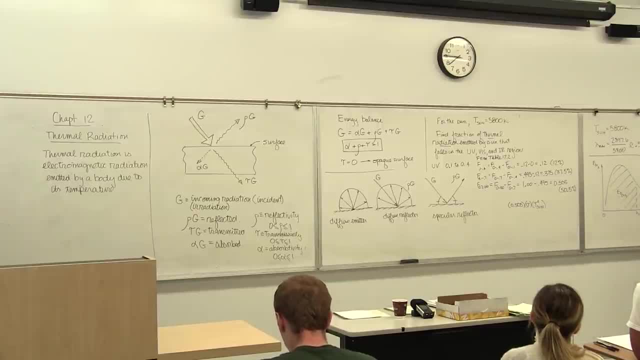 These lights? Why is there that bumpy stuff on that? I just told you over there in the window It's to spread the light out. They're light diffusers. The purpose is of that is that somebody's sitting in that back. 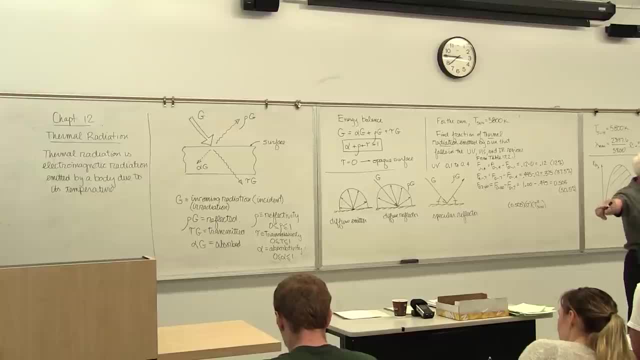 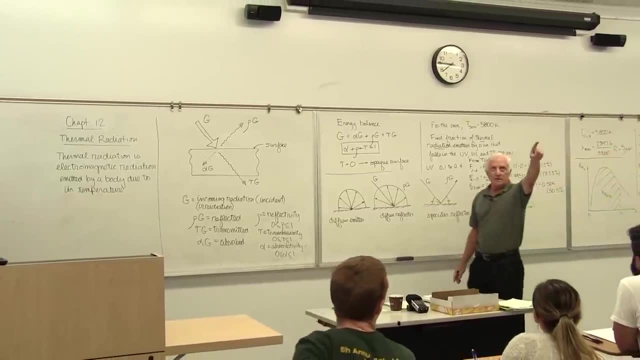 corner over there and over there and the person in the front seat there and there in the middle, all have about the same amount of light on their desktop. Okay, Diffuse surfaces for the lights for us, Otherwise you'd see just tubes. I see tubes, but I see. 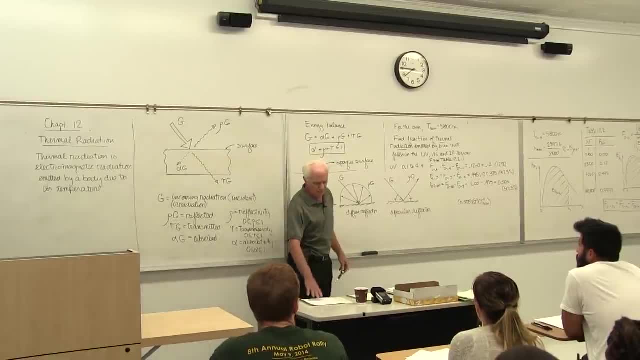 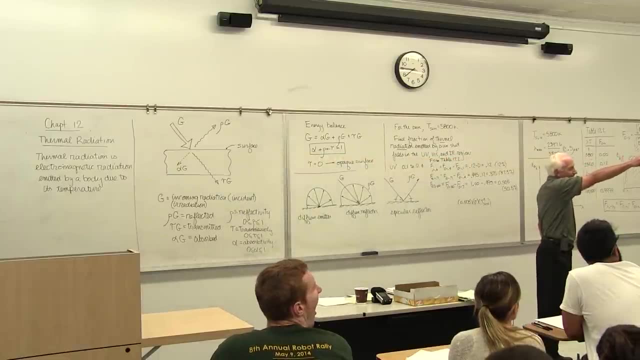 kind of hazy. You've seen my papers up here. All of a sudden they'll blow on the floor. They've done it many times this quarter. That guy over there, he's the problem. He's supposed to be an HVAC diffuser. There's the word again. 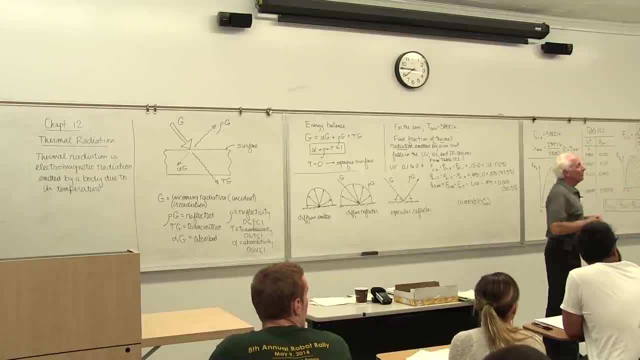 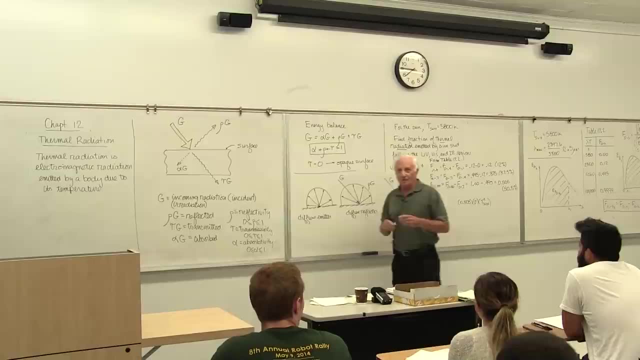 Light diffuser, HVAC diffuser. What's the proof of that guy? Well, he's got a problem, but this is the purpose of that guy. He's supposed to make it so nobody's hair in that corner, in the front, in that corner the front or the middle, nobody's hair goes blowing. and 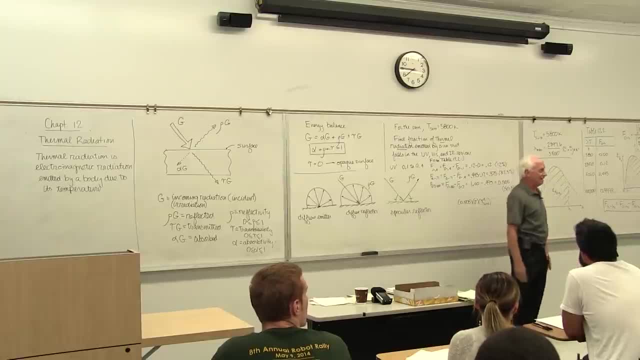 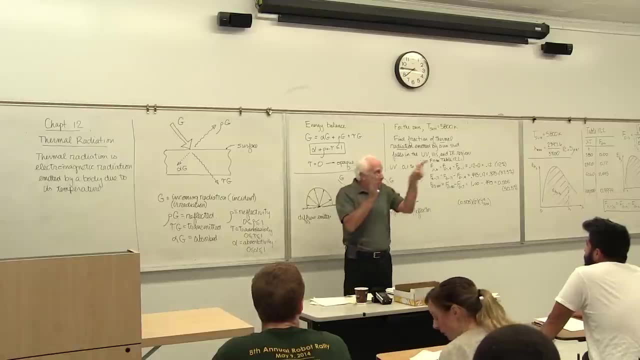 papers. don't blow off my desk up here. He's not doing too good a job right now. But those little veins in there, those little veins, those are diffusers. Their purpose is to spread the volume of air out, so it comes out very gradually and nobody's uncomfortable, Nobody's paper on their. 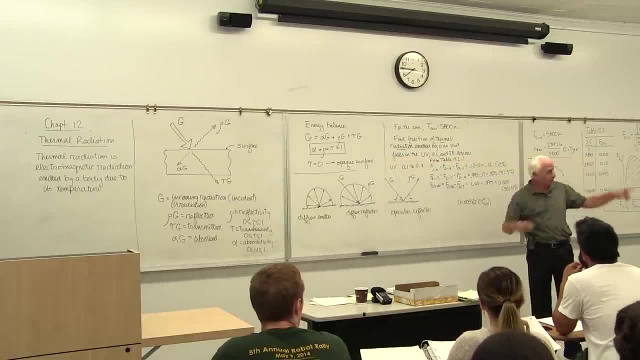 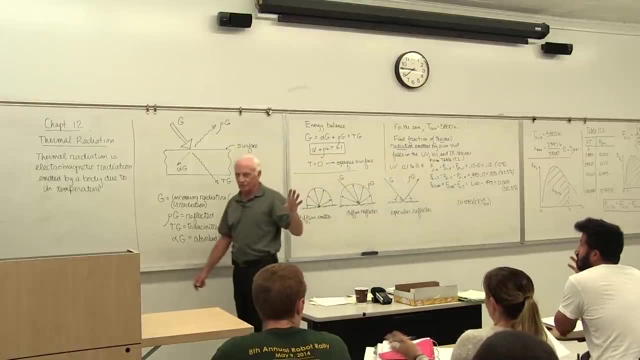 desk is moving around. Your hair's not flying around. No HVAC diffuser, A light diffuser. The window's a solar diffuser. Oh yeah, yeah, Most things in the world are diffusers. The wall's a diffuse paint called flat paint. So yeah, that's what the word.